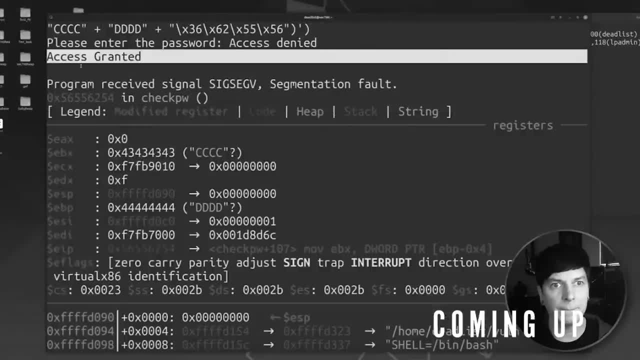 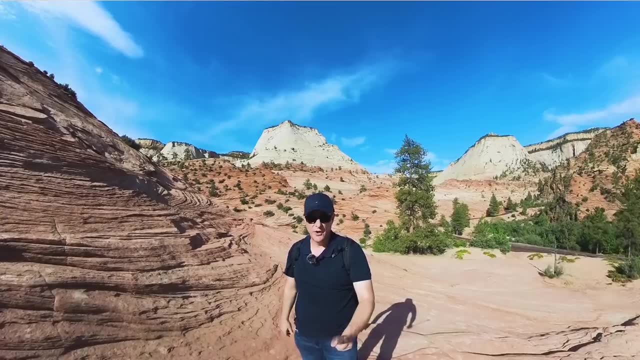 function. you don't return to it. you call it. look at that access granted. so we successfully bypass authentication. now, one of the things i've learned in it is that you can't stop learning. you've got to keep on improving your skills. you've got to keep on improving your skills. you've got to keep on. 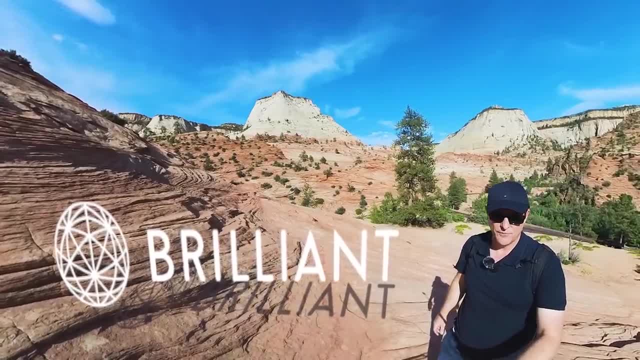 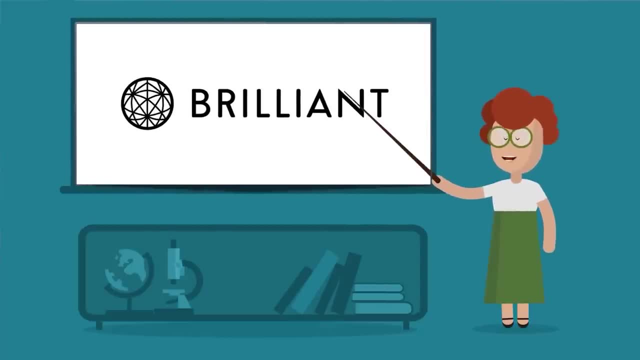 keep on developing your skills and brilliant are a fantastic platform, for that doesn't matter. if you want to learn math, computer science, artificial intelligence, you want to learn programming. they have fantastic content on their website. you're not just going to be reading a book as an example, or 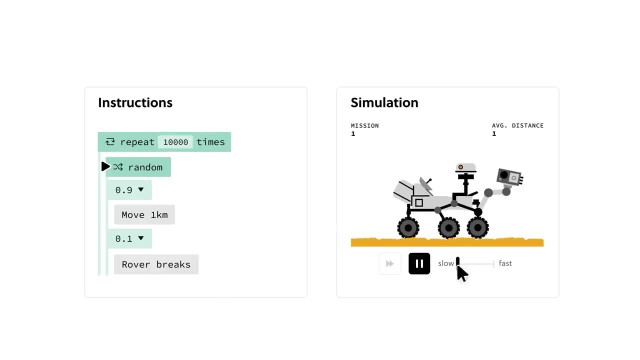 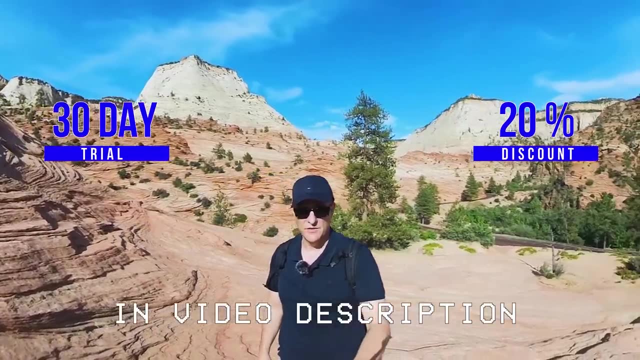 watching videos. it's very interactive and you are involved in your learning. i highly recommend brilliant. use the link below to get a 30-day trial and a 20 discount. so go to brilliantorg, forward slash david bomble. i really want to thank you for watching this video. i hope you enjoyed it and i 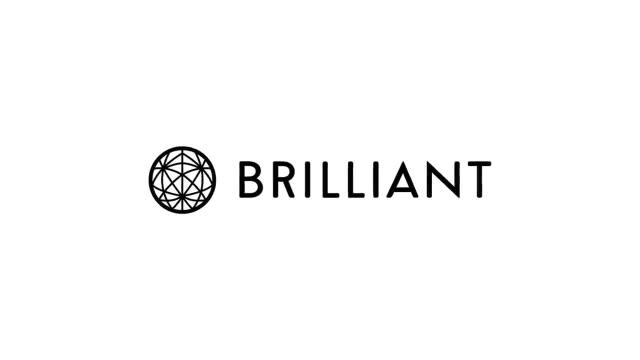 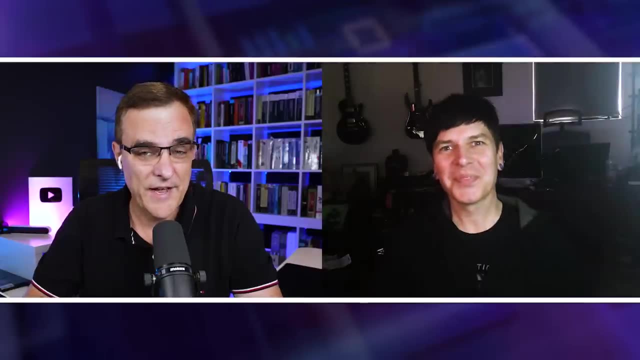 want to thank brilliant for their fantastic partnership and for sponsoring my channel. they really truly are brilliant everyone. it's david bomble back with a very special guest, steven. welcome steven, it's great to have you back. just for everyone who hasn't seen our previous: 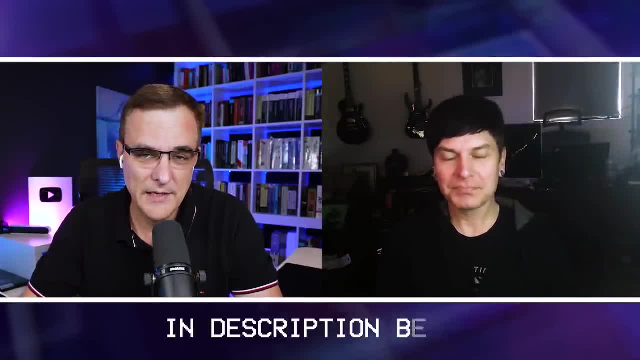 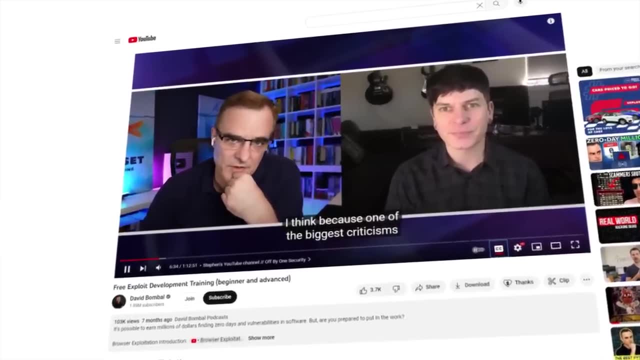 video. have a look at the link below. steven's talking about zero day millions and how you can like earn millions by finding a zero day. it was a fascinating story. lots of cool stories in that video. so have a look at that video if you're interested in learning more about steven. but 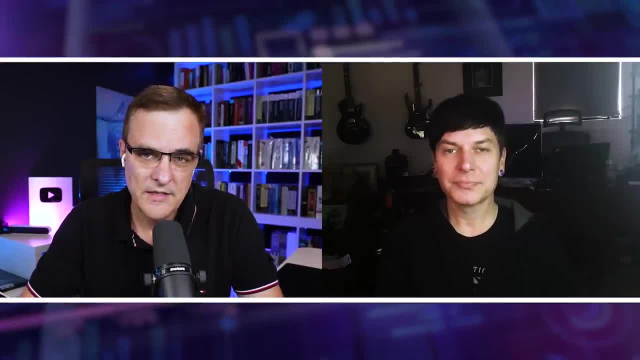 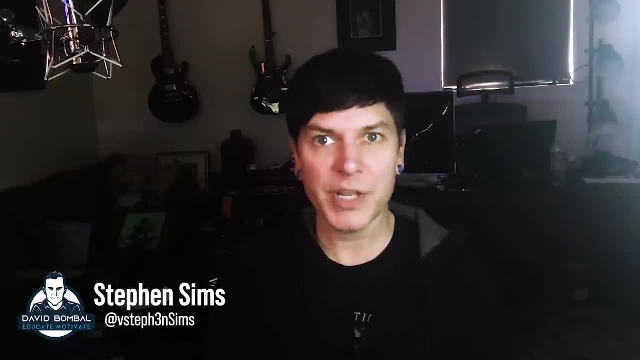 steven. just for people who haven't seen our previous video or don't know who you are, tell us yourself and tell us about your channel. yeah, great, my name, as david mentioned, steven sims. i'm a sands instructor with the sands institute and also the curriculum lead there for the offensive. 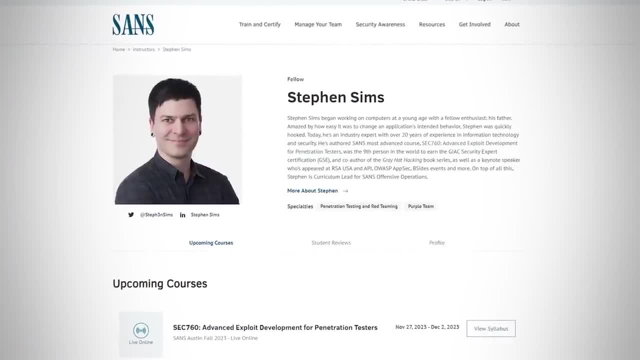 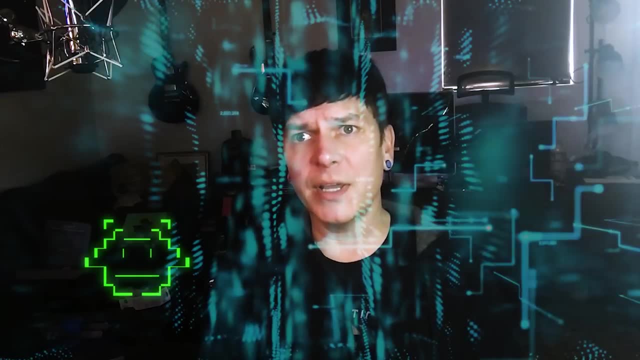 operations curriculum. i'm also a courseware author of a few of their courses on like advanced pen testing, exploit development. i live out in the bay area in california and i've been doing bug hunting and exploit development for probably close to 20 years now. time has flown, but it's a lot of fun. 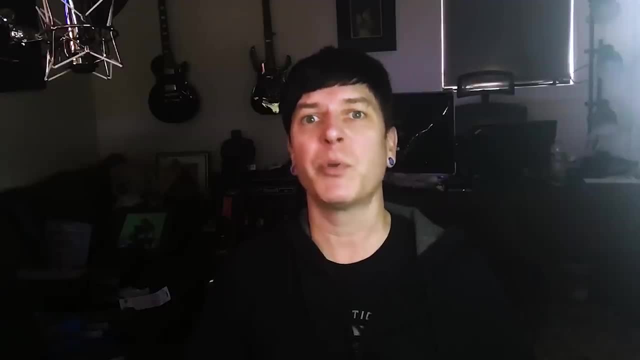 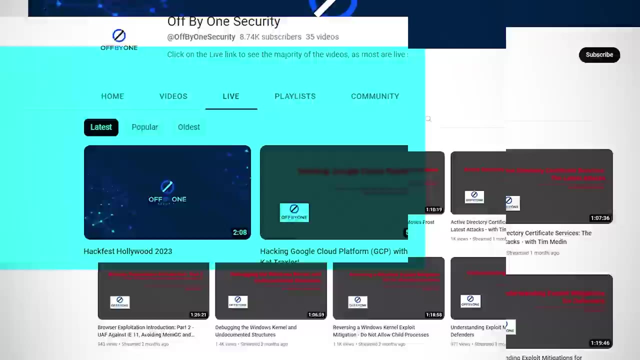 it's something where you never, never, you never lose your interest, you never will know everything. so tell us about your channel, because you've started. you started that not so long ago, right? yeah, so i started it off as like when i retire courseware content from a course through sands, i'm like: well, this is content that. 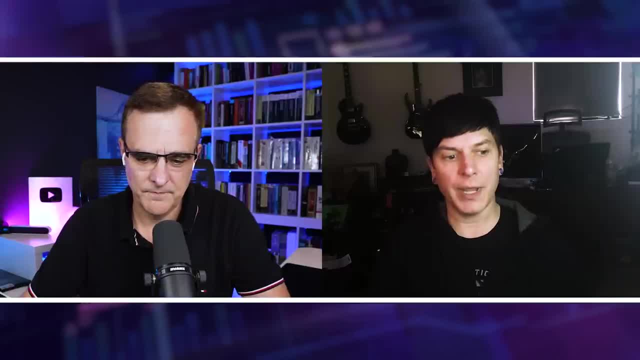 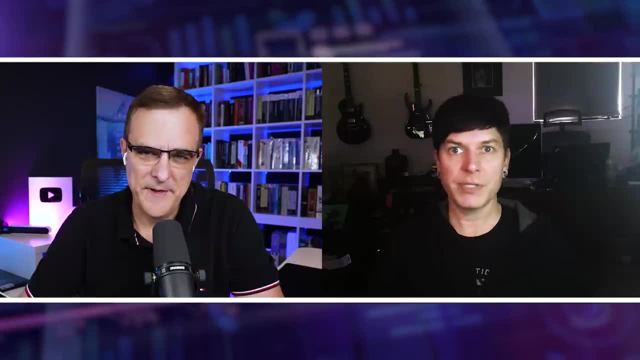 i think people would still enjoy just because we're moving it out. and so i reached out to the community and said, hey, would you all like to see something like browser exploitation against internet explorer 11? and people said, absolutely. so i started doing it that way and then continued: 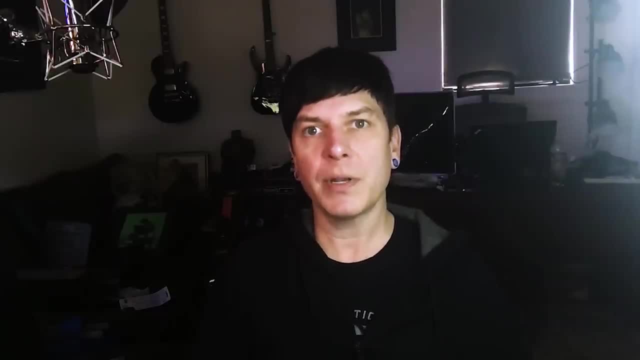 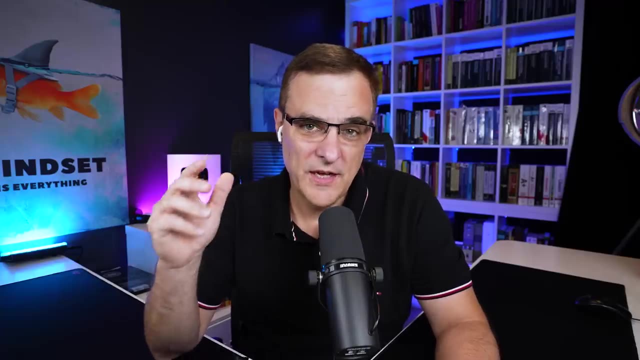 down like the advanced technical area, but it's branched out a bit like. i just had one last last friday on hacking google cloud. yeah, so for everyone who's watching, we're going to cover. well, steven, tell us the topic that we're going to cover. i'll just say: you know, go and look at. 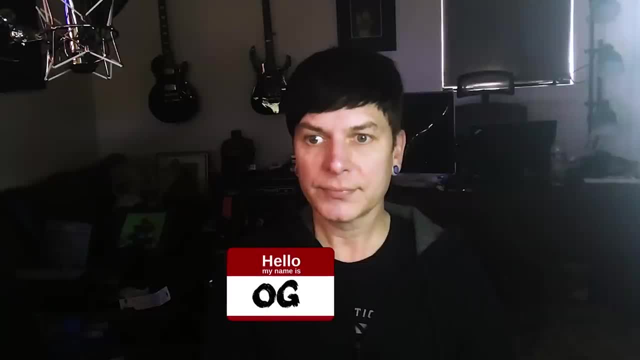 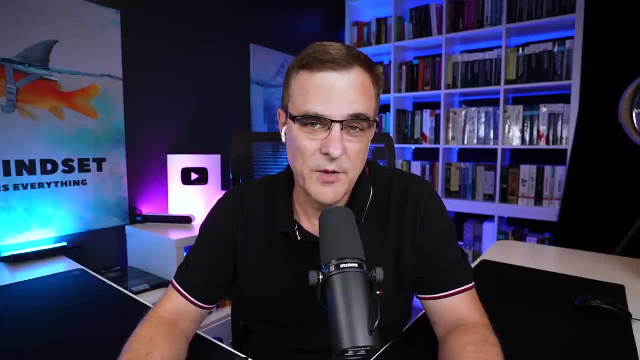 steven's channel for amazing content. steven is one of the ogs in this field. if you really really want to learn, go and have a look at his channel and go and subscribe. go and show the love. but, steven, what are we talking about today? yeah, today we're just going to cover basic buffer overflows. 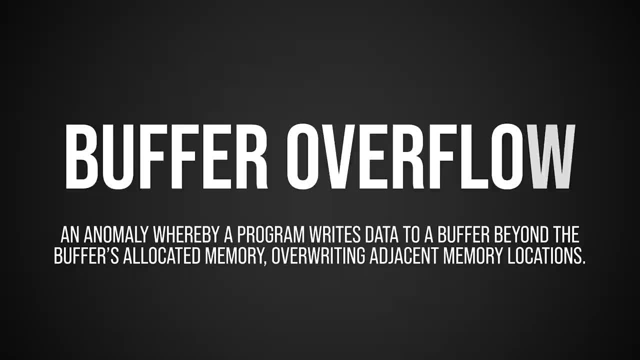 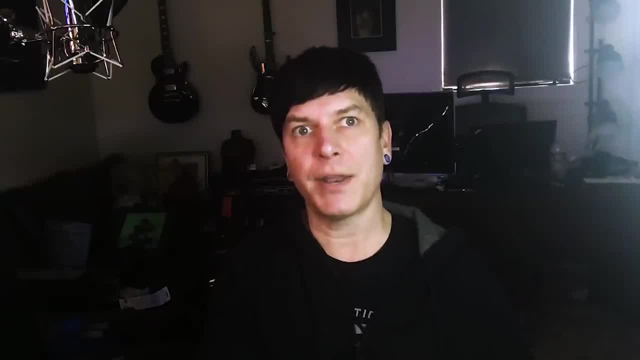 and i think it's important to do that because even if you want to jump in at the beginning of the 2023 or 2024 and get into exploit development, you've got to understand the fundamentals, even if a lot of those types of attacks are mitigated in many cases. you're telling me offline that 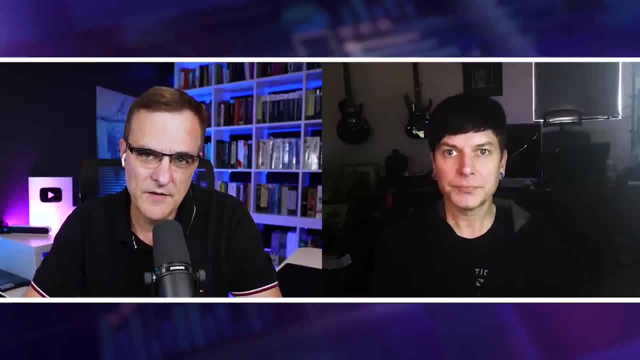 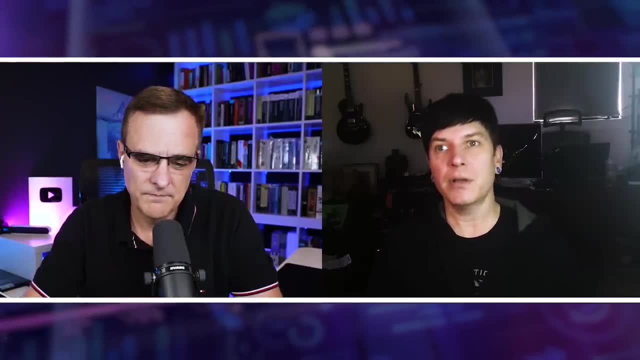 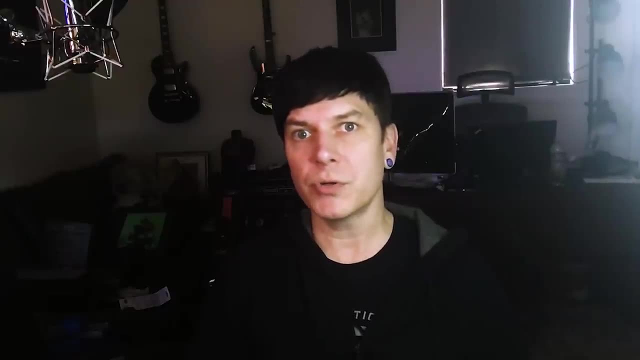 buffer overflows have been around forever. it's surprising that they're not dead now, but there's some news coming right. yeah, so i i will always say that the golden years of exploitation was back in the 90s up into the mid 2000s, because there were no mitigations or security controls that were there. 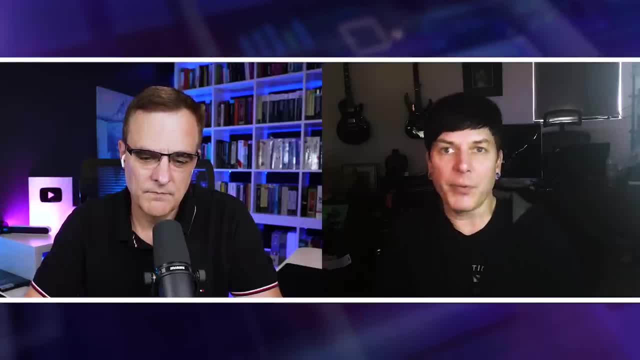 preventing for exploitation to be possible. so, even if the vulnerability is still there, there are these mitigations that try and stop the actual exploitation for being successful, or even your shellcode execution. so i remember people saying all the way back in the 90s, like the day of buffer. 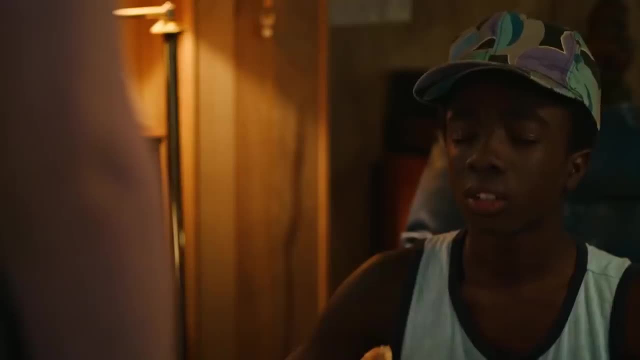 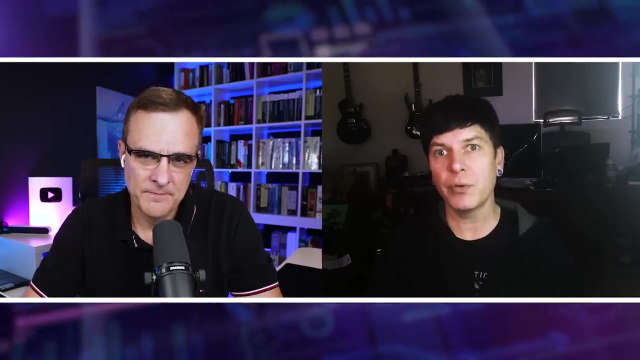 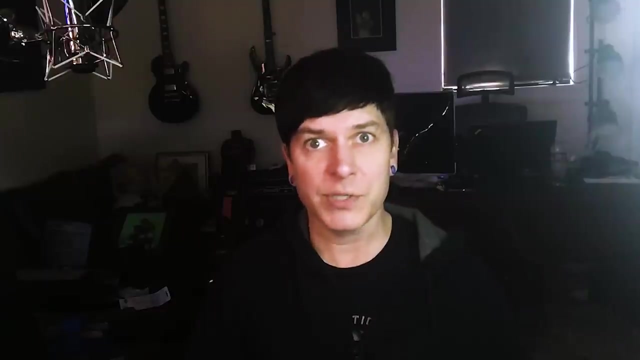 overflow exploitation is coming to an end any day now, and here we are- 2023- it's still possible. but yes, as you mentioned, there are some newer mitigations called control flow enforcement technology, or cet, as well as a shadow stacks and other mitigations that are even- i will say like they are- the end of buffer overflows, the 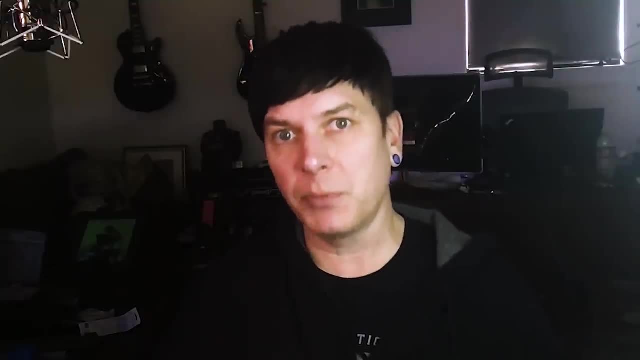 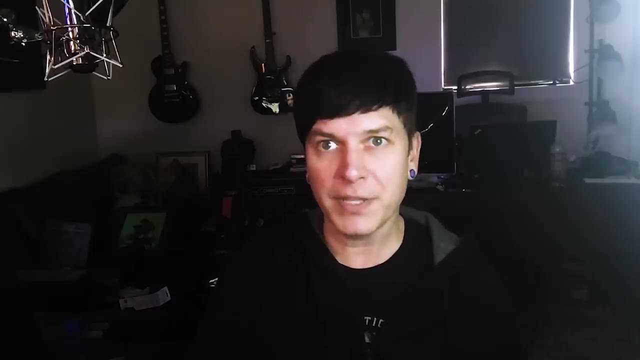 vulnerability is still there in the code, but the ability to actually exploit the vulnerability is pretty much will be mitigated completely once these roll out, and if you're on the side of the fence where you don't want to see this stuff go away, it's still going to be some time, because the actual hardware. the processors themselves have to support the mitigations, so they're not just going to flip. they, being microsoft or other vendors, are not just going to flip the switch and make it, so they break all your apps. so it's going to be a while. so you mentioned microsoft, is that? 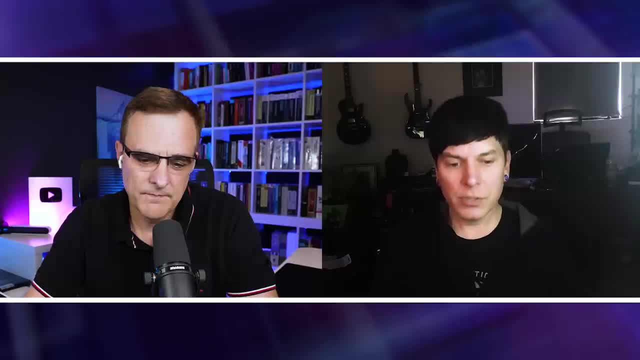 is that something that's built into windows, or do you have to do something to enable it? yeah, so on windows. it's part of something called exploit guard, which used to be called the enhanced mitigation experience toolkit or enet. exploit guard came out on windows 10 at some point. it's. still there on windows 11 and it's a, i would say, mitigation toolkit where the majority of the mitigations- and there are over 20- are turned off by default- almost all of them- because they're going to be turned off, because microsoft doesn't want to turn everything on and potentially break. 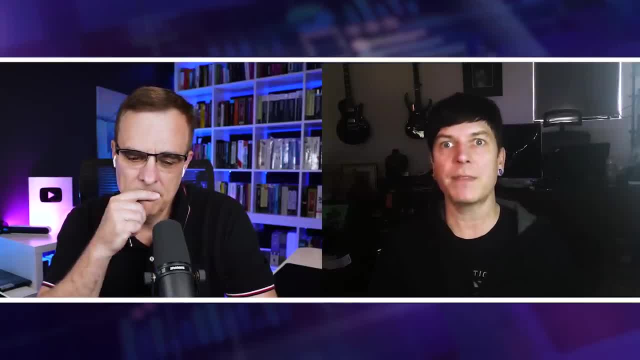 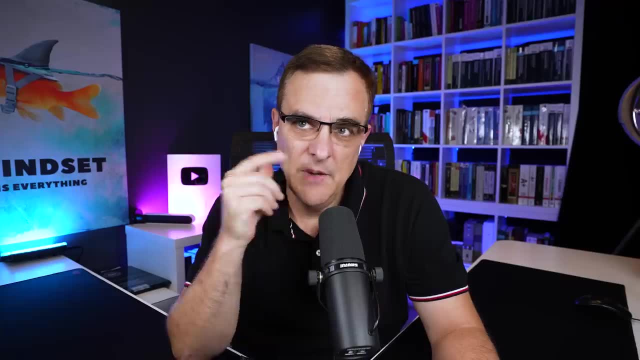 your application. so it's up to an administrator to understand the effect that the mitigations will have both on application performance, as well as breaking the app, depending on how it's coded and that's available in linux and mac os as well, or is it just a microsoft thing? yeah, most operating. 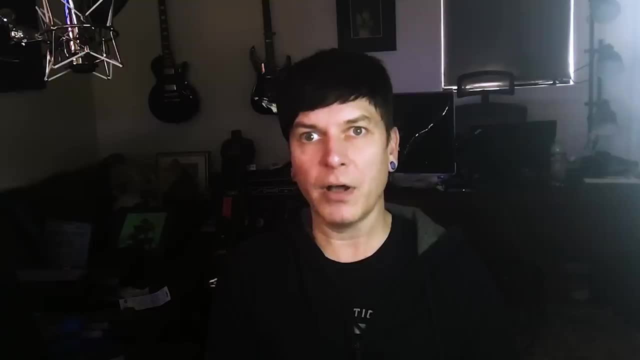 system vendors, all the big ones, have ways to turn this stuff on or off, but each are different in their own way. and is it what? what's holding it back? is it the hardware? was the applications? or yep, well, for shadows, stacks and stuff, specifically, that's held back by the actual hardware, the processor architecture. 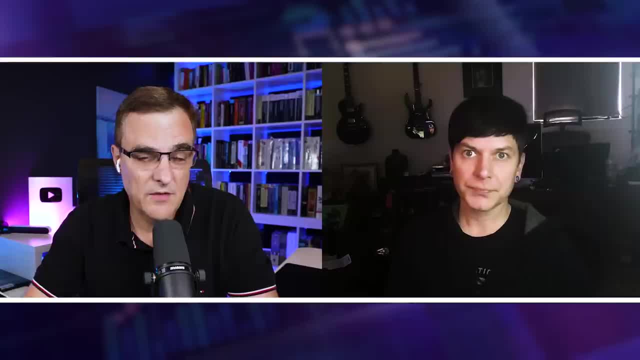 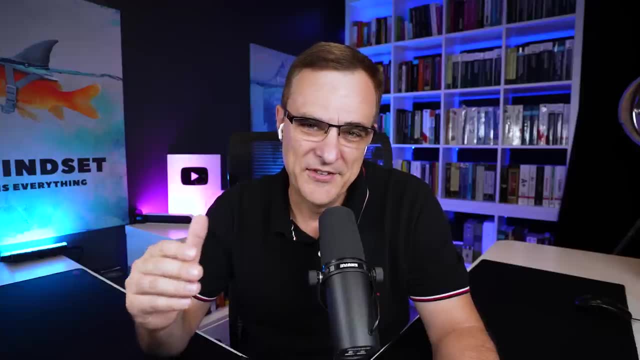 that's great. so, just for everyone who wants to learn- i mean, steven, it's important to learn this, like you said, it's it's it's a basic building block, right, that you need to know. so, even though this i'd read to say maybe stop soon, um, it's something that you need to learn, right? yeah, and 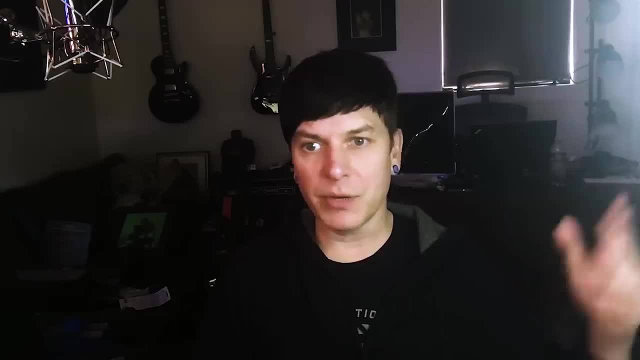 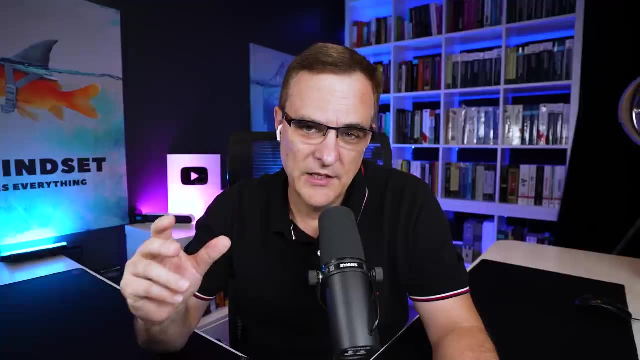 just because microsoft might be implementing it doesn't mean that the iot world and all these other things out there are hard for it. so i mean i want to keep quiet now and let you take us on this road, so perhaps you can just start like a gentle introduction and then go hardcore into it. what is a buffer overflow? why is it important? 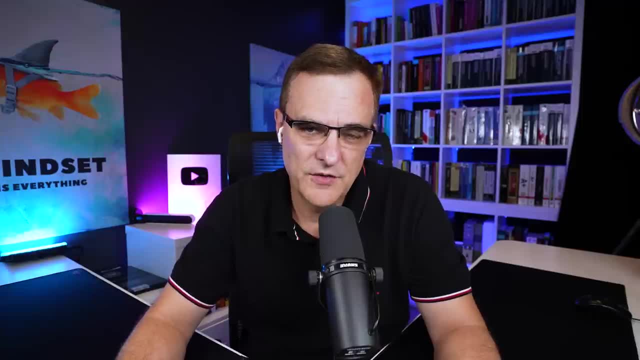 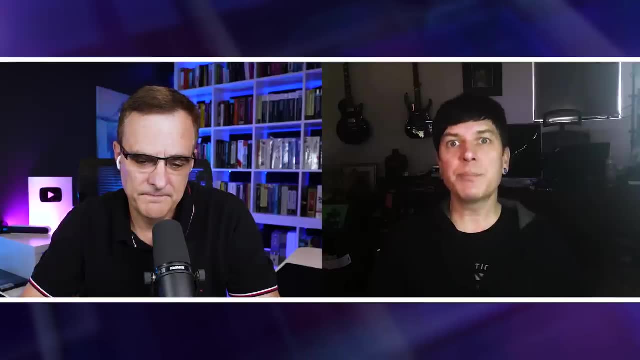 and i don't you know. i just want to let you take us down this road. i know you said you've got some slides and stuff that you can share, so you take it away, steven, yeah, great thanks, and feel free to chime in and ask away. um, so yeah, i did put some slides together, a few. i want to show you two types. 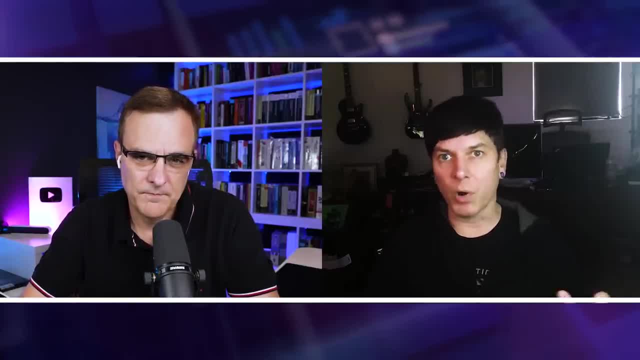 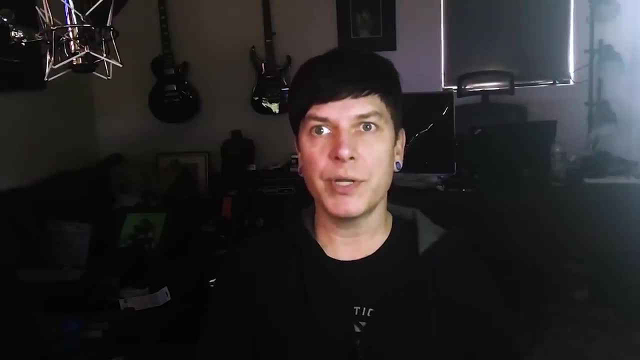 of buffer overflows, the. the first one's going to be the most basic, ordinary one that you would see in any college. you know that you attend and go to some security classes, see, but the other one i will show you, that's the one that's just going to be a screenshot of some disassembly of, uh, this one. 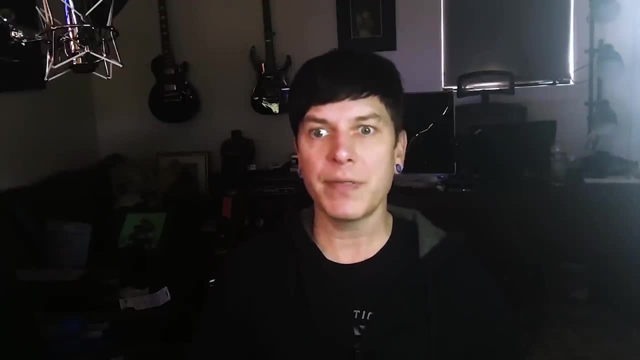 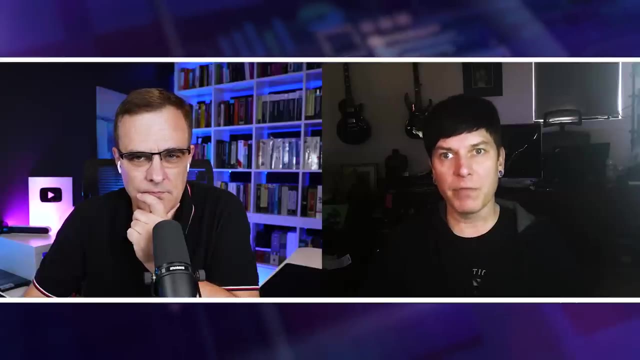 i'll show, just because it's easy to digest, is from the sig red vulnerability that came out a couple years ago. that affected dns, and that type of overflow is a heap overflow. so they're both buffer overflows, but one's on the stack and one's on the heap. and the second one i'll show you will. 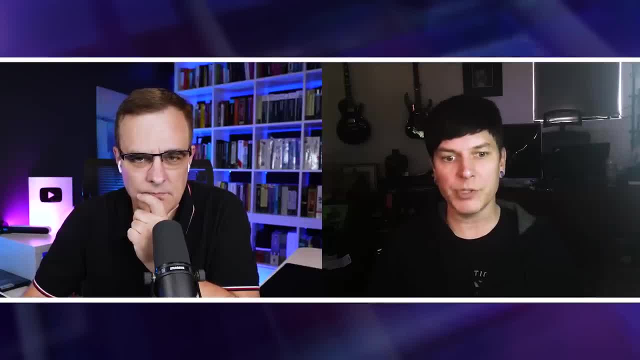 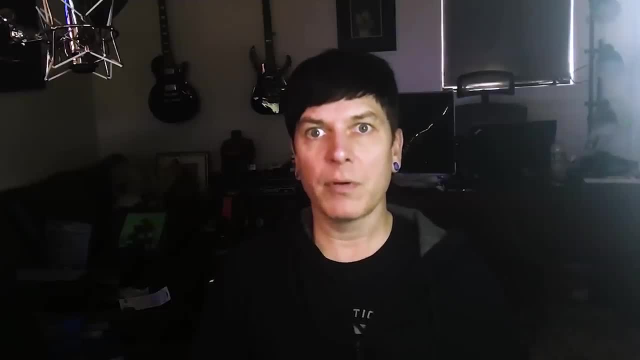 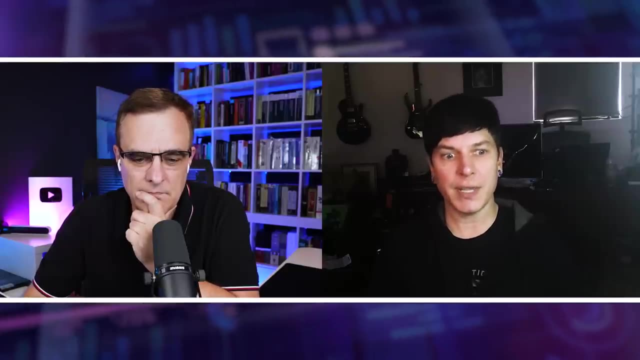 be more real world. and then i also plan on- we'll see how it goes- the plan on jumping over into command live and we can try and take a look to see if we can see this in a debugger. but a buffer is when you're dealing with a function that is being called, if that function needs to say copy. 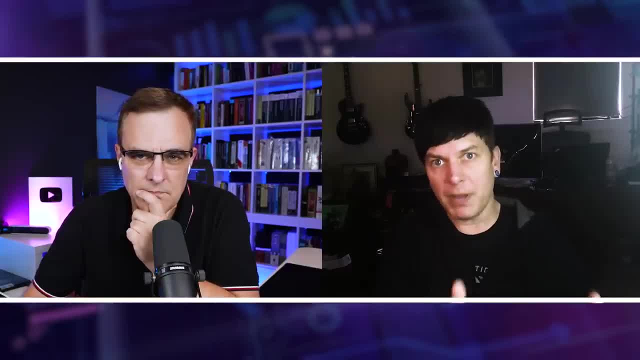 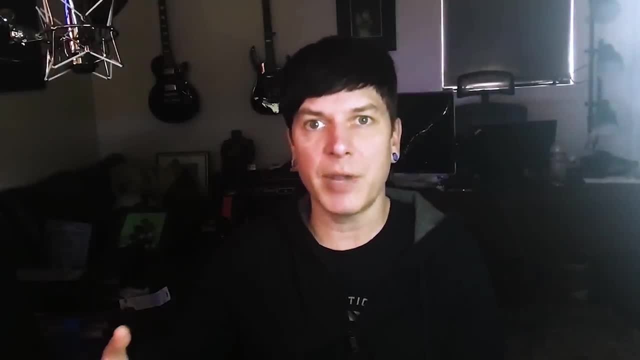 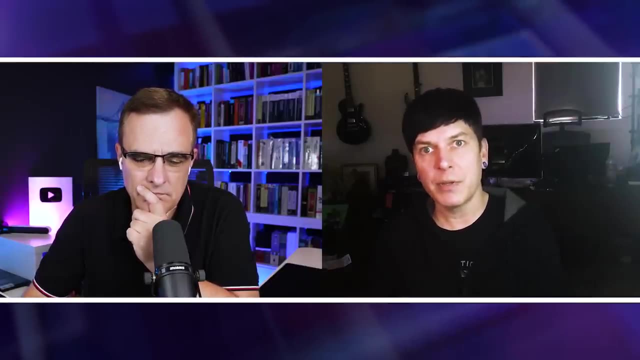 a string, meaning a number of characters, into this buffer and interact within the program. at that point you have to allocate the appropriate amount of space to store this information. so, to take a step back, each function call that gets made gets its own stack frame, so the stack is its own region. 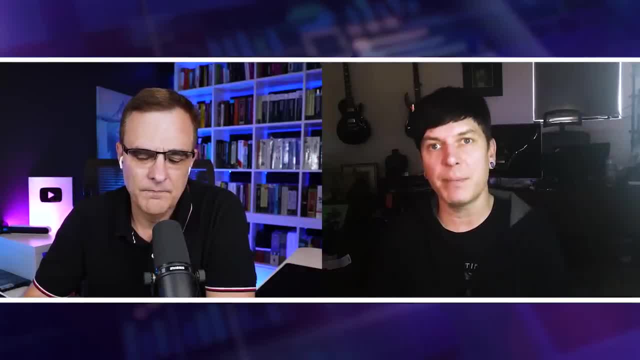 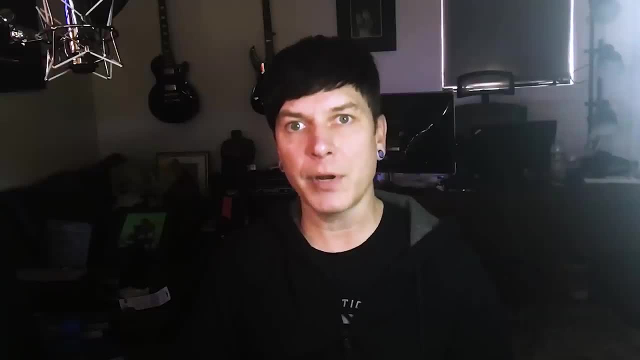 of memory and again, every function call gets a stack frame. so the stack is its own region of memory and some functions will need a buffer and other ones don't need a buffer, so the ones that need a buffer you need to allocate memory on the stack and it's a finite lifetime because it's only going. 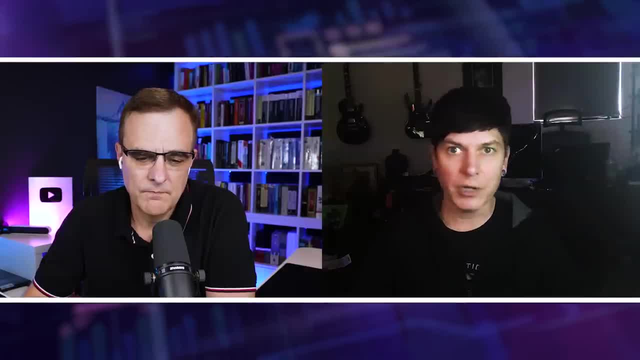 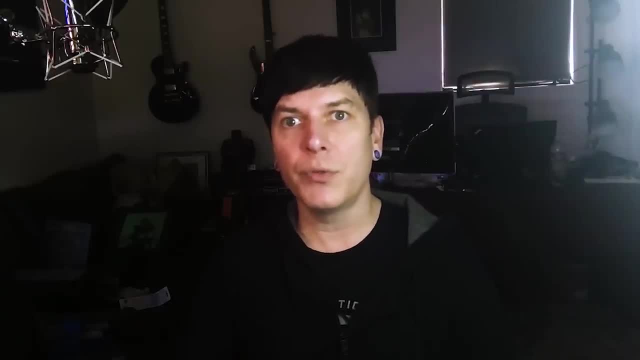 to be there during the function call itself. once the function returns out, then that stack frame gets torn down. it's no longer needed. so if that function needs a buffer, then you'll then have a memory copy operation. it could be one of many functions that actually copies the data from a. 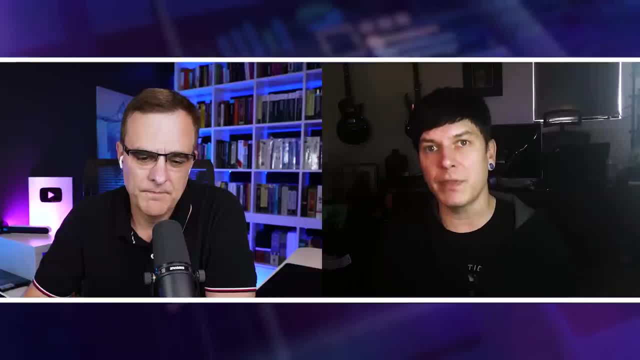 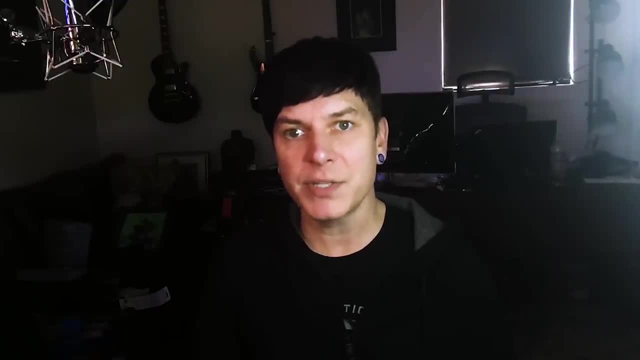 source into the destination frame. so if that function needs a buffer, then you'll then have a destination buffer that in this case would be on the stack. so the problem comes in if there are no balance checks or if we're not checking the size, the number of bytes that are going to be copied. 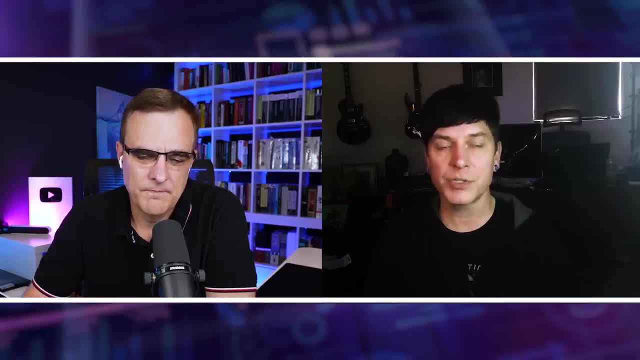 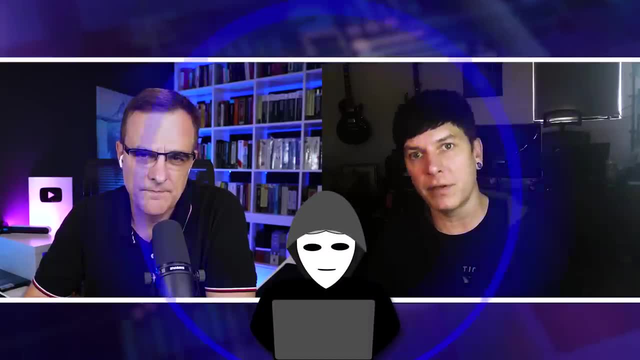 into the buffer, then it is possible for an attacker or just a regular user to inadvertently send more data into the buffer than is available, which means that overflow of information has to go somewhere. so what is it overriding? you know, there's the saying. i think einstein said it. 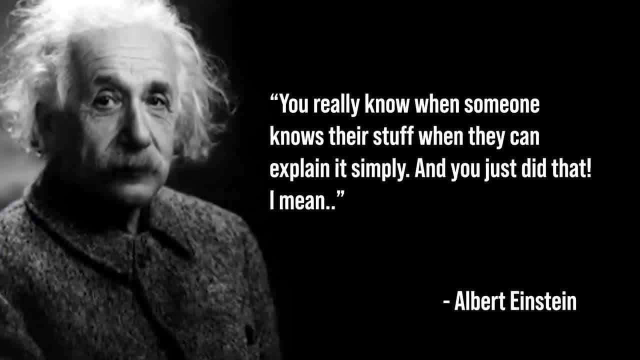 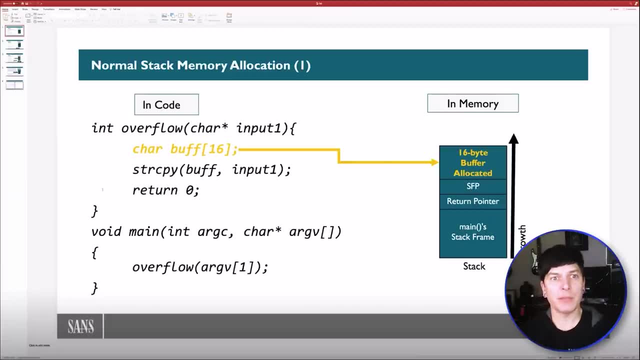 you really know when someone knows this stuff, when they can explain it simply, and you just did that. i mean, i've been doing a lot of research on this and it's like you just explained it so nicely so on this slide. it's going to be a very basic c program that has 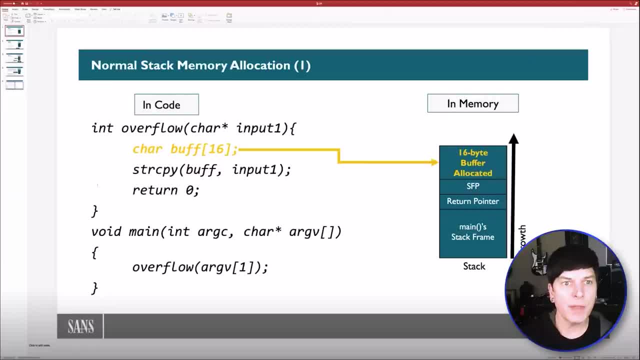 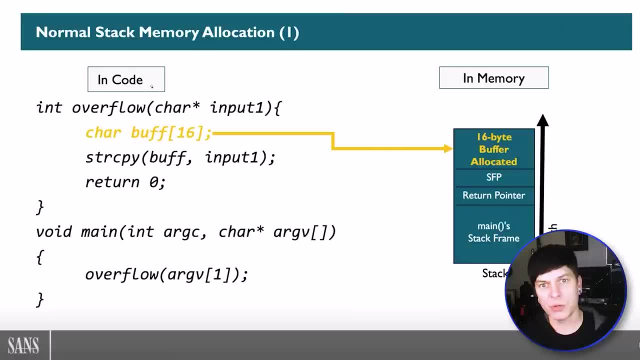 a buffer overflow vulnerability intentionally written into it. so on the left side where it says in code, that would be the code segment. this is where the executable code is stored in memory while the program is running, while the process is up and running, and then over on the right. 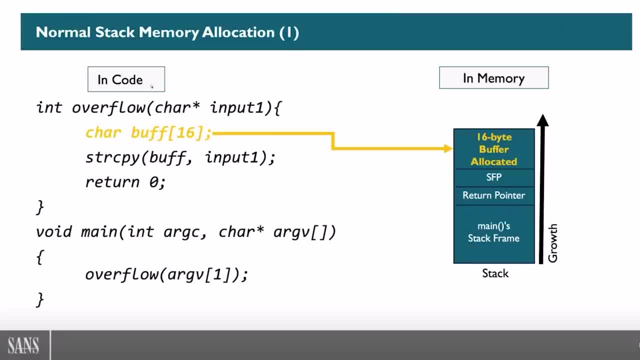 you see, on the bottom right it says stack. that would be a different location in memory that specifically be there to store stack frames associated with the various function calls. so in the code on the left you see that we're creating a buffer, we're calling it buffer, it's. 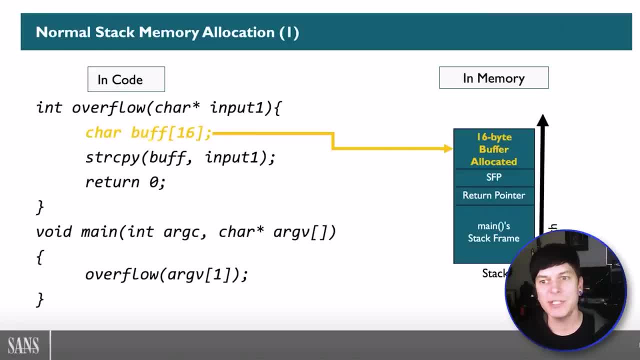 a character buffer and we're setting it for 16 bytes, so 16 total bytes of memory have been allocated on this stack frame associated with this function called overflow. so if we continue forward, we then have a function called stir copy, which is a banned function, and by that i mean it's 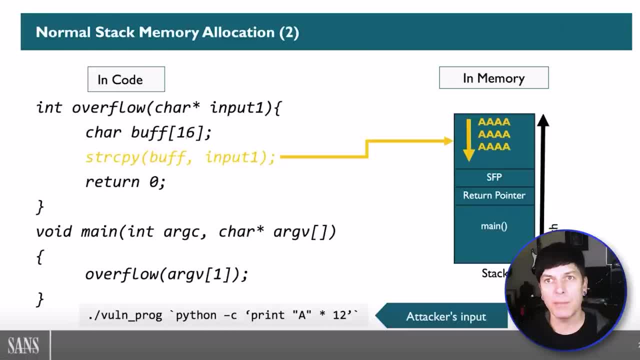 antiquated. it's unsafe, it should never be used anymore. but we're going to be able to store. but it's still out there in legacy code you will come across it. so it still has to be supported. but you see where it says stir copy buffer. so that is the destination first, which is that 16. 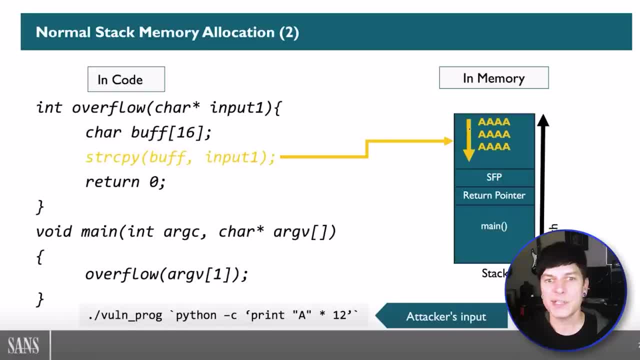 byte buffer that'll be allocated over on the right. and then it says input one is the source. so input one is going to be coming in from what we will call the argument vector one. so you might have heard of argv and argc. that's the argument vector and calder argv0 is always the program name. 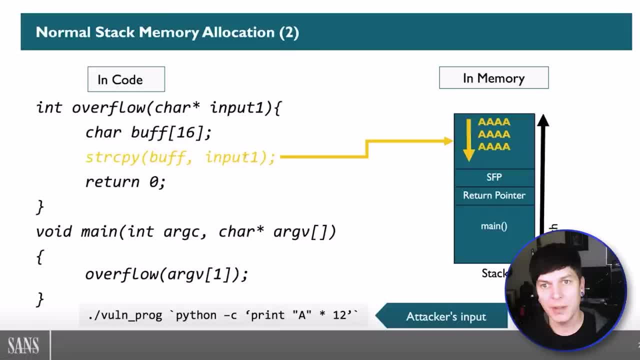 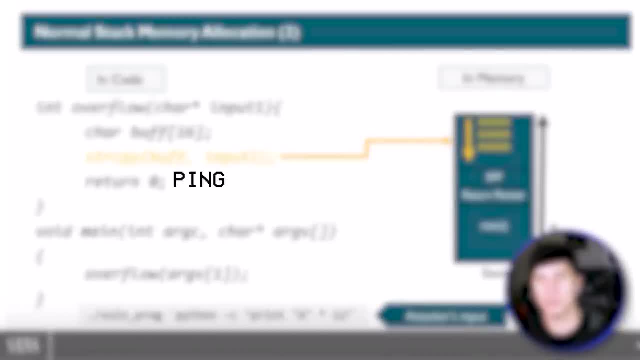 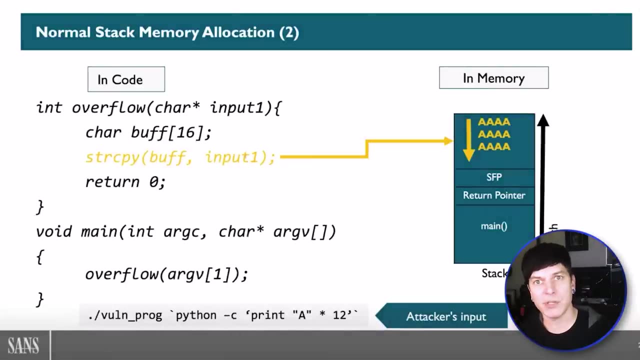 one would be the first argument that you pass in via command line and then, if you have another argument, it's expecting argv2. think about an example like ping. if you say ping space 127.0.0.1, ping is the program name, that would be argv0 and then your ip address that you use the loopback in. 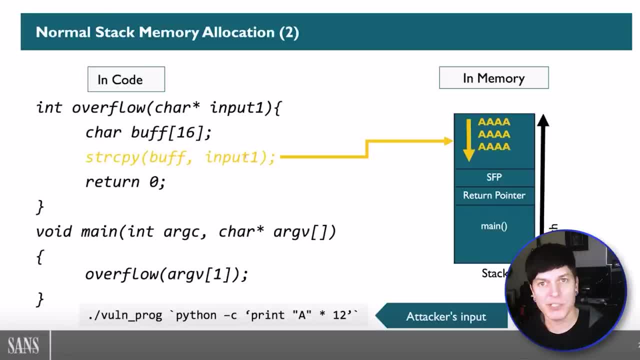 that case, 127.0.0.1 is the address that we're pinging. that would be the argument one. so in this case, whatever the user types in as a command line argument is being taken and written via stir copy into that buffer that we allocated with 16 bytes. and if you look at the 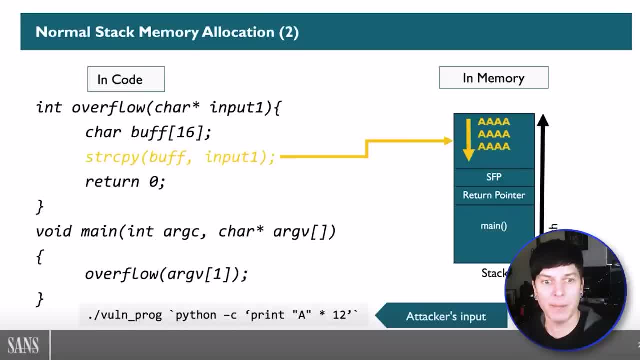 very bottom you can see we run this program called vuln program and we're using python to just send in 12 a's and you can see that those 12 a's are being written to memory into that buffer. it's being written from the top downward and that's what that arrow means pointing down. so we've 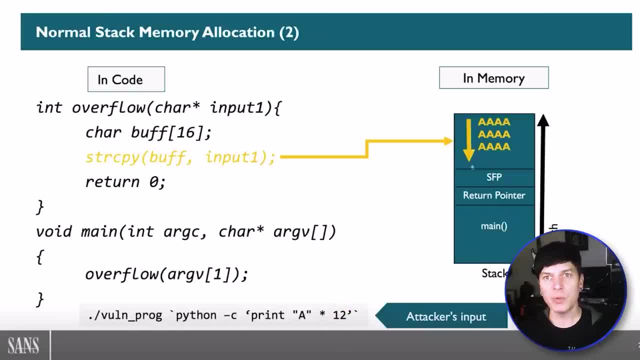 only written 12 bytes in this case, so we're not hurting anything. so you wouldn't realize that there's a vulnerability yet in this program, because the process is not going to crash if we do this again now. you can see on the bottom. we do a times 32, so we're writing 32 a's into a. 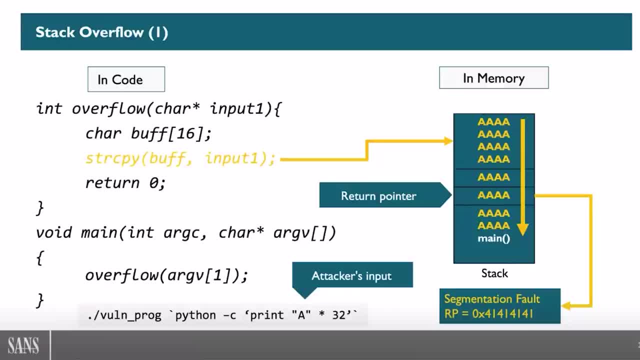 16 byte buffer. you can see over on the right. we've overwritten everything else that was there, notably the return pointer. so the return pointer is how the function that we've called, in this case it's called the overflow function. it needs to know where to return control after it's done. 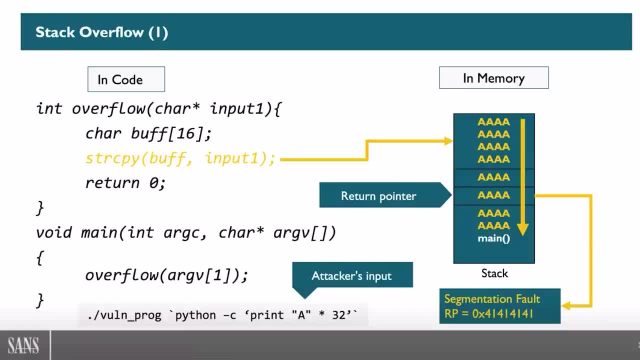 doing what it's supposed to do. so we do that by returning to the return pointer. there is a special instruction called call. so if we're running this program in the main function- so we just started up the program- and you hit this instruction that says call, overflow the call. 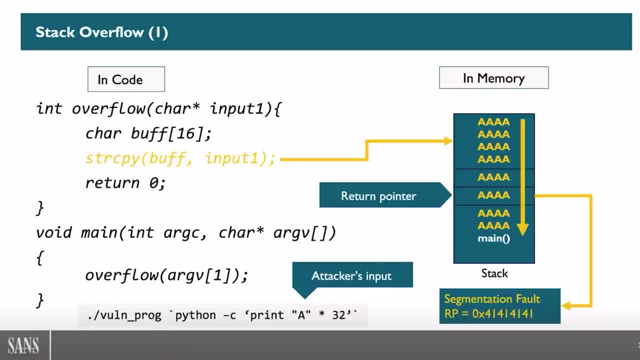 instruction takes the very next address where execution would have continued. it pushes it onto memory so that once the function we've called finishes, it knows where to return control. in this case, we've overwritten it with these a's, so the process would crash and we get this segmentation. 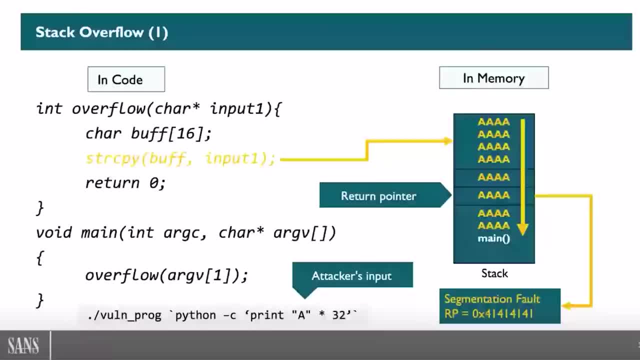 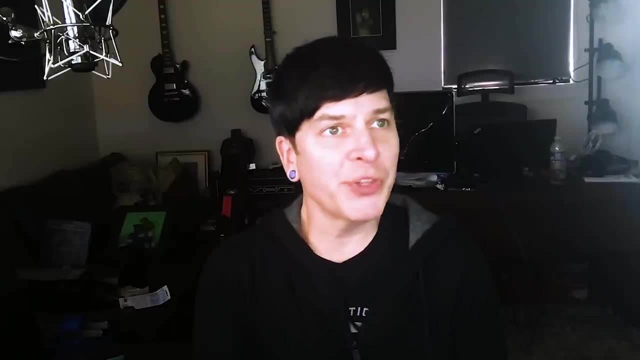 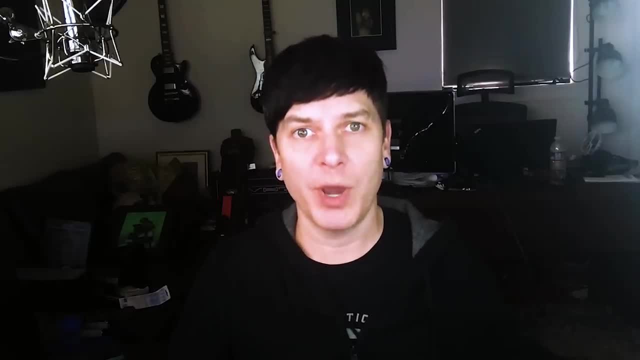 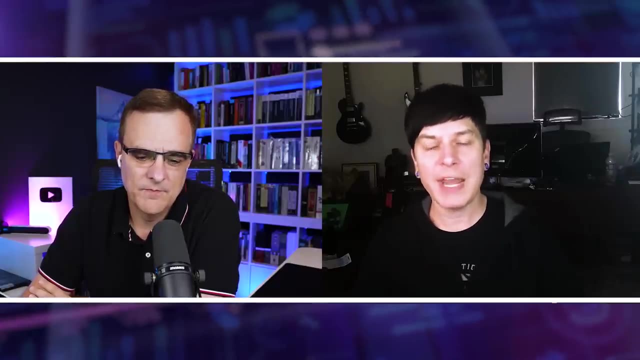 takes on that. uh, what is that? hey, it's just the first letter of the alphabet, and why not, after all, why not? another big part of that is if you see your four one, four, one, four ones showing up anywhere or memory, you know that that's your data that you sent in, so it's kind of like a little signature. 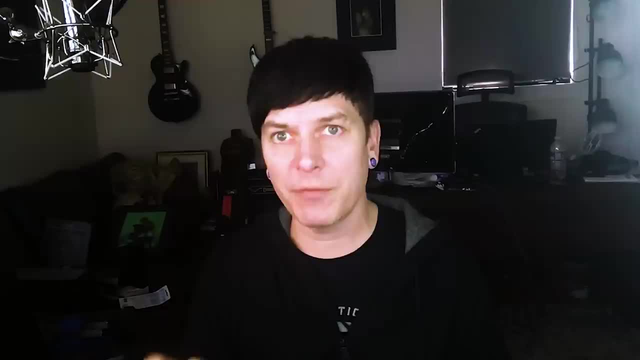 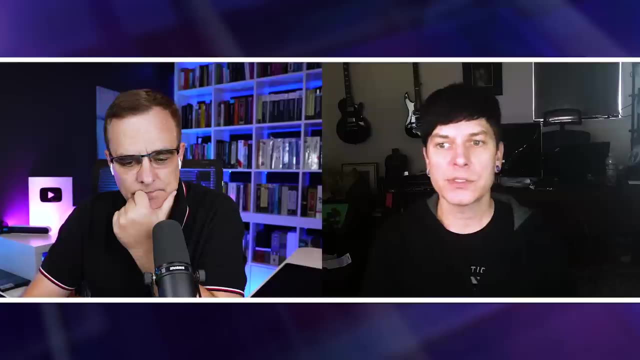 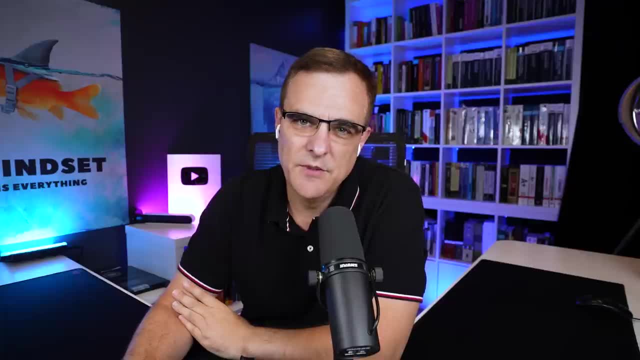 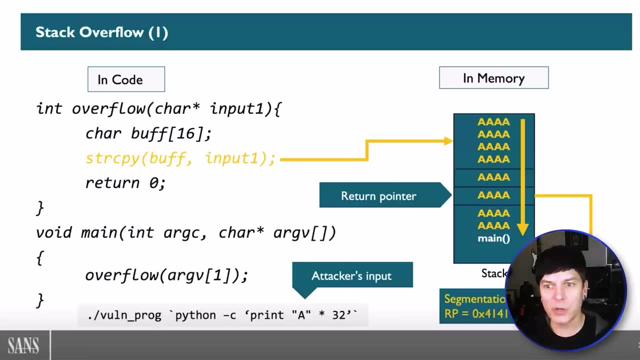 it's not mapped and it will just cause an instant crash. yeah, I've seen all the examples. it's a, so it's great to get a like a real explanation of that, other than people just doing it for whatever arbitrary reason. so thanks, no worries, so that's. 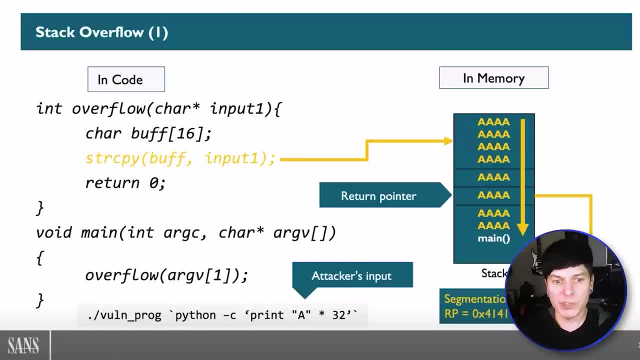 that's in its basic form. again, if we start over real quick and just summarize, we start this program called Vaughn program. it wants an argument, so we just send us some A's. the main function is the very first function to execute once the process is created. you can see here that the 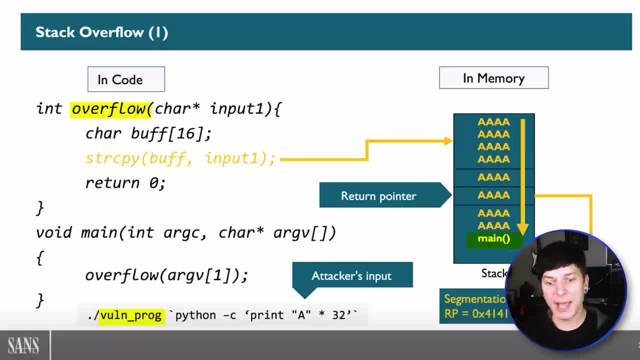 main function calls a function called overflow. the overflow function allocates a 16-byte buffer on the stack. then string copy copies whatever command line argument you sent in into that destination buffer on the stack. well, since stir copy does not include a size argument limiting the number of bytes that are permitted to be written to the destination we can send in. 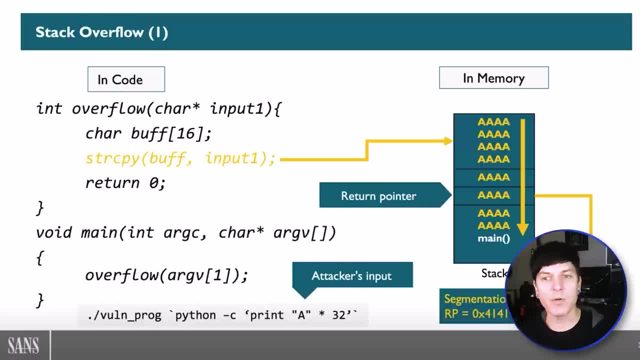 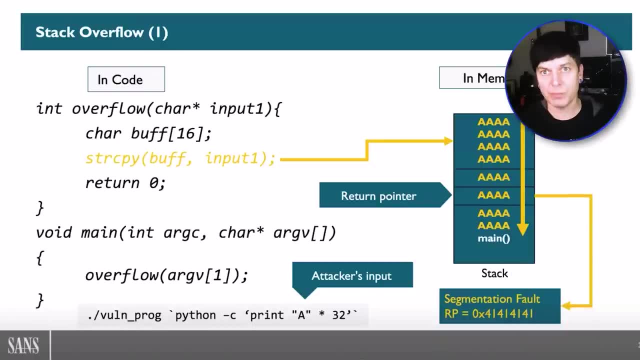 as many as we want. and when we overrun that buffer, we're overwriting, in this case, something called the return pointer, which should be how this function knows where to send the process, the instruction pointer, once it's done, to continue execution, like it should be. but we've overwritten. 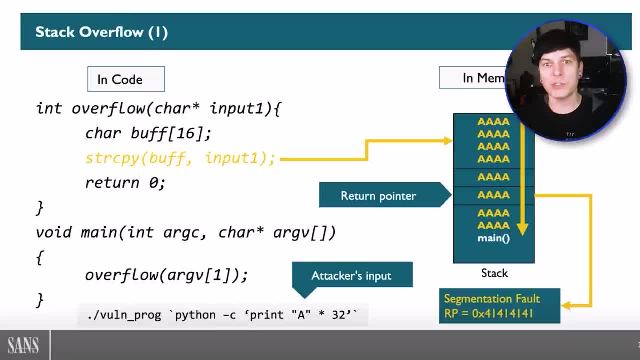 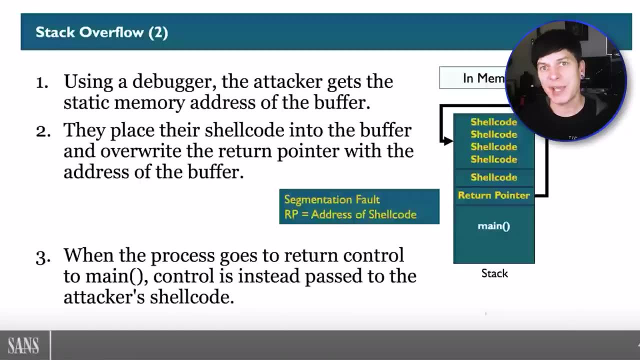 it with a, a, a, causing it to crash. what the attacker wants to do, we would do it with the debugger and we want to start understanding. if a mitigation such as address space layout randomization is not on which it typically is, then we can statically set the. 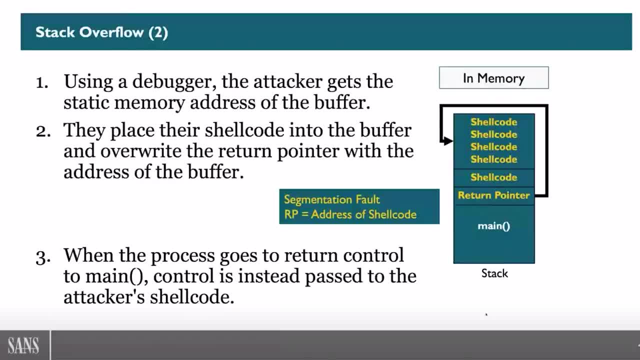 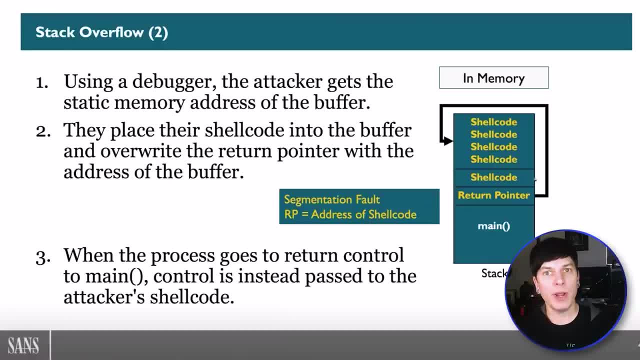 with an address in virtual memory where we can send our data so that buffer that was allocated. if we can get the address of that, then we can put our shell code, which is our payload we want to have executed, like maybe you've heard of meterpreter, or just command exec shellcode or add a user, there's all. 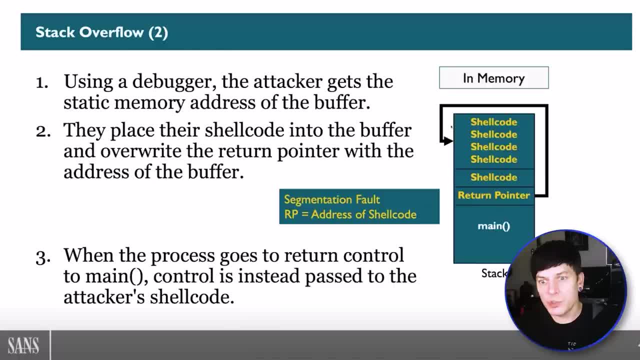 different types of shellcode. the two big parts are: you've got your vulnerability, which you exploit to get control of the process. then you've got the shell code which serves as your payload, which is what you want to execute once you do get control. so what we want to do is put our shellcode into that buffer, overwrite the return pointer with. 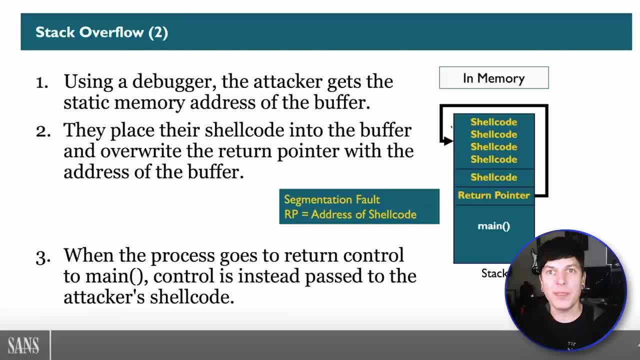 the address as to where that shellcode is in the buffer. then when the process goes to return, we get our payload execution. that's the goal, yeah. so that would be a very basic stack overflow and, as the time has gone on and on, lots of different mitigations have been put into place to try to. 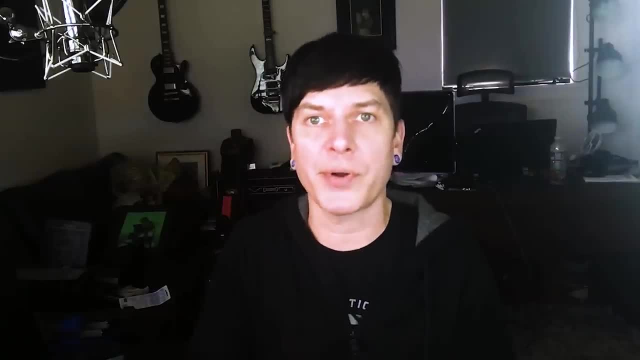 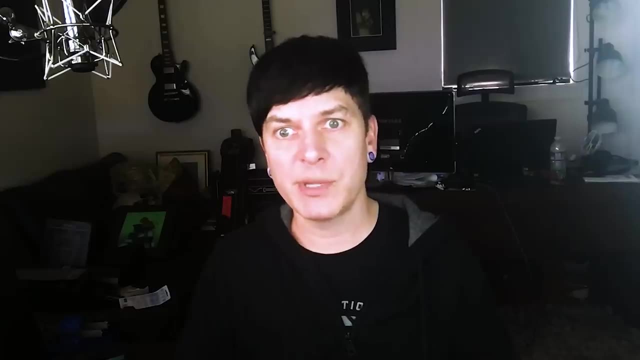 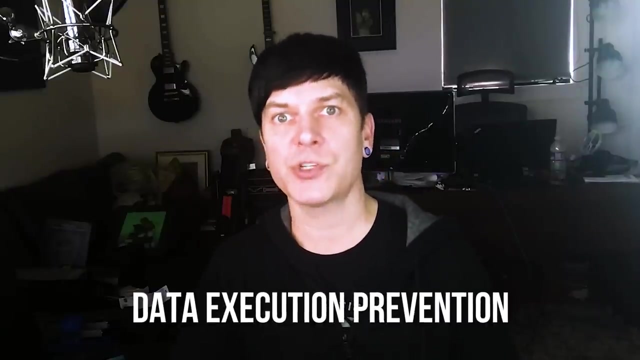 make it so you can't exploit this simple vulnerability. so it's not treating the root cause symptoms. the root cause is the bad coding. the symptoms are obviously these types of things that we're able to do. so an example of a mitigation would be data execution prevention. now this one. 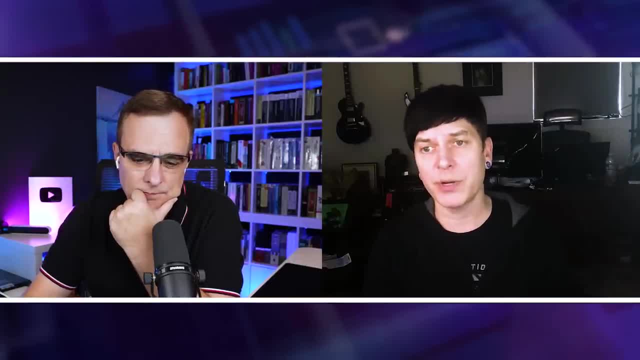 came out way back in XP service pack 2, if we're talking about Windows, but it wasn't turned on by default for all processes because Microsoft didn't want to break your programs. but what that would do in this case if we overwrite the return pointer with the address of our shellcode on the stack, it 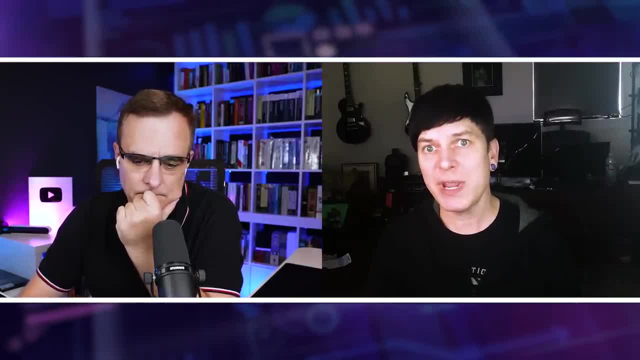 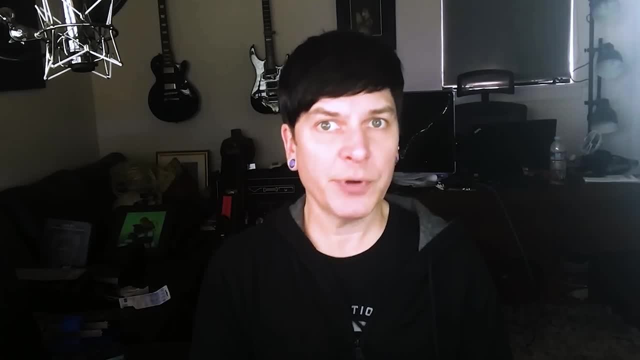 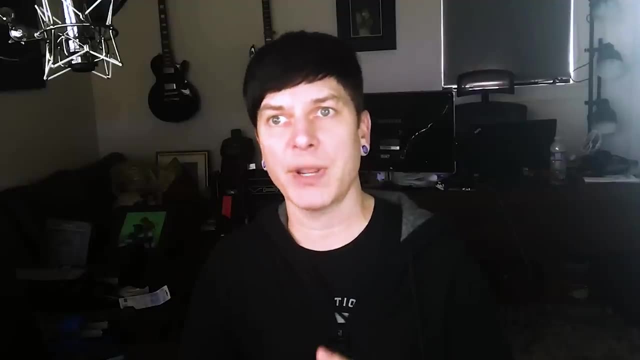 would break the exploit, because the permission that we need, which is execute, is turned off, with depth being on data execution prevention. so that's a pretty effective control. there are ways to get around it. it's like a cat and mouse game, where every time a new mitigation comes out, we try to figure out how to get around. 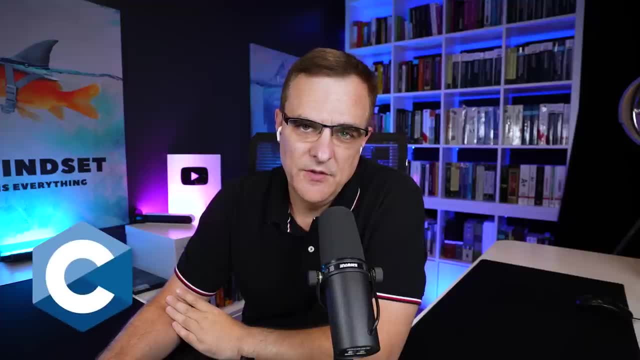 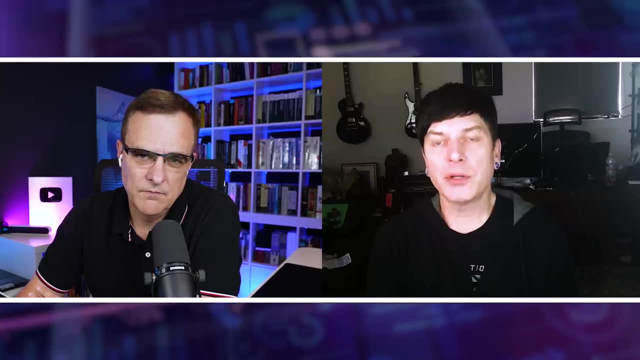 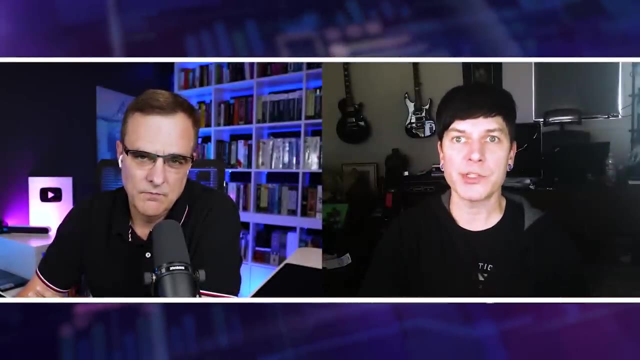 it or avoid it or disable it. Stephen, I always see examples where people using C and using C. here again, is there a reason why C's used rather than say Python? yeah, great question. so these are low level C, C plus plus. these are examples of low level languages. objective C is another one, and 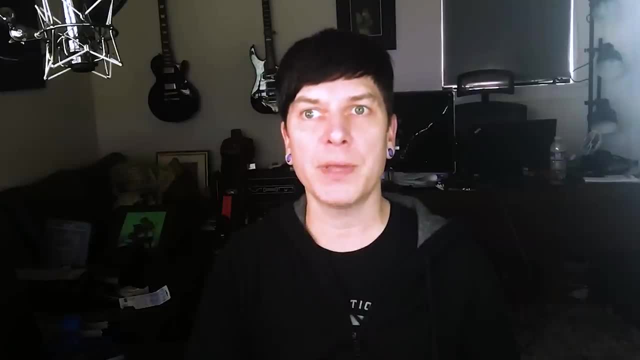 these low level languages are extremely powerful because you have direct access to processor registers, direct access to memory and the power to allocate and deallocate memory and move memory around those low level operations. you've heard that term: with power comes responsibility. right, with great power comes great responsibility. something similar to that you have to be. 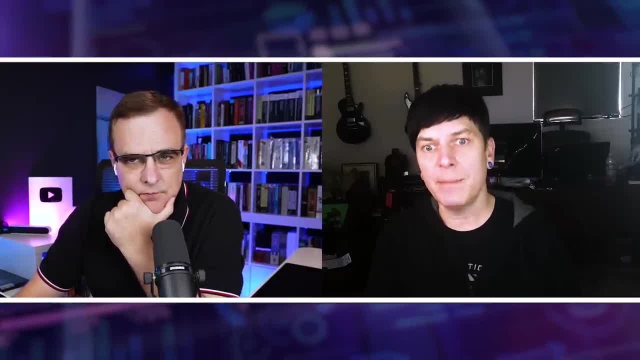 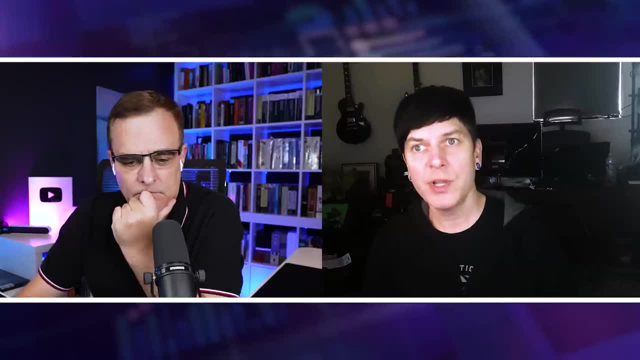 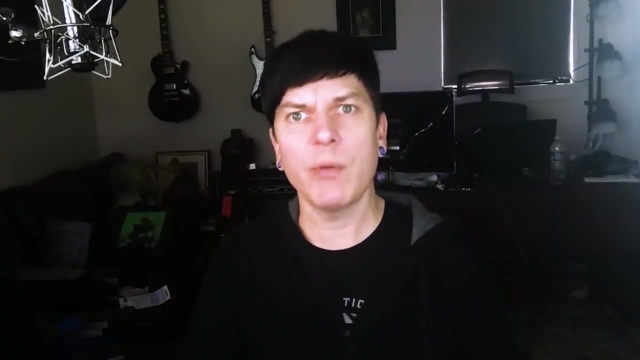 very careful if you're writing in a language like C, because there's no protection, there's no management of the memory that's being allocated and deallocated to protect you, such as a higher level language like C, sharp, so that's, that's kind of the the reason behind it, and you might say: well, 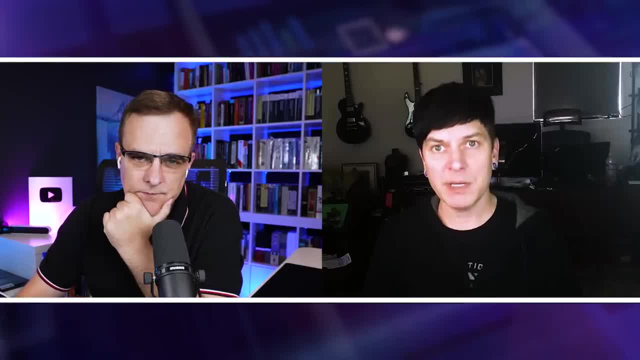 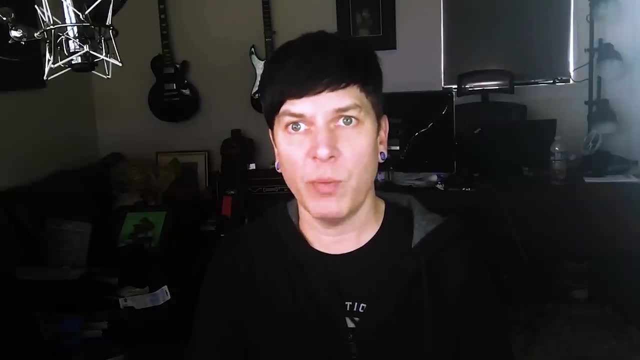 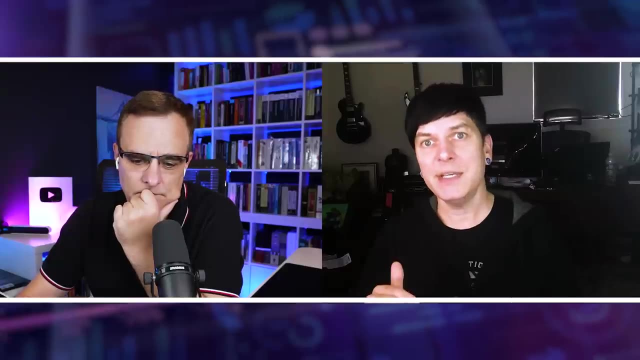 why would people use these low-level languages if they're dangerous? because the speed, the speed and power that you have, you might compile something and the compiler compiles it to a way that you don't like, it is maybe inefficient or it's not allowing you to do something that you want to be able to do so in C. 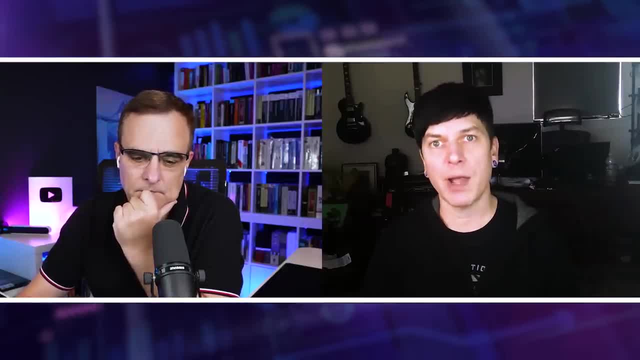 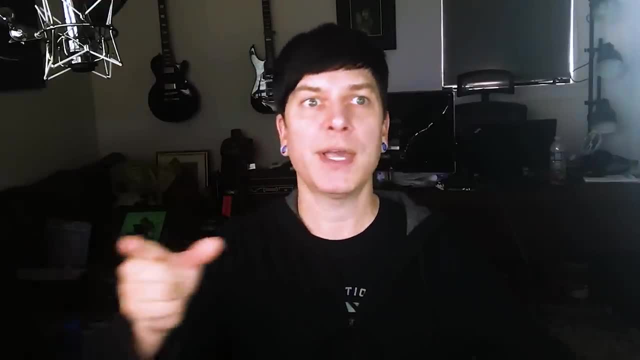 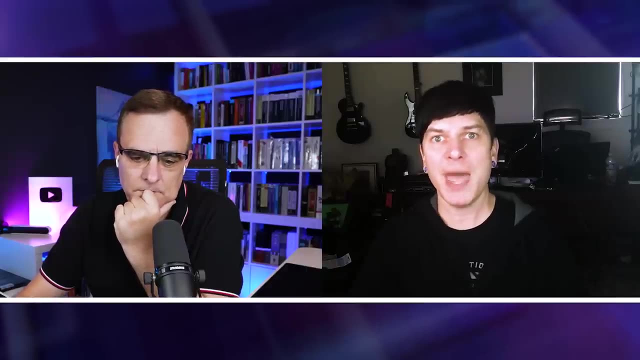 you can just create some inline assembly right there in your program and you can make it do what you want it to do. so you can literally say: move this data from this register into this other register and pop this off the stack. like it's very powerful. so the higher level languages they manage. 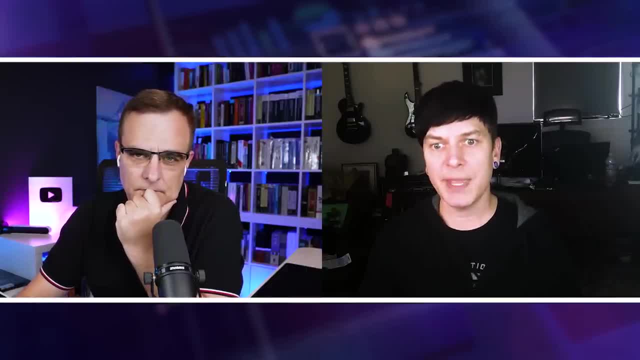 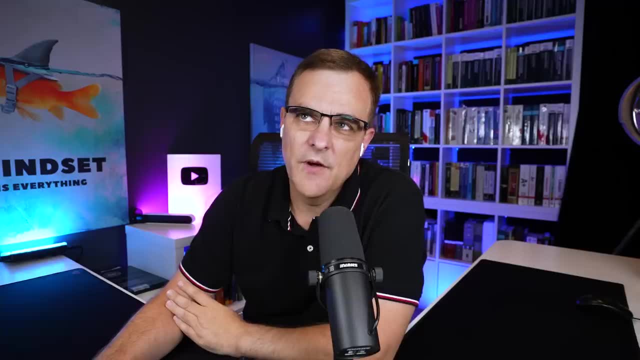 memory for you and other controls and protections to make it impossible or virtually impossible for those primitive or old-school type of attacks to be possible. I've heard a lot of people say you should rather Use Rust rather than see when coding in like production, yeah, and absolutely Microsoft. 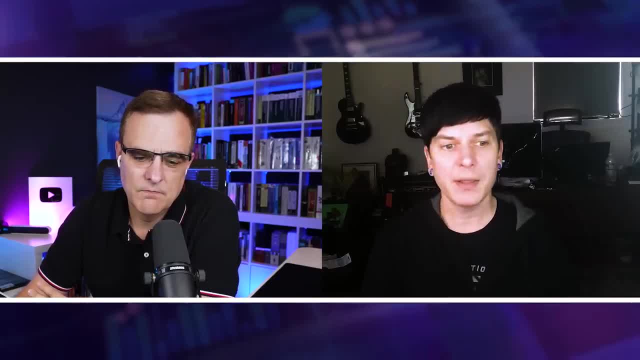 I'm sure You've been watching they. just recently- a couple months back, I think it was Mark percentage or someone, said: hey, if you're interested, check out the latest update. I think it was a preview version of Windows 10 or 11 and win32ksys has some components of it that were are running in rust now. historically you would see Win32ksys, which is probably C++- It's a driver- But then Win32krssys, I think it was. that's the Rust version, or at least part of that has been rewritten in Rust. 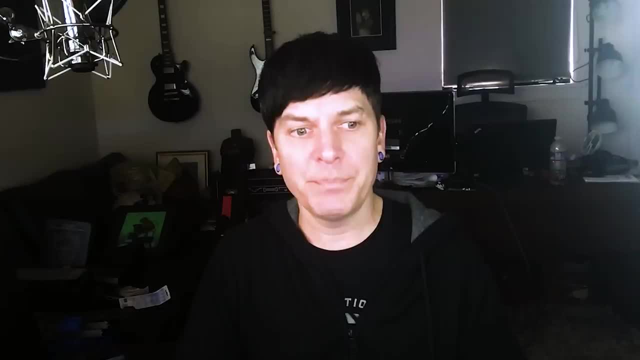 And the interesting thing about Rust is you get a lot of the speed and power that you need, but with this memory safety that you benefit from with the higher level languages, There's a lot to it, though It's going to take. I mean, there's millions of lines of code in. 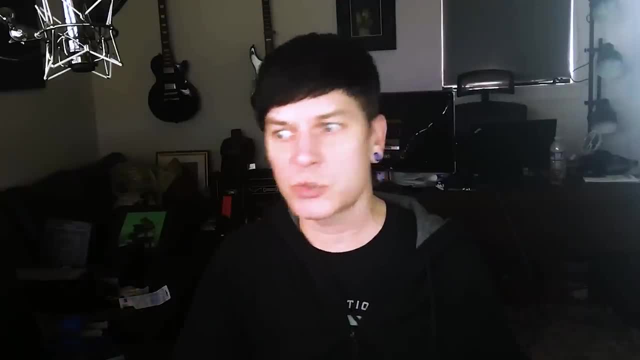 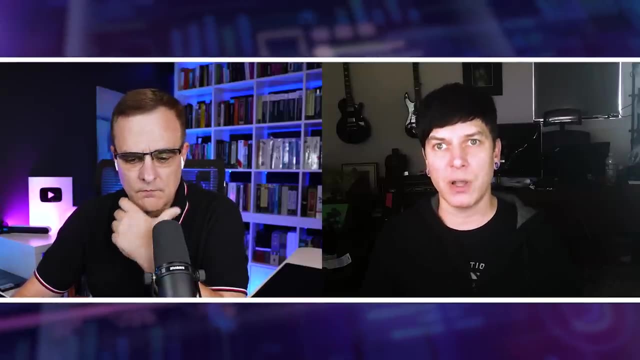 let's say Windows operating system, So you can't just overnight swap all that stuff out. And another issue you run into are limitations with the language, because the language hasn't been around as long and it's not as mature, So something that works fine in C++ may not. 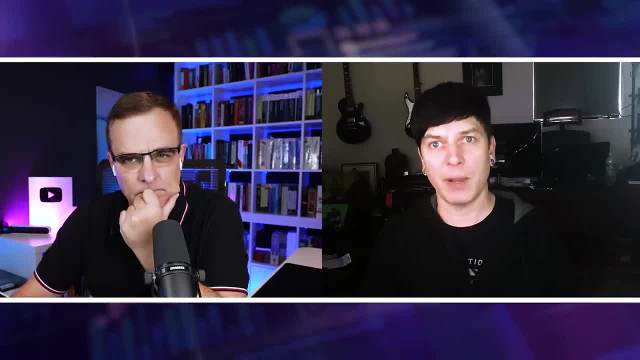 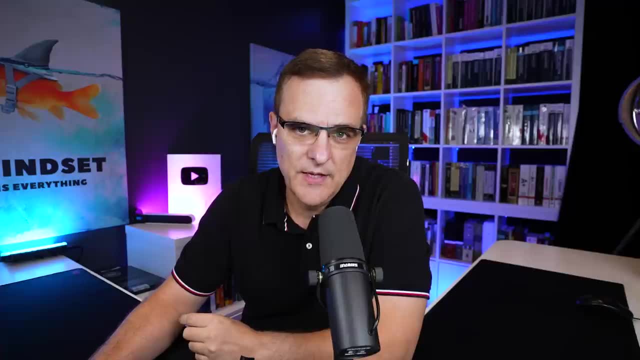 be possible in Rust. So they've got to work with the language developers to actually implement support. But if I was writing an application based on your experience with exploit development and all of this, would you recommend developers today write in Rust when they can rather than C? 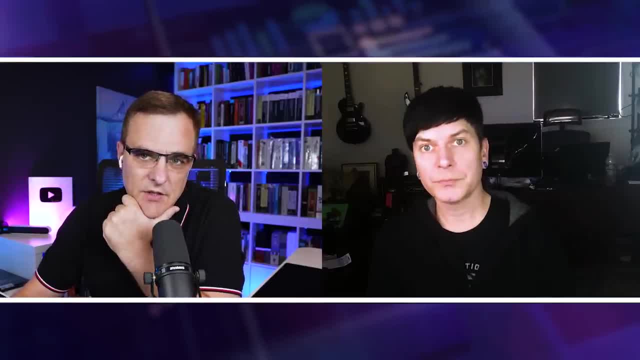 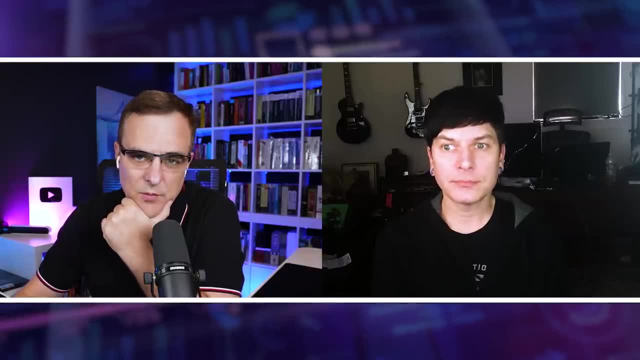 Yeah, absolutely Yeah, Because I mean it's so nice to see this example, because you hear these messages saying: learn Rust or program in Rust, But I mean this is like a really nice visual example of why you'd rather use Rust or Python, let's say, than C, And it's great that you've given us advantages. 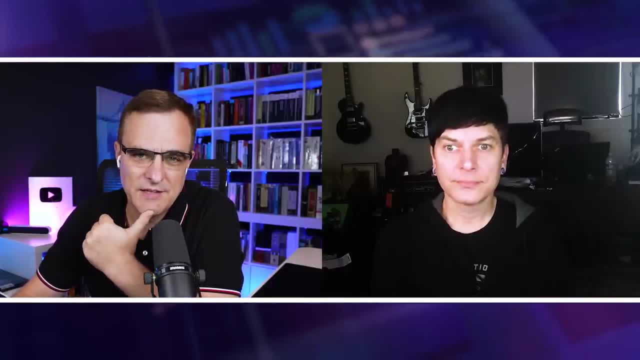 and disadvantages of each. So sorry for taking us on this tangent, but that's great, Great information. Thanks. I always say in the classroom and you've heard this before millions of times: if you have a question, it's a good chance. 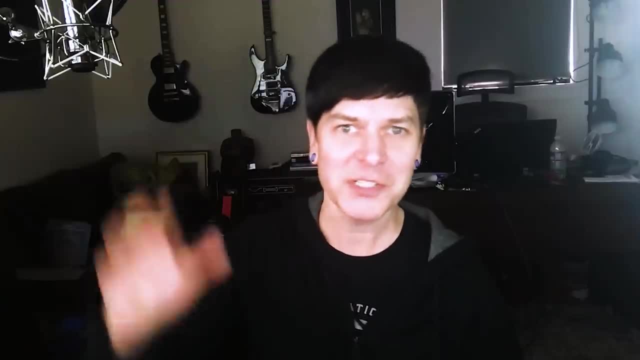 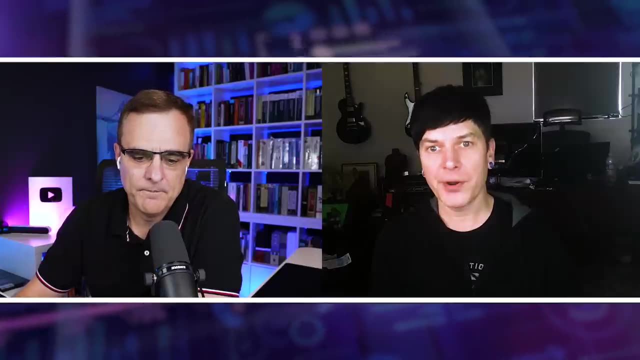 Yeah, there's like 10 other people on that same question. You got to be the one that raises the hand. But yeah, there's- I mean so many of the browsers and big applications like Adobe Acrobat Reader and whatever Editor, And then you've got email clients and the operating. 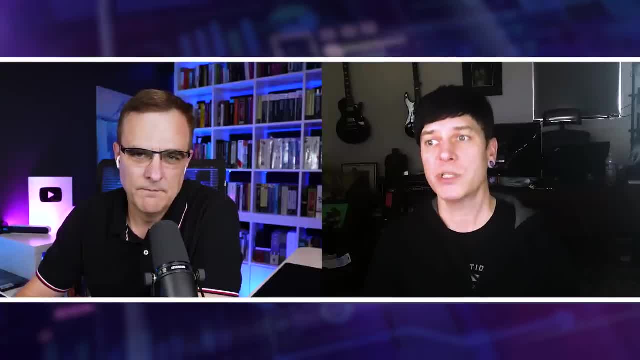 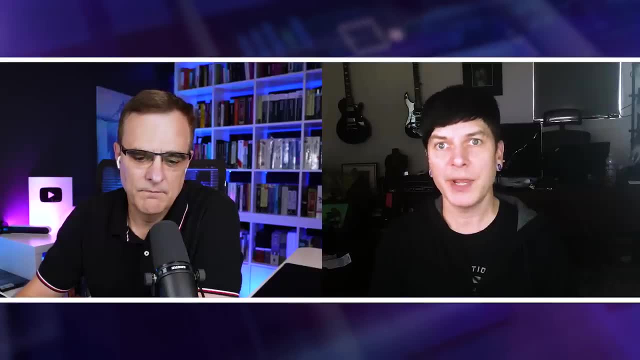 systems themselves and all these big applications. Most of them are in C++ And it's because of that power and that speed that you get with that language. And you're having to go and now train a lot of legacy developers who have so much history and experience with C++ And now they've 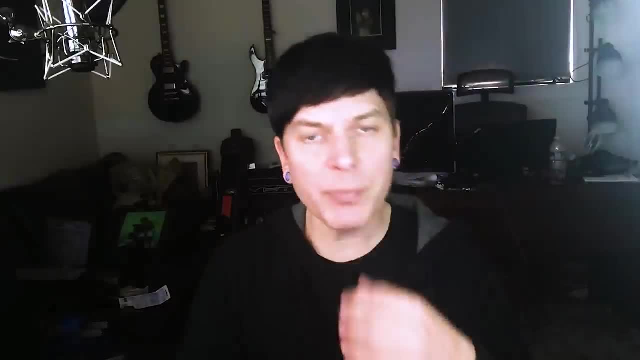 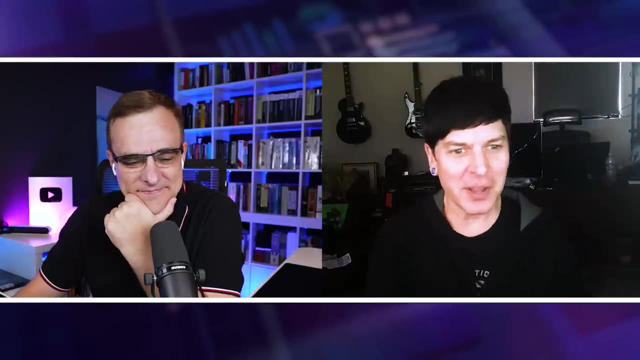 got a lot of new language And that's going to be come with a set of challenges. I want to jump over to the command line in a little bit here and see if we can get ourselves into some trouble, So we'll see what we are able to make happen. But I want to show you one more example of a different type. 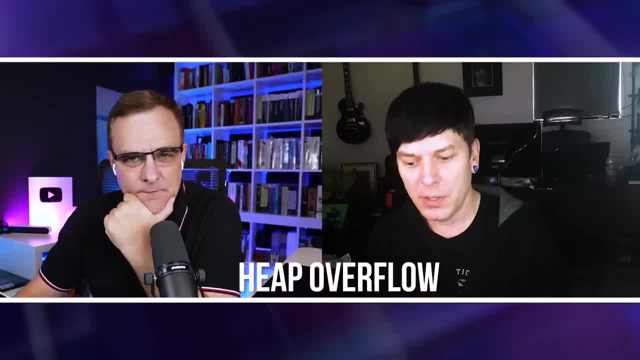 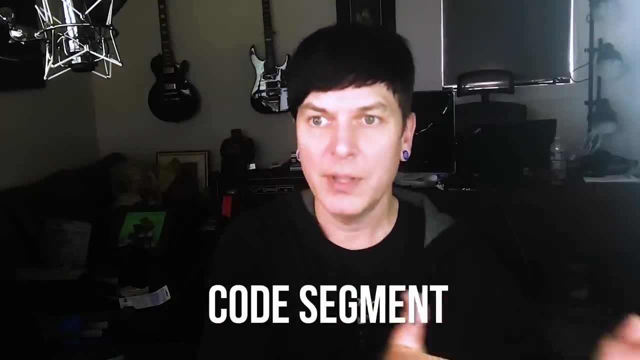 of overflow that I mentioned earlier, which would be the heap overflow. So the heap is actually a different region of memory than the stack, And so when I say different regions, like the code segment, the stack segment, the heap segment, what that really means is your. 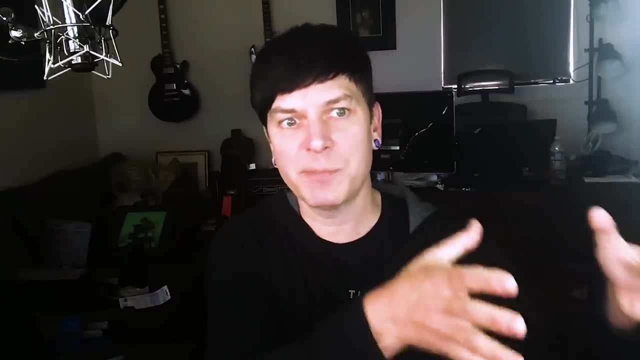 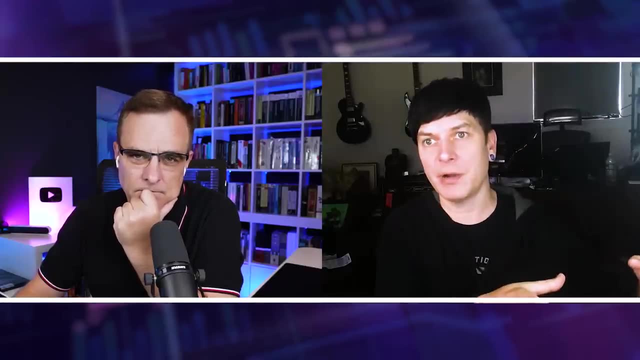 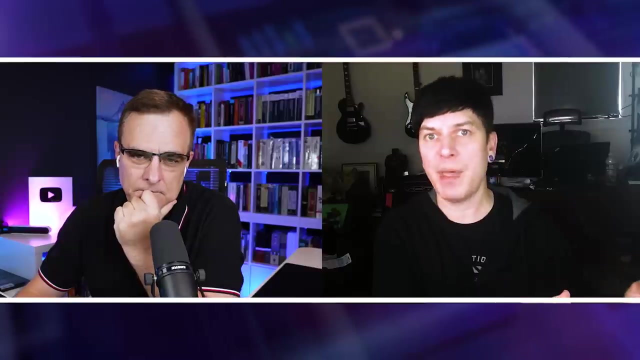 carving out a different section in virtual memory that's specifically been reserved and allocated to support one specific thing. So the code segment is specifically there to hold the executable code associated with the process. So in that case you can mark that region of memory with the execute. 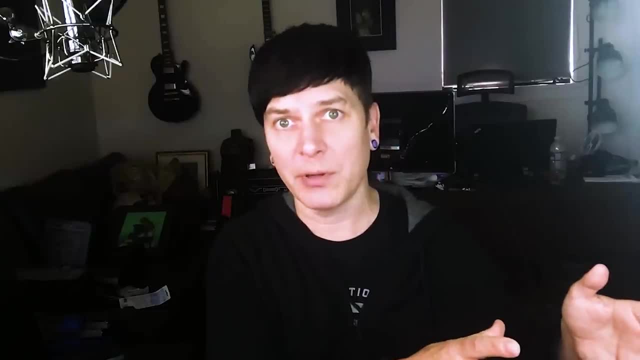 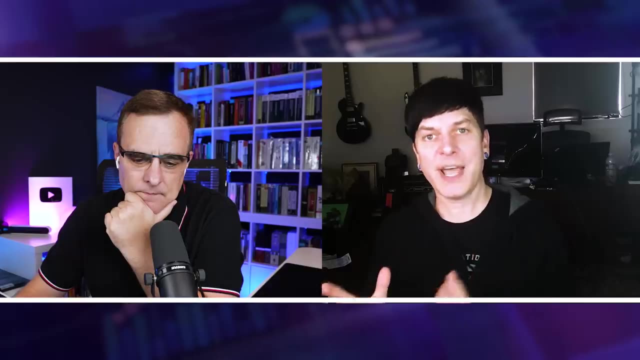 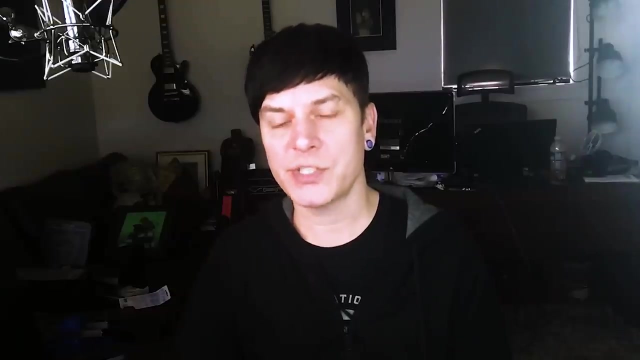 permission being on because it has to be on, but you don't want it to be writable, So you turn the write permission off And then all the other segments, like the stack. to simplify, what the stack is is a specific region of memory that is used for function calls. Every function call gets its own. 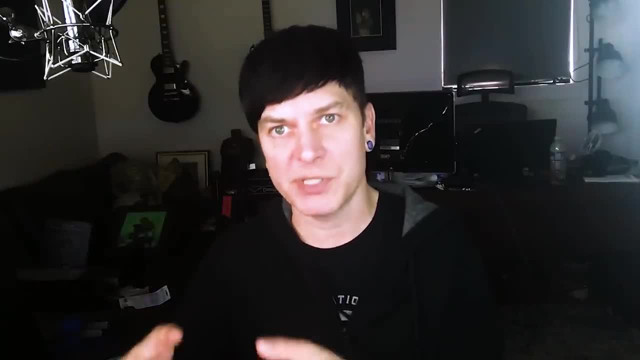 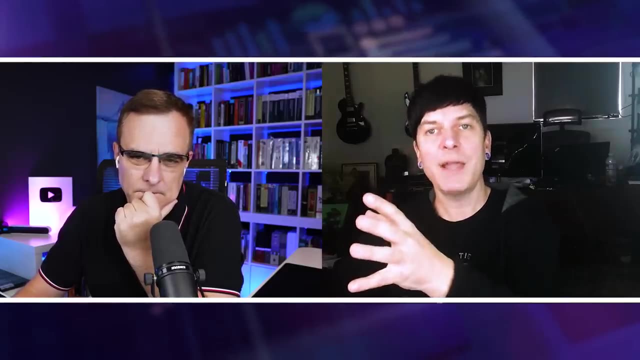 stack frame, which just means a small little allocation reserved specifically for that function. It goes through something called a prologue: at the beginning of the function that sets up the stack frame And then at the end of the function you go through an epilogue and that. 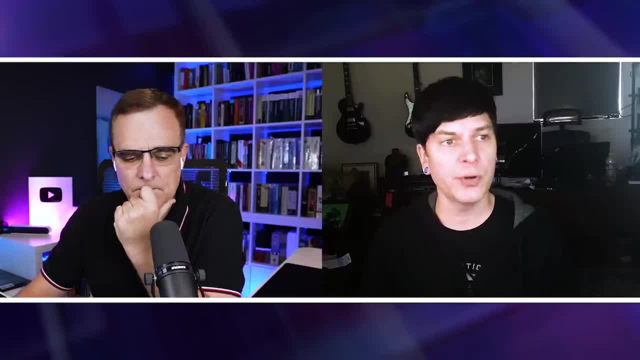 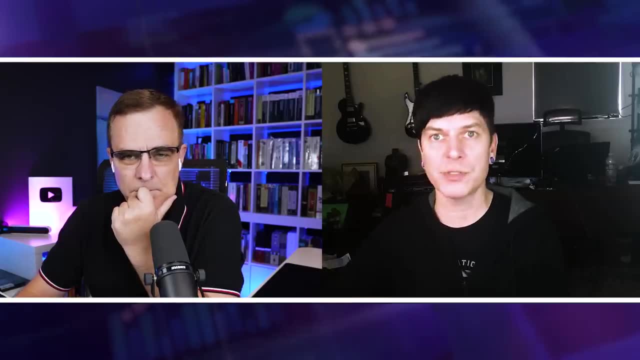 tears down the stack frame And that is all compiler inserted code. You as a programmer don't need to care That stack memory again, it's for finite operations, for function calls. You get in, you get out. Now, when you talk about the heap, 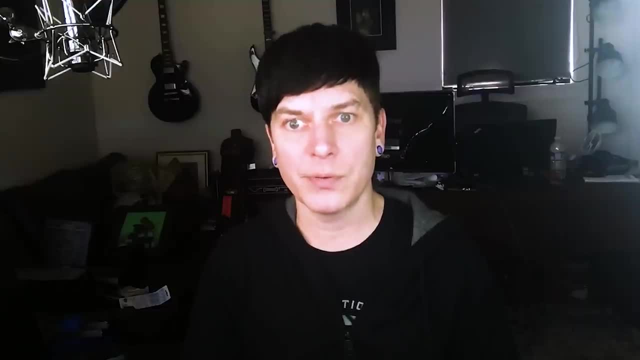 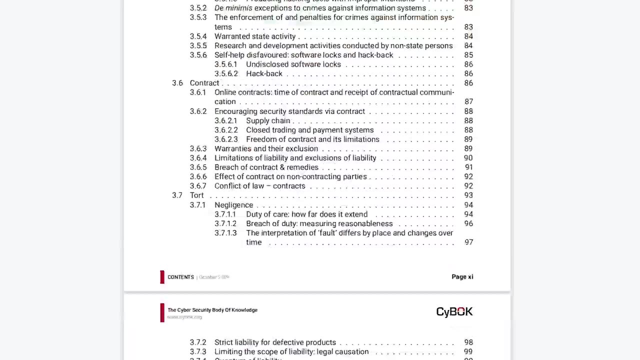 that's a more dynamic area of memory, And let me give you a good example So it'll help you understand. Let's say that you're using Chrome and you're navigating the web and you go to a website that's actually a PDF document. So you're now in your browser window viewing a 10 megabyte. 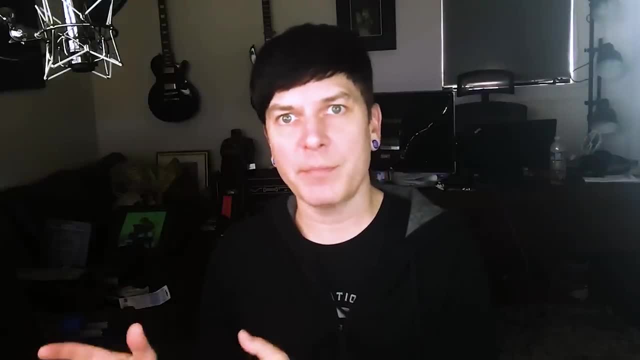 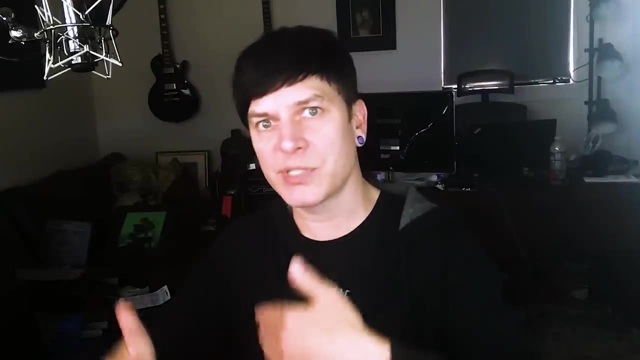 PDF document. The stack is not a good area of memory for that, because the stack is, like, really closely tied to the code segment where I can see the stack. So I can see the stack and I can see the memory again Every time as the process is running, as functions are called that function. 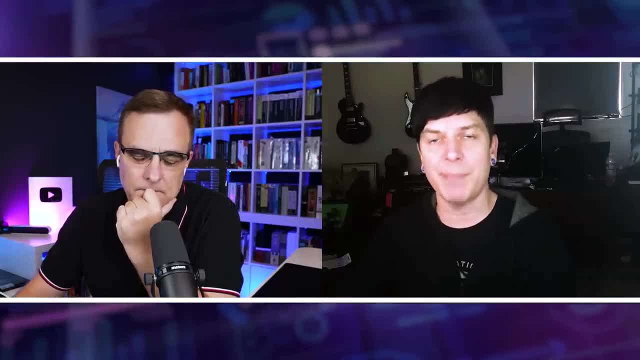 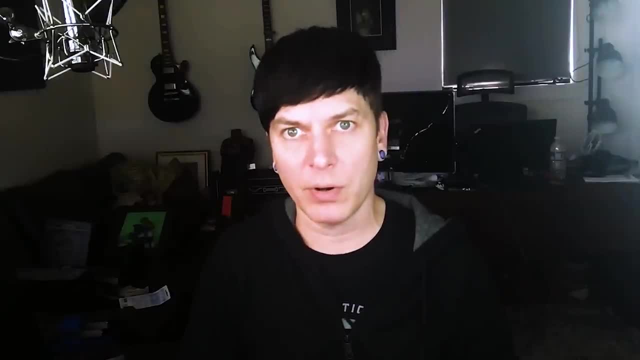 that gets called gets its own little stack frame And it's just constantly going on and on in the background versus the heap. That would be a good place to store the memory associated with that PDF document that we're looking at, because it's not finite. The developer of the browser has no 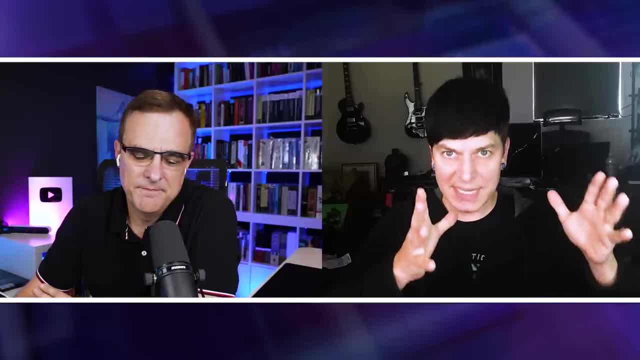 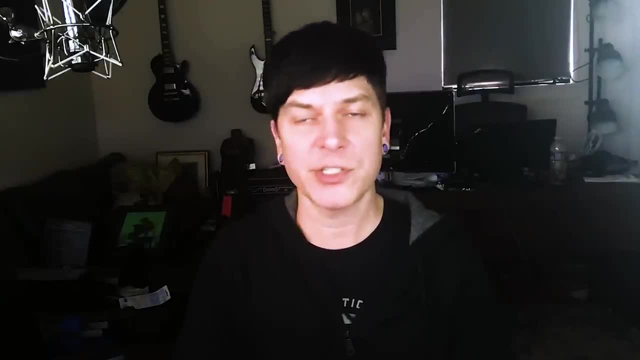 idea how long you're going to keep that window open. We need to leave that memory stay in use and resident until the user goes to the URL and changes it to the code segment. So that's a good place to store the memory. So that's a good place to store the memory. So that's a good place to. 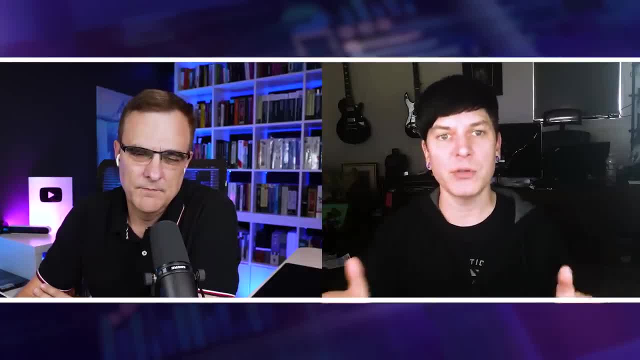 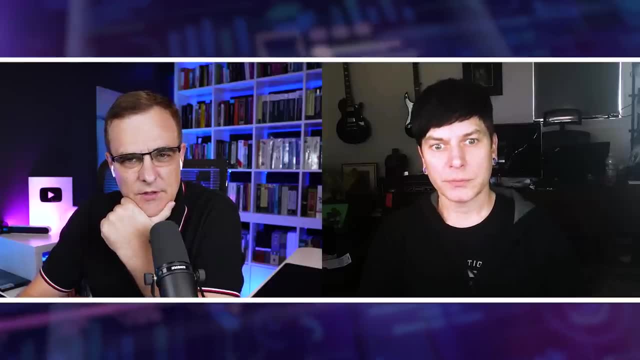 Google homepage, Then we free all of that memory that was being used up by the PDF document so it can be recycled and reused by the process. And the heap, if I understand right, can also be very big files, So like. hence the example of a 10 meg PDF, or it could be 100 meg. 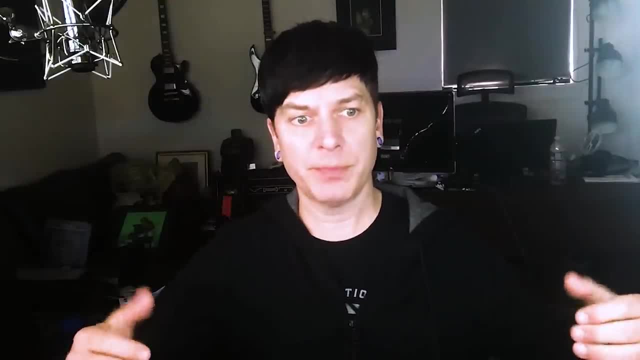 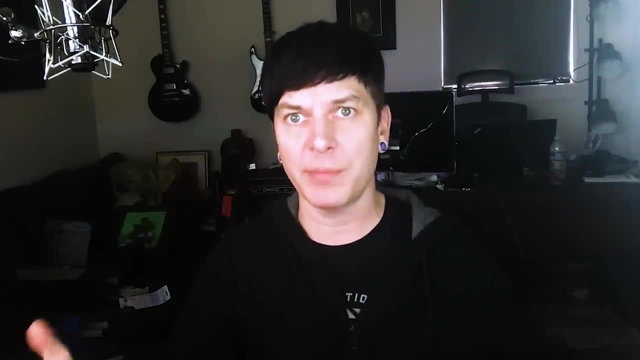 or something, right, Yeah, So the heap and the stack are both considered dynamic regions of memory that are able to grow, And so, therefore, they don't play nicely together. You got to keep them apart from each other because you don't want them colliding into each other, So you'll. 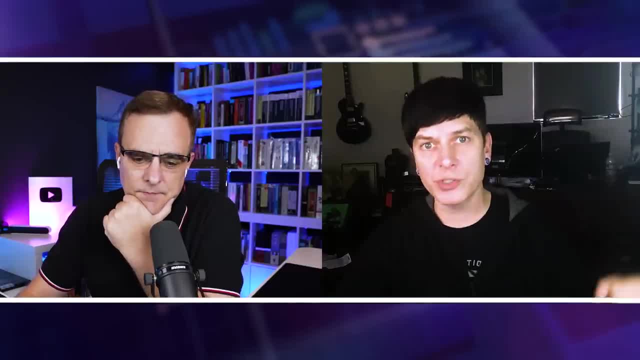 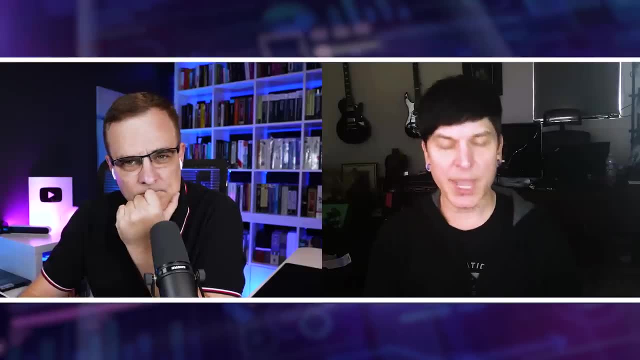 multiple gigabytes away from each other and growing towards each other, and they should never collide, or you'll see them growing away from each other. That's how Windows does it. So, again, the heap is for dynamically allocated memory that doesn't have a finite lifetime. The interesting 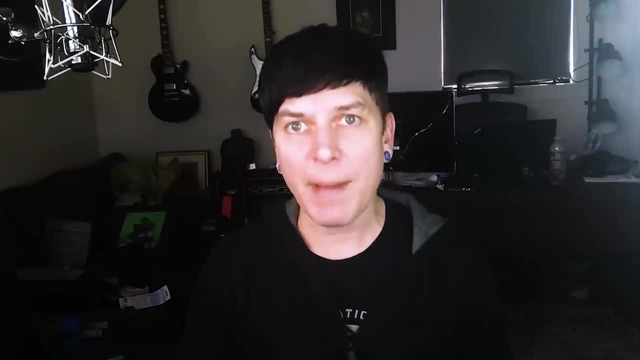 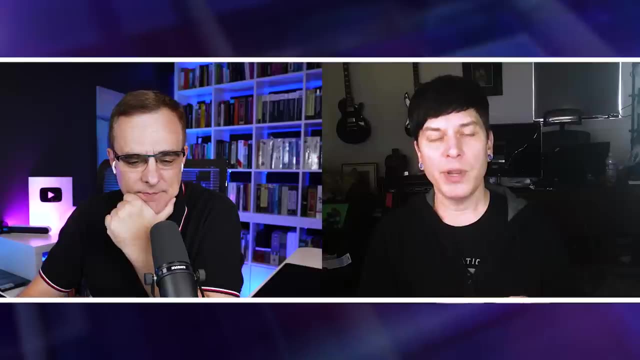 thing about that, though, is- this is another area- We're not going to go down the rabbit hole into this, but vulnerabilities like type confusion, use after free- those are heap related vulnerabilities When, if you're familiar with programming, you know what a function does. We call it. 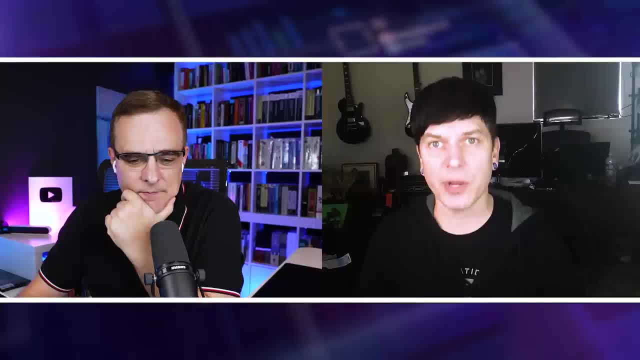 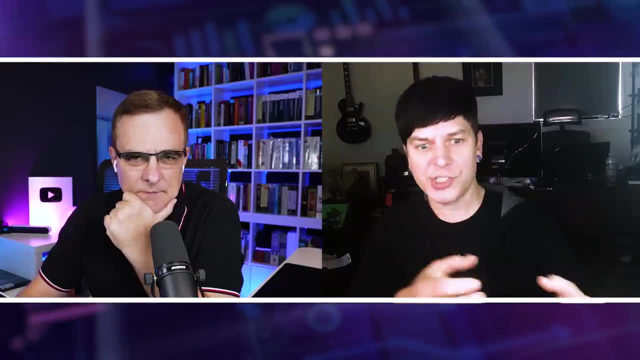 function, Like: maybe we create a calculator function and it wants two arguments. give it two numbers and it will multiply them together and return back to you the product. That's again, the function is just taking those numbers, multiplying them, displaying the result and 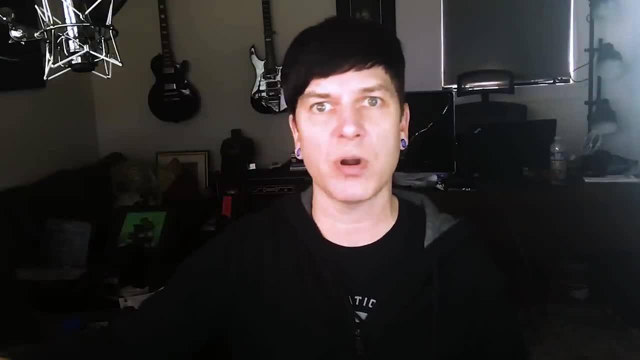 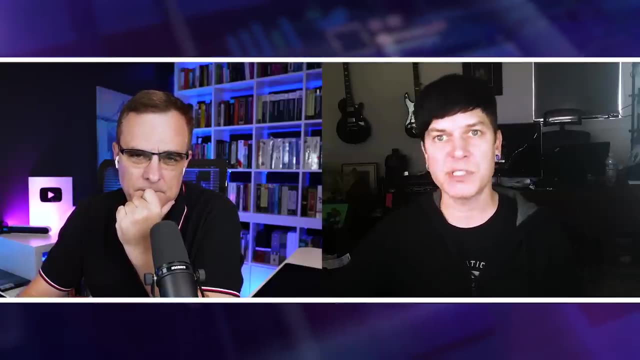 returning out. So that function call doesn't store or preserve anything that you just did. It's just a little template that you can call over and over again to do a very specific thing: You get in, you get out, versus the heap Heap memory is. 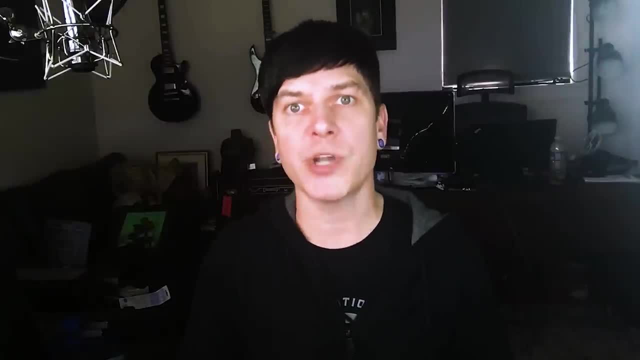 once it's allocated, we, maybe, maybe we want to create an object. You've heard of object oriented programming, I'm sure. So let's say you want to instantiate an instance of something called the dog class and this dog class, to use a silly analogy, you can choose the breed. 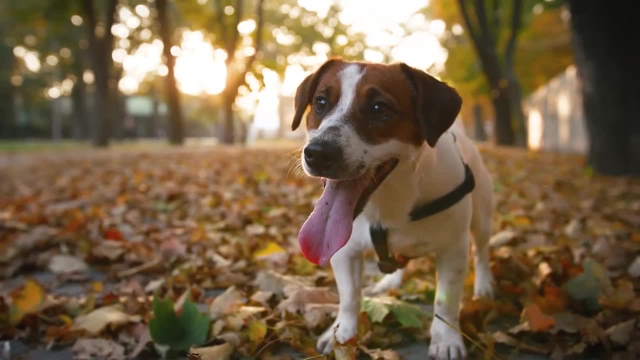 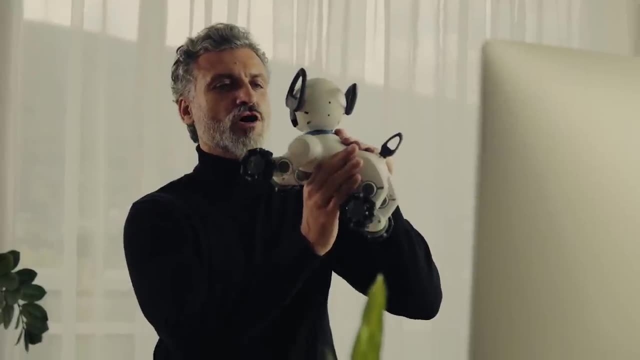 of the dog and various attributes such as like the fur color, the size of the dog, the eye color of the dog. Those are all the attributes you can select. And then you've got the methods or functions, like sit, roll over, lay down, speak, And when you instantiate an instance of this dog. 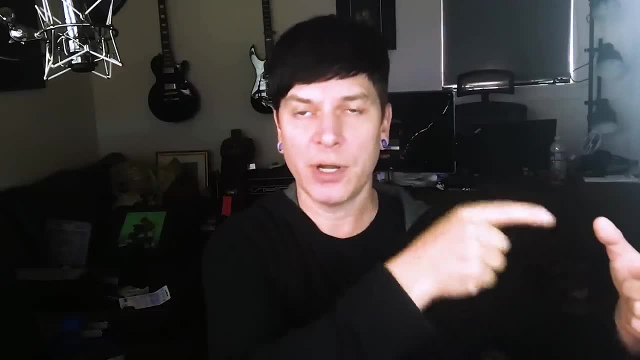 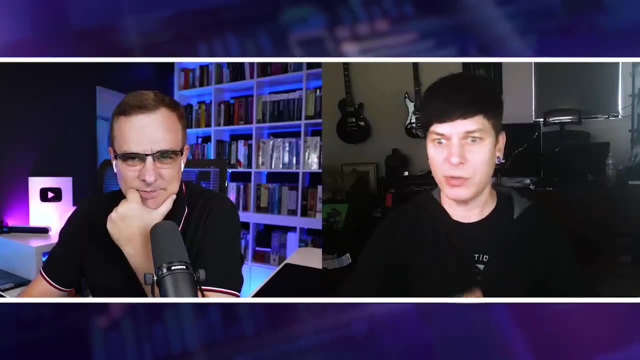 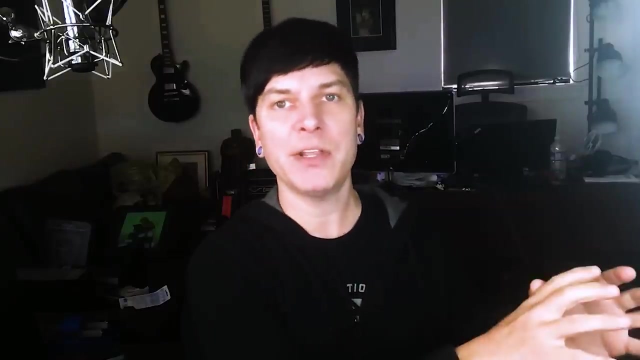 you can then reference that dog, the object, and say dogspeak or dogsit, And that instance of that object will do those things you're telling it to do, And you can instantiate as many instances as you want. This all lives out on the heap. It gets very complex because something has to manage. 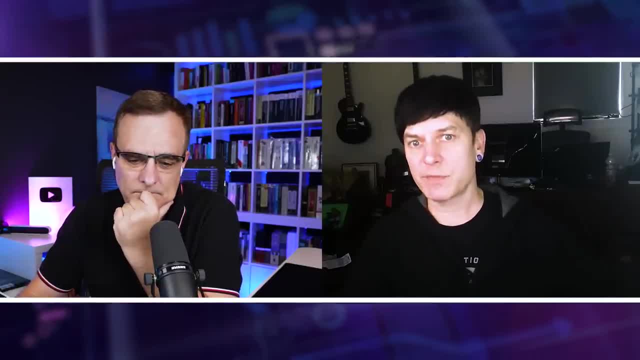 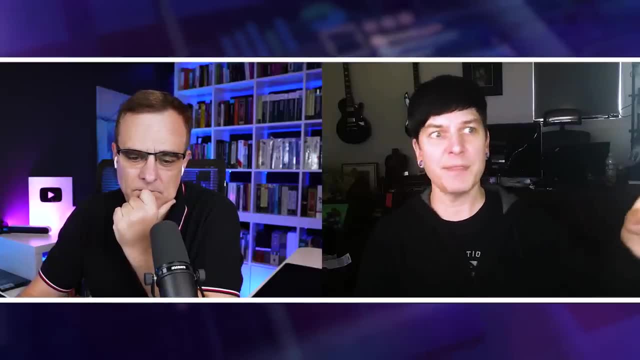 that memory and manage those objects, so that this vulnerability class called use after free. for example, if we're somehow able to trick the process into thinking that that object is no longer needed and it destroys it and gives it back to the heap, what if the process still needs it? 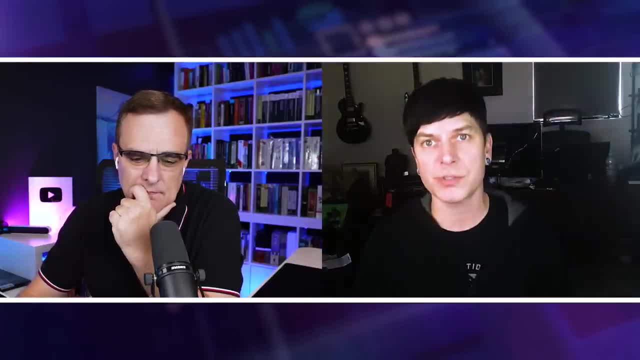 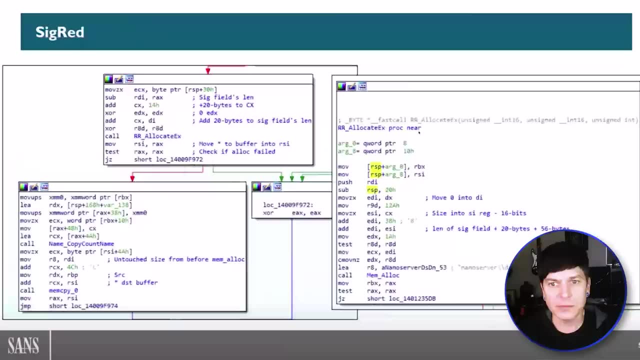 It goes to access that object that's supposed to be there, Oof, it crashes. So it gets very complex out there on the heap. But this example- I'm going to show you what we're looking at here and I know it's a lot of junk. it looks like seemingly this is a disassembled program. 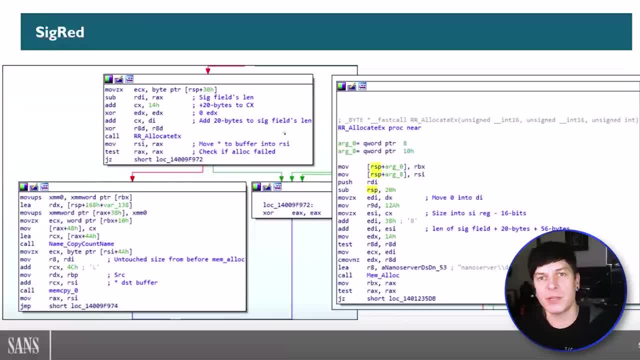 a small piece of a function of a disassembled executable. Specifically it's dnsexe from Windows. This is a piece. what we're looking at is where the vulnerability resides, from SIGRED. if you heard of that vulnerability from a number of years ago, It was a very critical vulnerability. 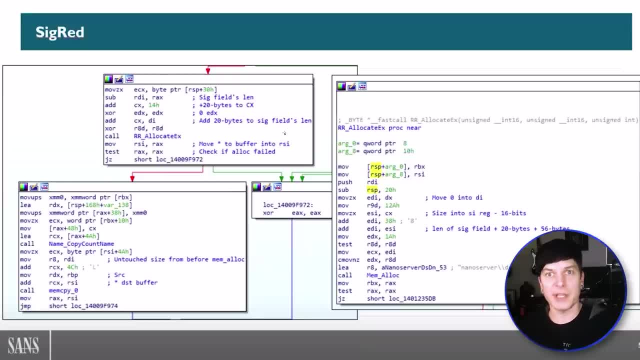 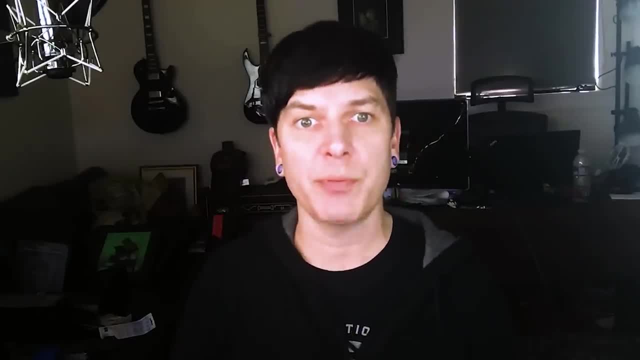 because it affected DNS, which is a publicly accessible service. So obviously from an attacker's perspective, that's very interesting. The researchers that discovered this vulnerability were from Checkpoint. On the left we've got a snippet of one function, And on the right 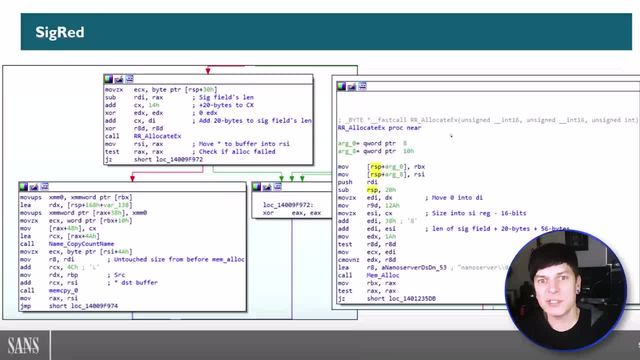 we've got a snippet of another function. The snippet on the right is called by the snippet on the left. So see, I'm using my mouse cursor. I know it's small. See where it says: call rrallocateex. The little snippet on the right is rrallocateex. 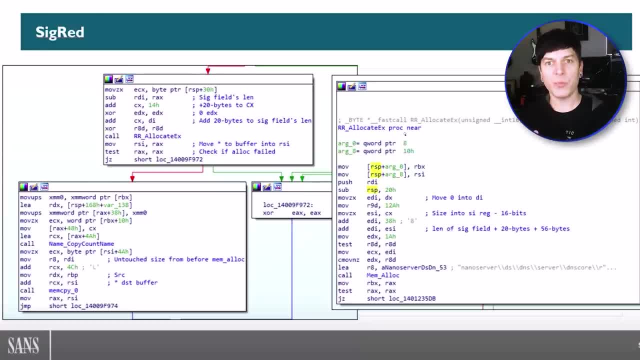 disassembled. So what does disassemble mean? That means when we've compiled a program the kind that you double click on to get it to run. that's all in machine code, So it's basically hexadecimal. And that hexadecimal that you're looking at are opcodes and operands, So that's. 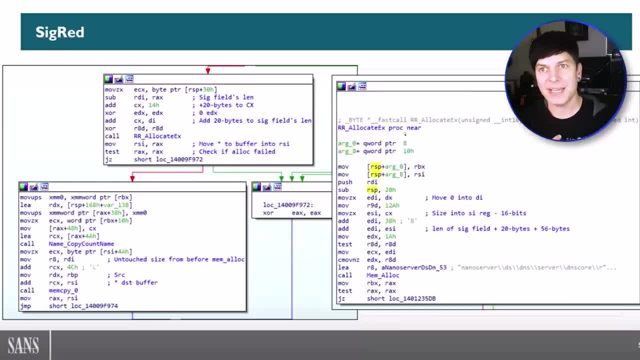 what the processor uses. Obviously, for us that's not easy to read. a bunch of opcodes like 90, EB 06, 34, 41. I mean, that's pretty crazy. So what a disassembler does is it takes those opcodes, it disassembles them. 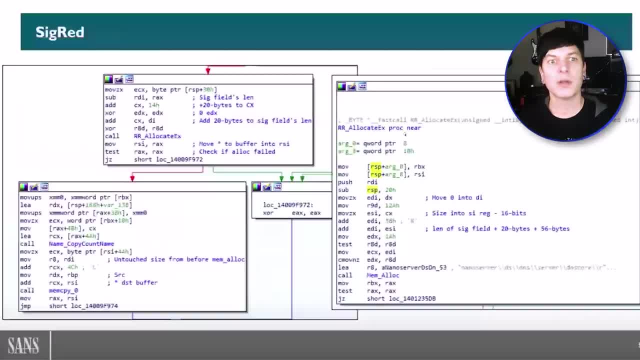 into their mnemonic representation, which is what you have here on the screen, called disassembly. It's still not easy to read. This is very low level of what we're looking at. This would be an example of x86, 64-bit disassembled code. 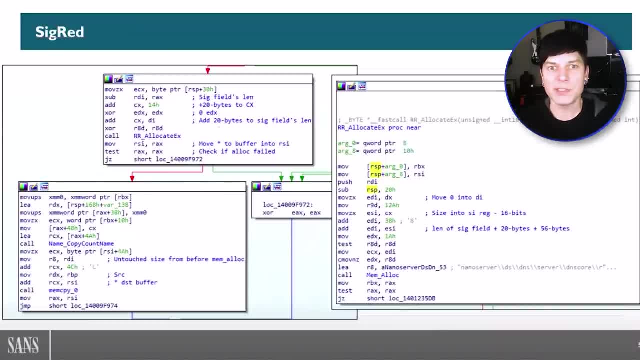 It's these little. there's a little bit of blue on the right everywhere. That's comments that I added in but I'm not going to take like. I'm just going to really quickly show you what the issue here was. You can see down at the very bottom. call memcopy. Memcopy is a function that has a. 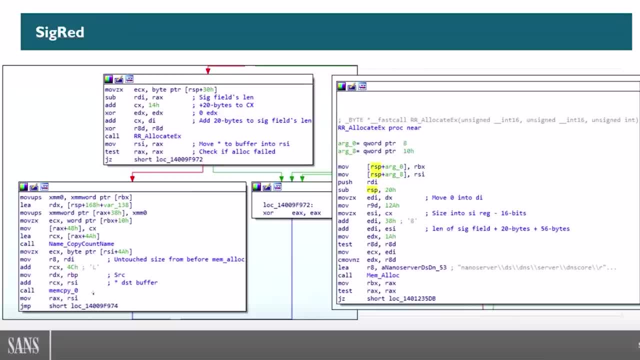 size argument. So you would think, if it's got a size argument we can specify the maximum number of bytes that are permitted to be written to the destination, preventing a buffer overflow. So stircopy didn't have that option. There was no size argument. Memcopy does, So how would there be a? 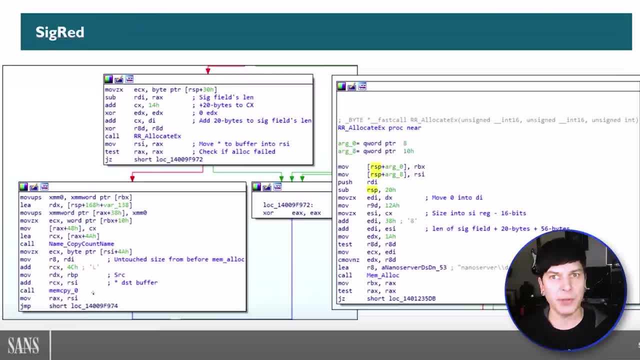 vulnerability. Let's talk about this because this gets. it's where it gets complex, Not what we're going to talk about here. but what gets complex is the calculation of that size argument, Because oftentimes we can't statically specify what the size is, So it has to be calculated from something. 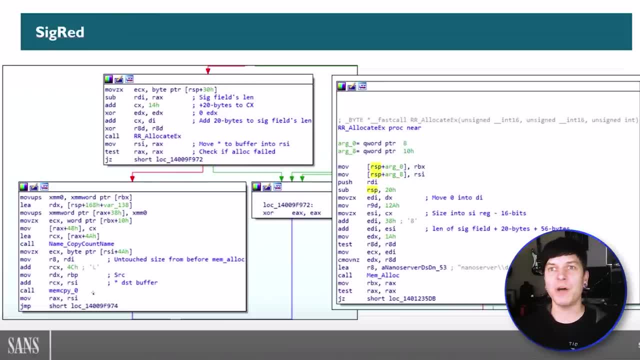 else And that something else unfortunately oftentimes is user influenceable. That's a word that we can influence that calculation. Now, to be able to influence that calculation can be quite complex, And that's where the research comes in. But what's going on? 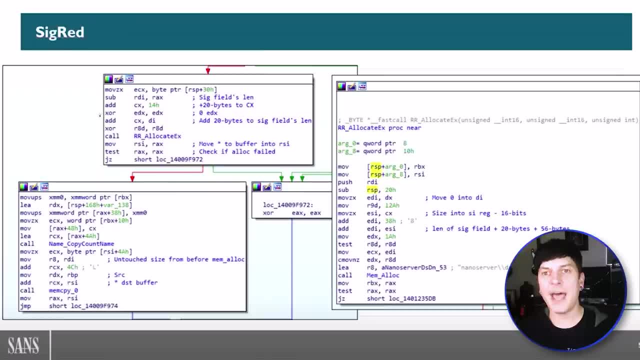 here is. there was a special DNS query type. That DNS query type allowed for you to do interesting things Like normally DNS runs over UDP port 53, but DNS can also run over TCP 53. That would allow us to increase the size and have, you know, Axe and Synex and stuff like that. Like it increases. 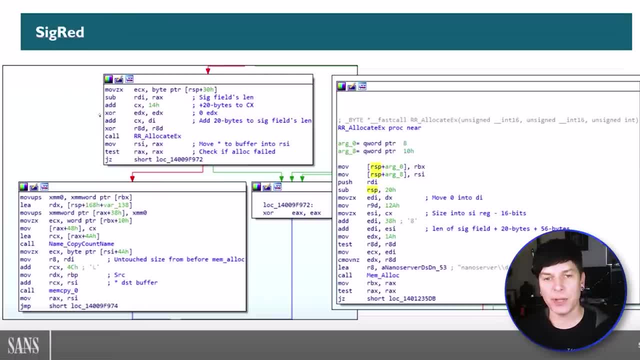 some options And this specific type of DNS query through compression and other factors, allows you to massage or groom how much data ends up needing to be copied to a destination. So this call to RRAllocateEX. if you look in towards the bottom on the right it says call memalloc. That's the actual function that allocates. 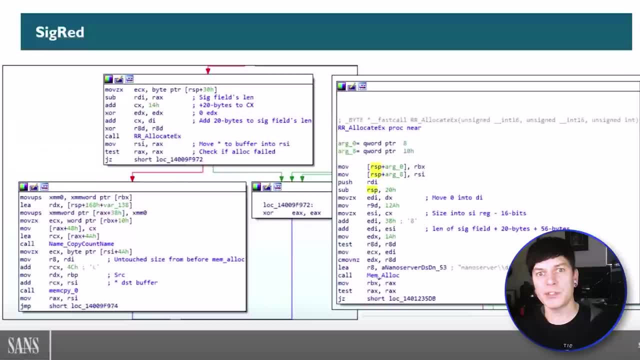 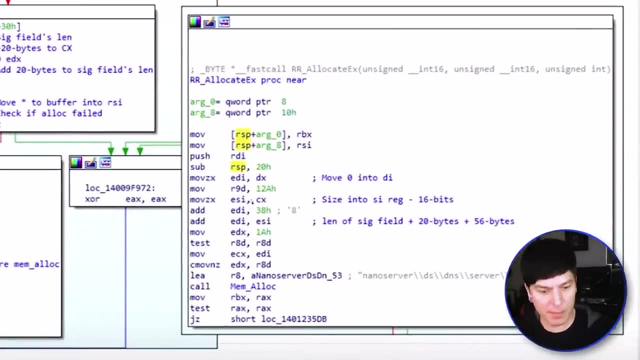 the memory on the heap to store the data associated with this DNS query. So we've got to allocate memory to store the data associated with this DNS query And that's where the research comes in: dns query coming in across the socket. so the issue that happens here is, if you look and maybe you can, 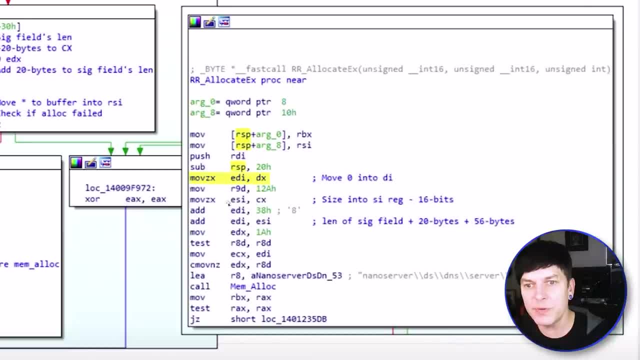 add in after the fact a little pointer here. it says: move z or zx, dx into edi, move zx, cx into esi, dx and cx. those are two byte processor registers, two bytes, so two to the 16th power maximum, 65,535 max. only the lower two bytes of this processor register are being taken into. 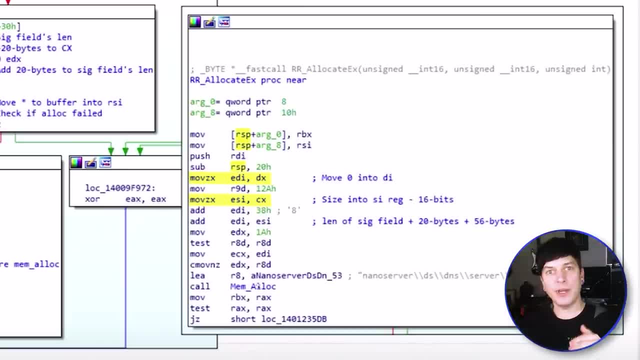 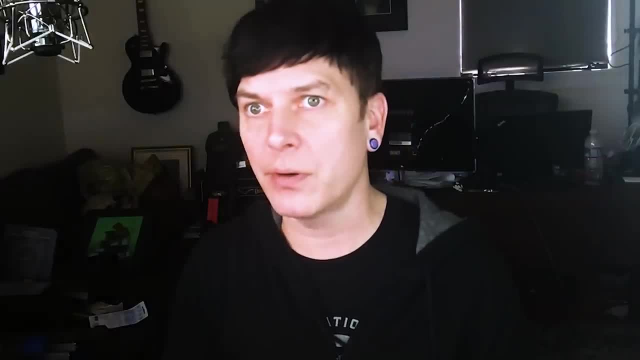 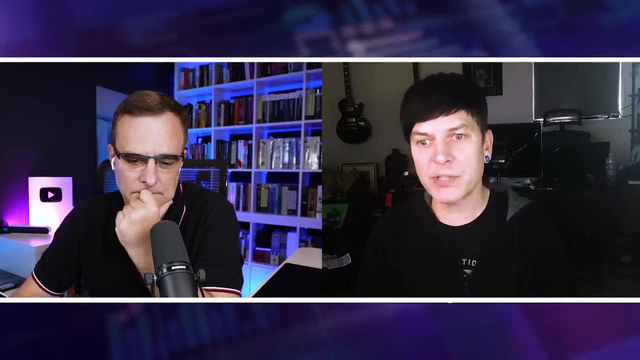 consideration for the memory allocation. so, in other words, the maximum memory allocation can be 65,535. that's the max. because of this vulnerability in the code, it should not be limiting to only two bytes, but it is, and what happens is we get into trouble because there's 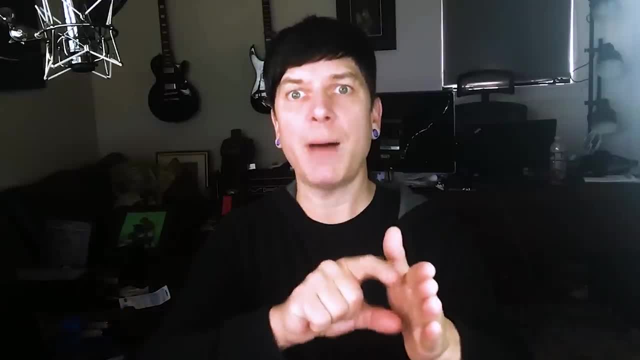 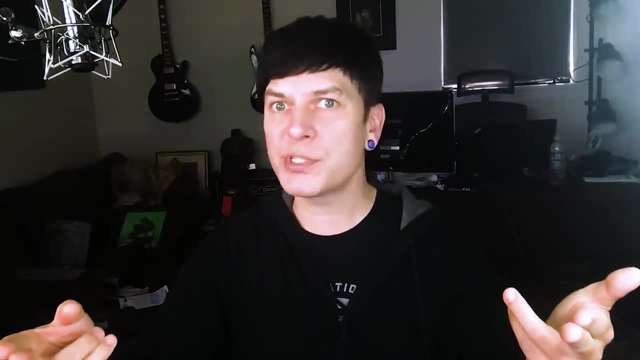 something called an integer overflow. if you've ever looked at an odometer and the odometer says 9999999. when you add one to that, what happens turns over. yeah, it rolls over back to zero, or does it really? those digits roll over to zero, but it carries the one to the left right. 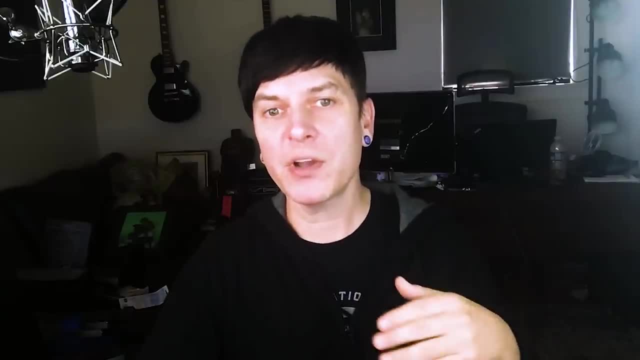 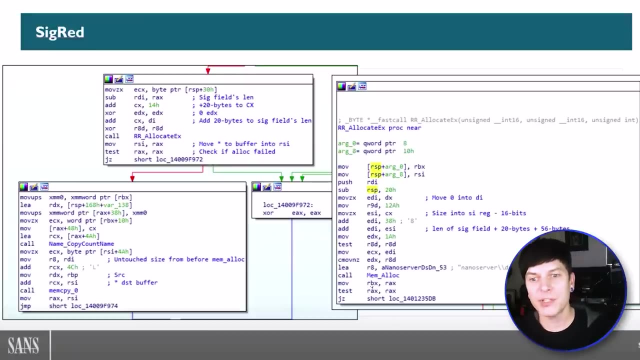 so that ends up becoming the issue. if we can cause an integer overflow rolling over two to the 16th power back to zero again, the memory allocation that gets made- because it's only looking at the lower two bytes- ends up being really tiny. meanwhile, if we go back to the caller mem, copy is what. 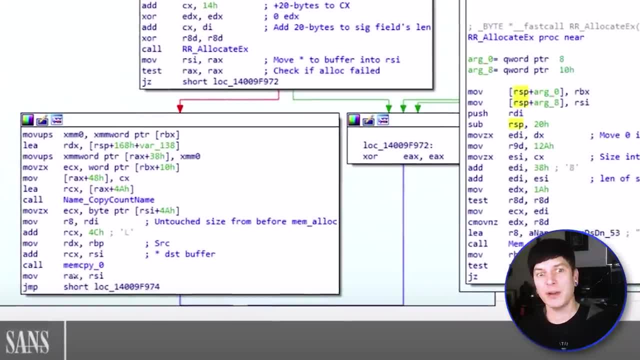 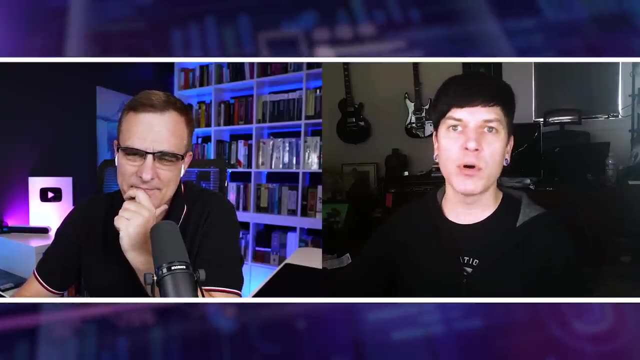 actually needs to copy the data to that destination buffer that's been allocated. mem copy takes in a unsigned 32-bit integer, so four bytes are taken into consideration, not just two. so you see where i'm going. so what's going to happen? there is, mem copy will happily copy in way more than two to the 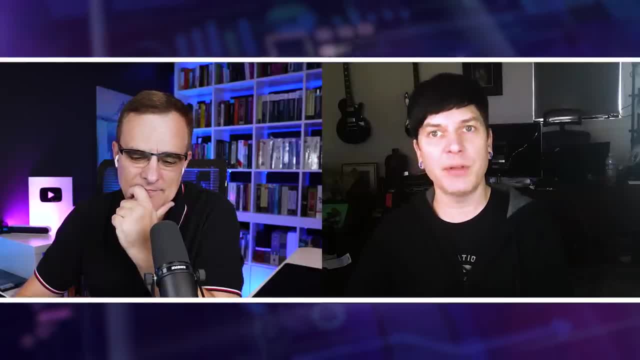 16th power to the destination buffer. that wasn't capable of ever holding that much data, so it results in a very small number of bytes and it's going to be a very small number of bytes. it's going to keep overflow and that's where we got into trouble here and that occurred on the 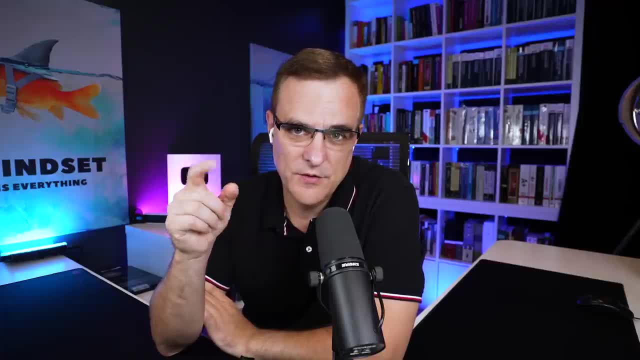 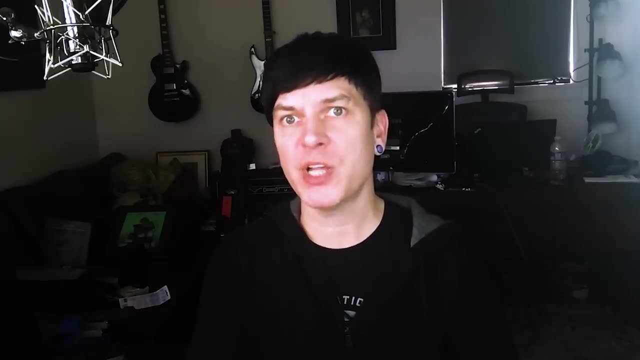 server right or was it the? so the client was able to get overflow on the server? yep, it was a server side vulnerability. so, as you can see, just just from that explanation- and i tried to simplify it as much as possible, but just based on that, that information- you can see how much more complex it. 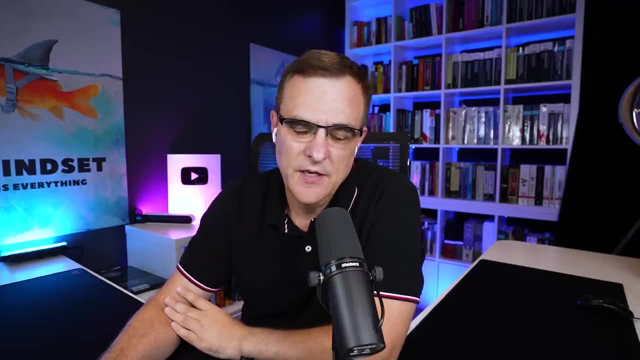 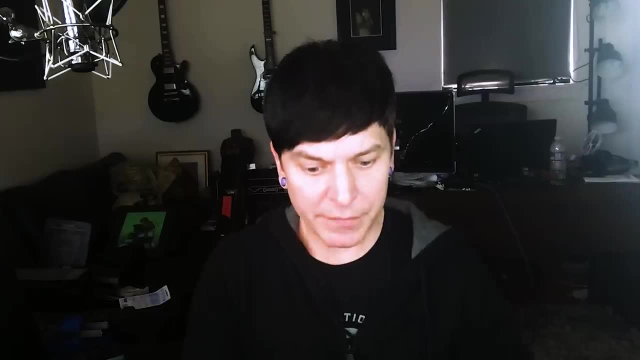 is now. i love, i love how you're explaining those, steven. i mean, i can see number one, that you train a lot of people, and number two, you really understand this because you're explaining it simply even though it's complex. so i appreciate you doing that. yeah, for sure. 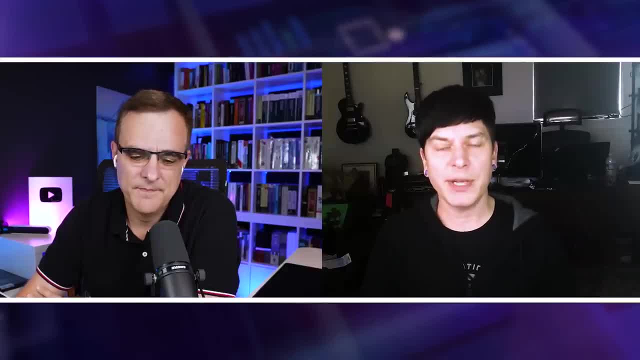 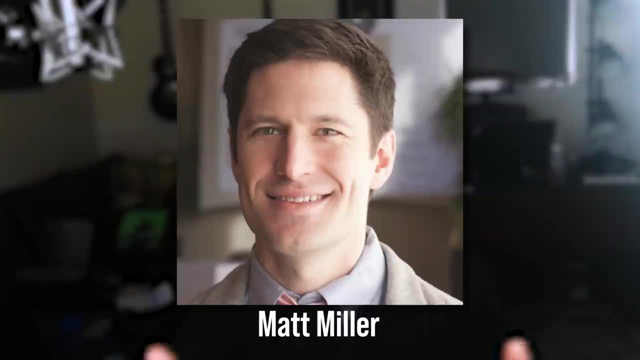 it's. it's a lot of fun, i mean, even though a lot of these vulnerabilities end up getting mitigated. they get patched, of course, but the folks at microsoft, like uh, matt miller, who is the guy who wrote the original meterpreter module, works at microsoft now for a long time. he's one of the 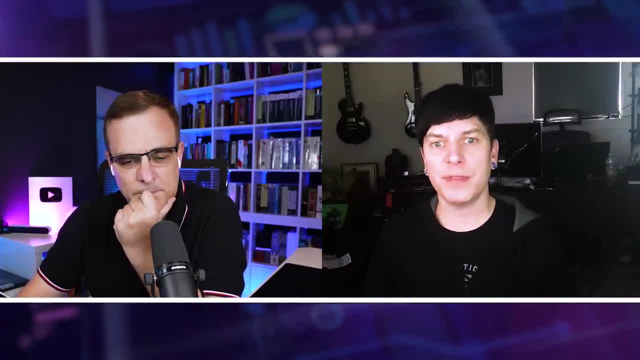 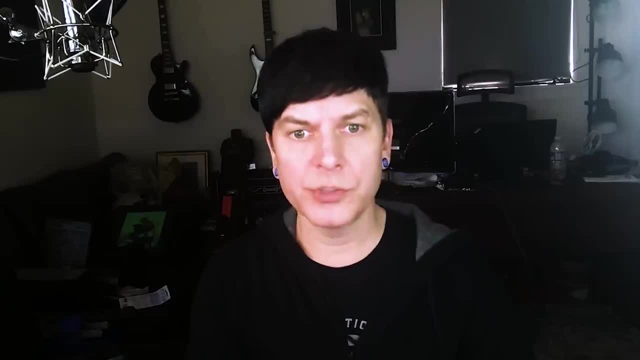 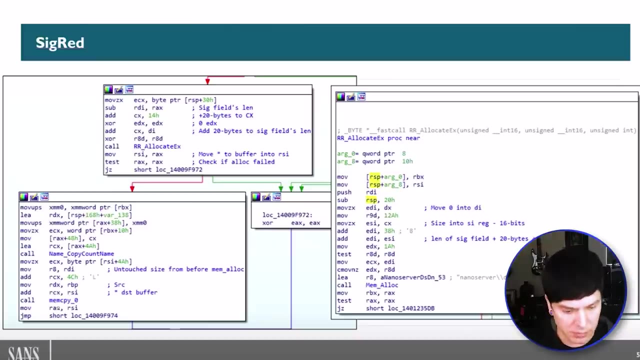 guys responsible for implementing and creating these mitigations that make those types of exploit techniques not possible. what i want to do now, if we have time to do so, is jump over that line and just take a look at what this would look like in the code. it might not let us do it, but we'll give it a shot. all right, so we're in command line. 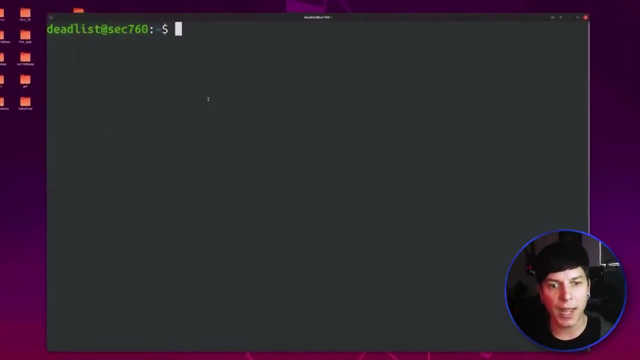 right now i'm on this just ubuntu virtual machine, and what i want to do is try to create a little program and intentionally cause it to have a buffer overflow vulnerability. i'll just go: bull that sounds good, all not see. and then we use vim, and now we're going to go ahead and start. 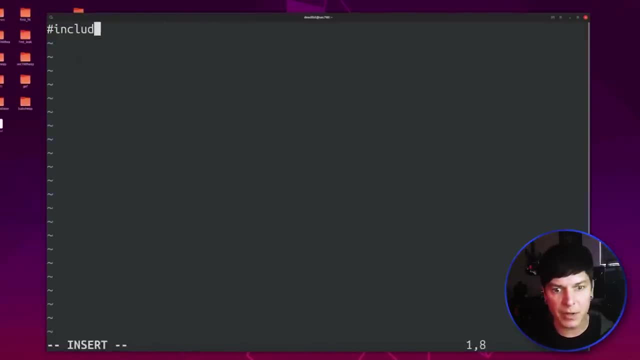 coding it up. so i'm probably going to add more than i need, but i don't want to have to deal with many compiler errors, so we'll just add in the appropriate um support data and then we're going to use std i o and that will include a couple more. i don't know if i'm going to need them or not. 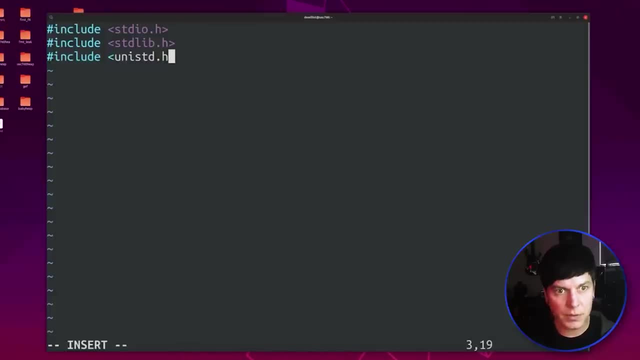 but better to put them in than not standard lib close that out. so these are the headers that i need for this, and then i'm going to create a static password in here. you would never do this in the real world, but define a password and we'll call it password, because that's a great password. 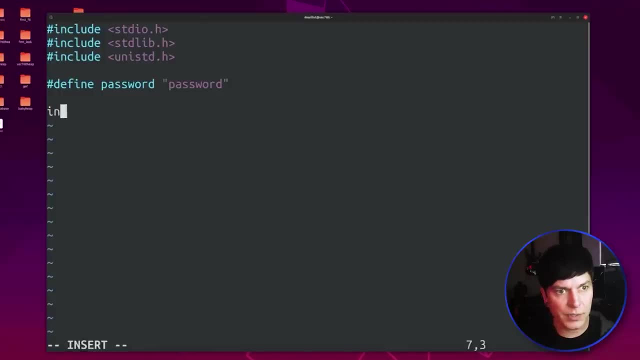 of course, and then i'm going to start with the main function, so int, main and, and so here's where i'm going to do arg c, that's the argument counter, and i talked a lot about this a bit earlier. but and then we'll also do argv. and, if you remember, argc is the counter, argv is the vector and argv. 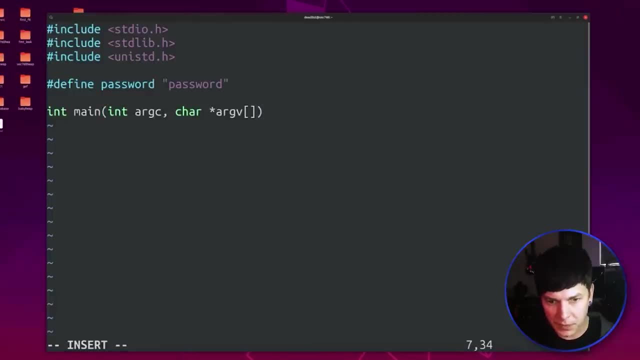 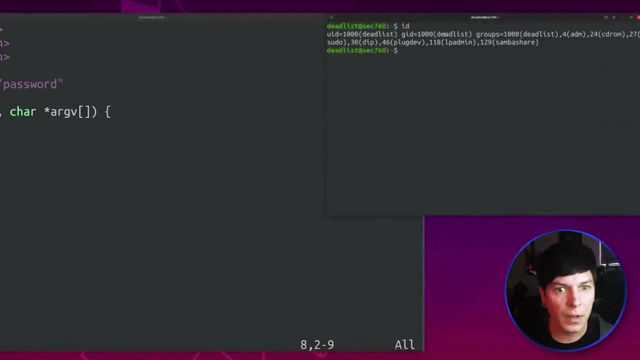 zero is always the program name. so that's what we'll start with there. so let's jump into the main function here. and the main function: I don't know what my id is currently. let me see if I can check that real quick. so my id is 1000. I should have guessed that. all right, so I'm going to say: 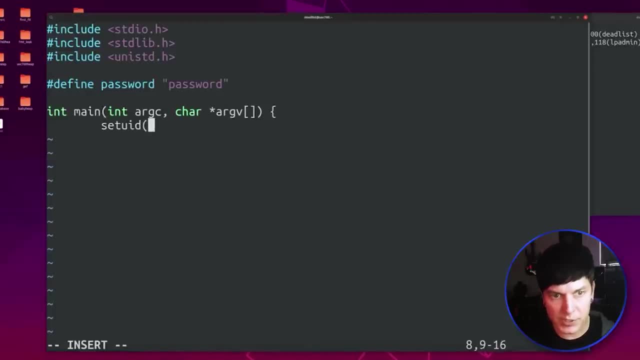 set uid because what happens a lot of times is a process will drop your privileges, so I'm going to set it back. probably don't need this. normally this would be the case if I want to make sure it runs as root, but I'm not going to mess with that right now. so we've got set uid if that works for. 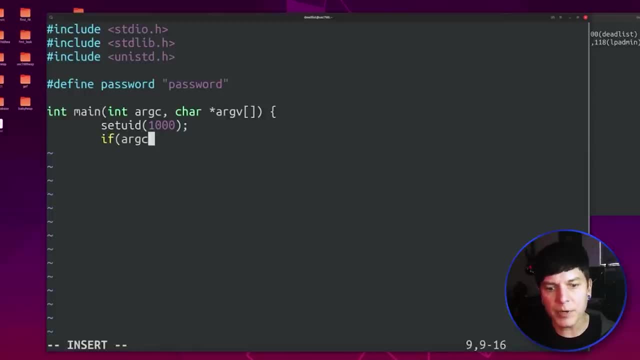 us if, and then I'll say arg. I'm only putting this in to help you understand if you're not familiar with c very well, like the argument vector, because I'm sure you've seen when you run a program, if it wants command line arguments, it yells at you and says, hey, I will mail out arguments, or maybe it. 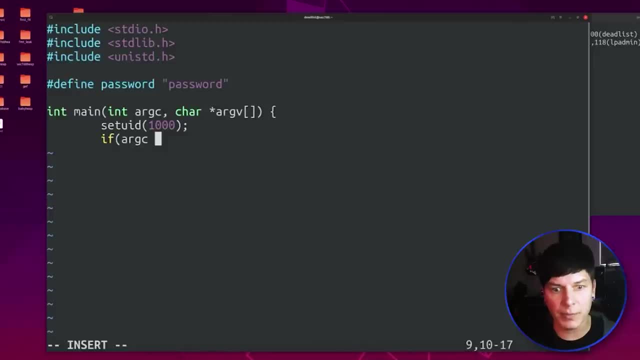 doesn't like command line arguments. so this program I'm going to make it so it doesn't want command line arguments actually. so we'll skip the argument, vector part, but I'll still put it in here. so, char, and what I'm going to do here is say, if the actually that's not what I want, if the argument 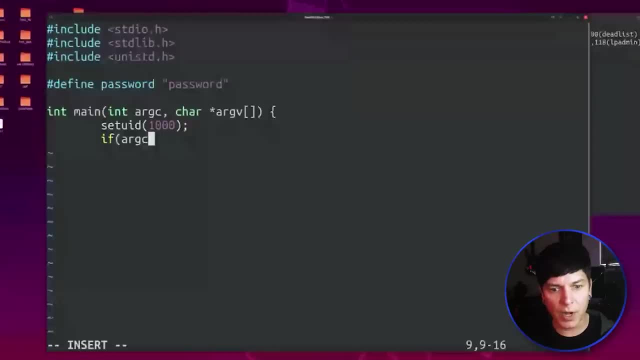 vector is greater than one. so I don't want any arguments in this program. so if the argument counter is greater than one, then I'm just going to give it a usage statement. print f: there is no usage. I'll put that in there. and the reason again I'm putting that in there is because it should help you see, kind of, how the argument. 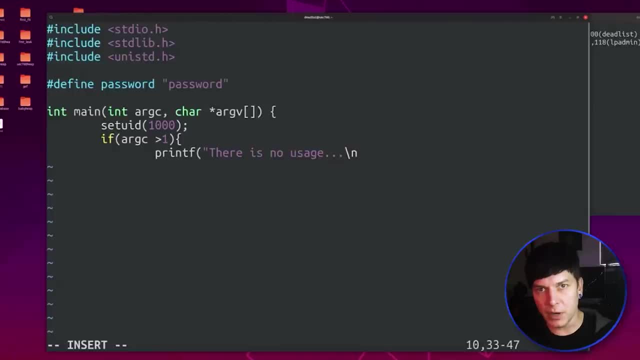 vector encounter works again. argument v0 is the program name. arg v1 would be the argument that you send in, the very first one. I don't want any. so somebody tries to send an argument, I'm going to yell at them and say, hey, there's no usage. not terribly exciting. I mean you're keeping it simple. 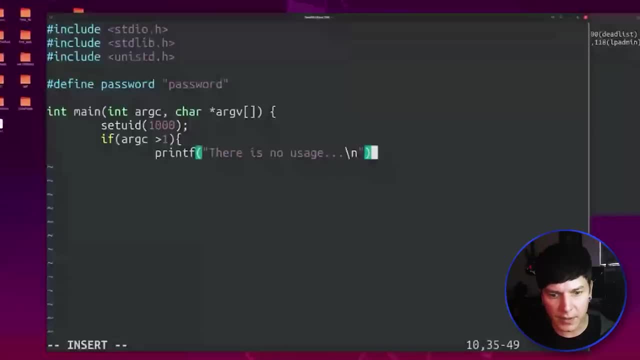 which is great, yeah, so all right, we've got that knocked out, and then we'll just say: if that happens, we'll exit with a one meaning an error and we'll close out. so that's a little check and a check to see if you have it in an argument. and now I'm just going to call the vulnerable function. 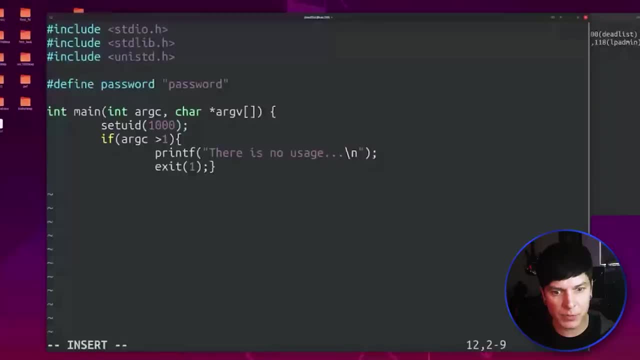 or the function with the vulnerability that haven't created yet. I'm going to call it check password, check pw, and it doesn't want any arguments, return zero if we don't have any issues and then close out. next, we got to create the vulnerable issue, the vulnerability, so I'm going 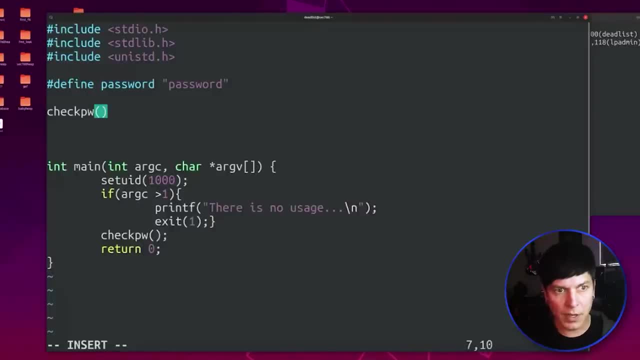 to create a function called check pw and then when we go into this function it's going to say print f, please enter the password. we'll say yes, this is the vulnerability. I'm using the gets function. you should never use that function because it doesn't have a size. 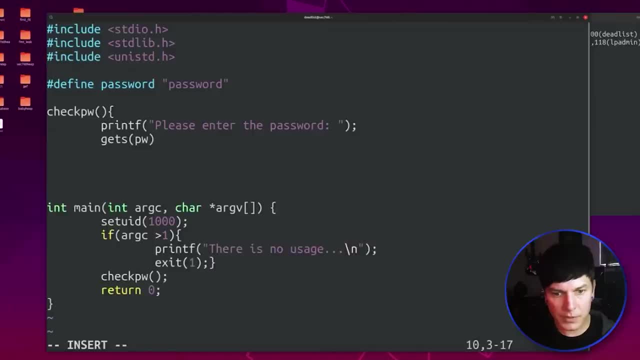 argument. so I'm saying gets pw. and then inside of here we're going to say if string compare, password is password, then call the grab the function. and we haven't created that function yet. else we're going to say print print after access denied. I'll close that out. let me just think here. 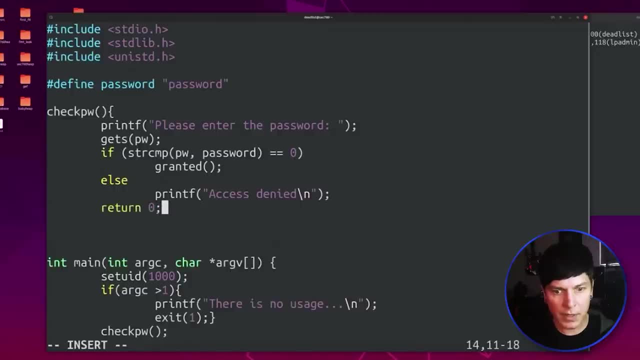 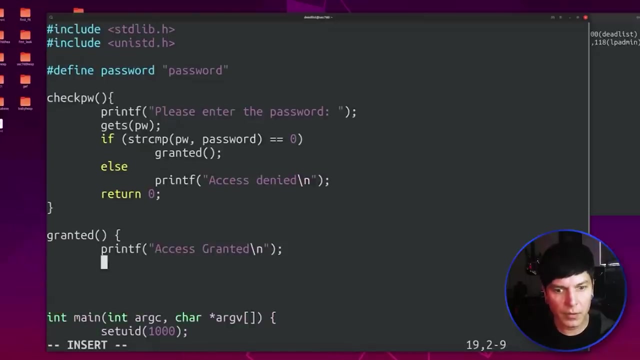 real quick. you know, return zero and then close this function out. we need one more function called granted, and this function will simply say: print f, if you reach it, then print f, access granted, and then return zero, close that out, and that should be our whole, our whole program. so if we walk through that again, 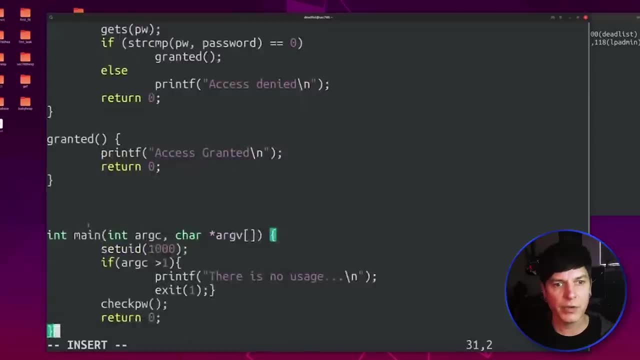 we've got the main function is the first thing that I'll execute. it tries to set the uad back to 1000, which should be fine, and then it says: if the argument counter is greater than one, meaning if someone entered in any argument, print out a message that says there's no usage. 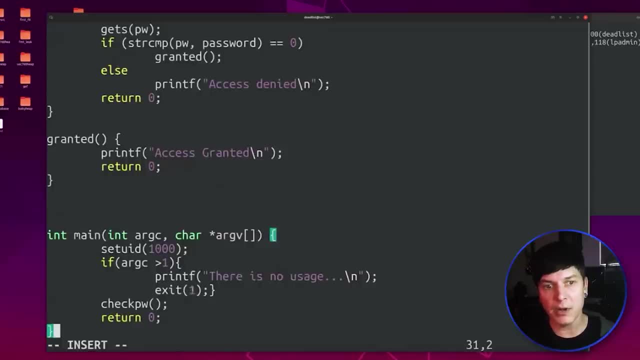 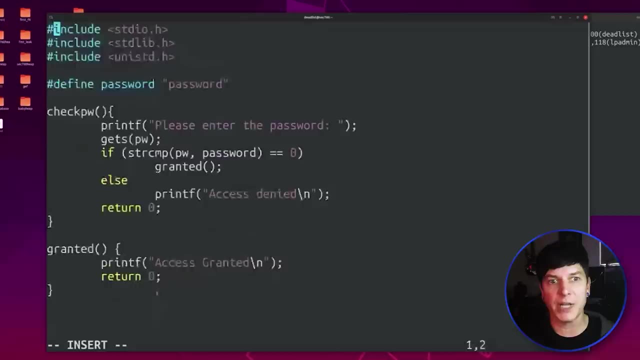 and exit out with an error of one. zero would be no error, one is an error as a status code. well, if there is no arguments, call the check pw function. the check pw function says please enter a password, gets pw. so it's going to prompt us for standard input to enter in a password. 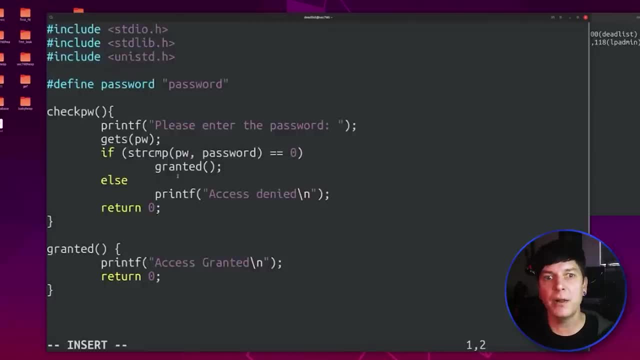 it comes in. it says: go ahead and compare the password, which is basically just a string password, against what we sent in. if it's zero, meaning they were equal. if they met, then call the access granted function. that will print up access granted. otherwise print access denied and return out. it's a pretty simple little program but it's got a buffer overflow because 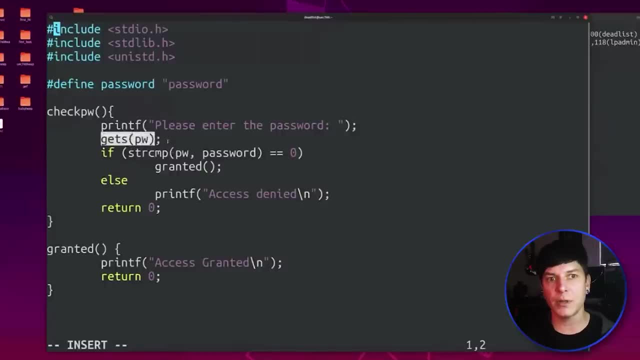 this guy here doesn't have a size argument, so I've only allocated a very small buffer. have I even done that yet? let me see here: nope, I forgot to do that. right, I went through that and actually read through that, because it wouldn't have worked. I love it when master- people like yourself make. 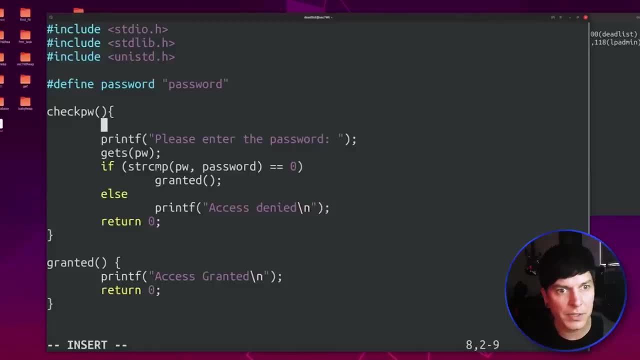 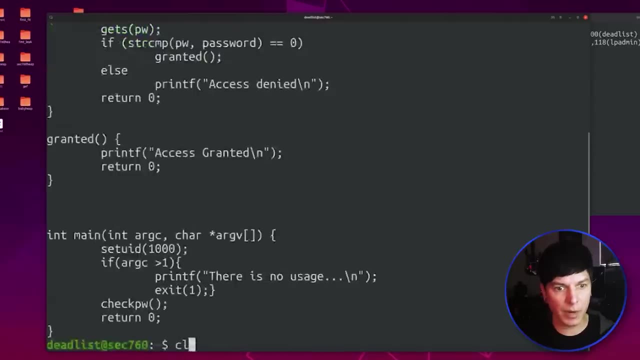 mistakes. it's encouraging for the rest of us, especially in very basic things like this character pw. we're going to make it a hundred byte buffer. all right, that should be good, all right. so there's a little program. let's see if we can get it to compile. now. that's going to be the question. it might block us, but we'll try. 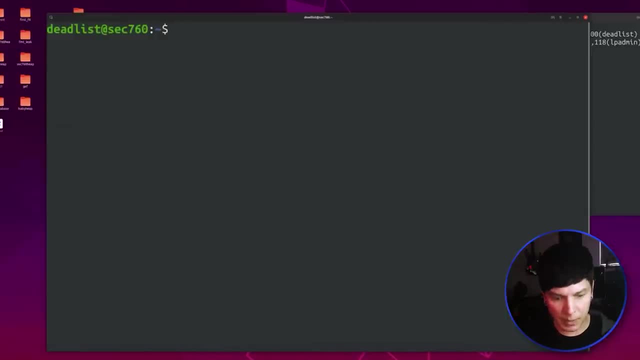 all right, let's do. uh, I'm going to make it just a 32-bit executable right now. to keep things simple: gcc minus m32. now I'm going to put in some mitigation. uh, m32 means compile as a 32-bit binary. but I'm going to. I'm going to kill some mitigations that would otherwise be automatically. 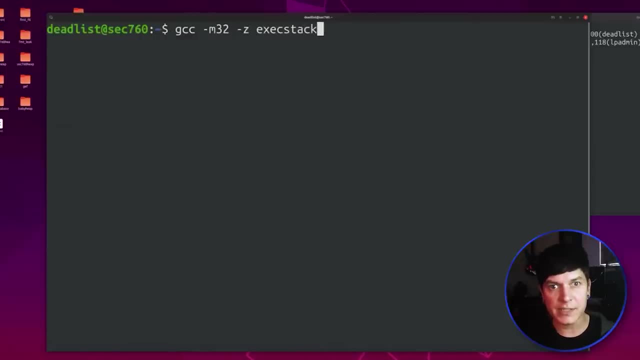 added in. so I'm going to say minus z is exec stack, which turns off depth, and then also minus fno stack protector. I think that's what it needs to be. that says turn off stack canaries, and then the program name is volumec. we'll just 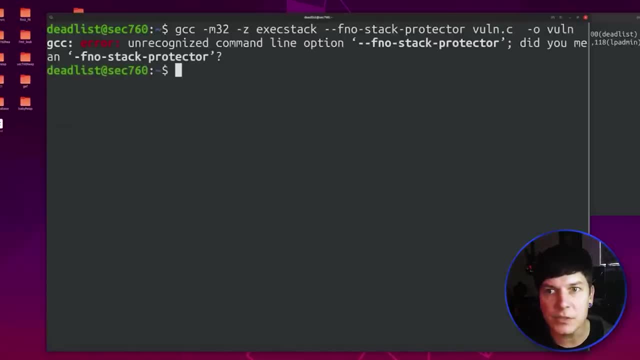 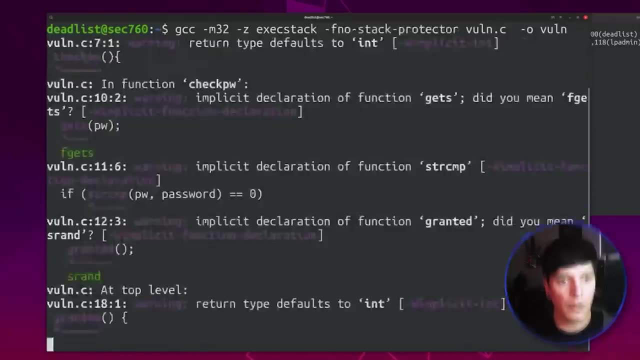 call it volume. it's going to yell at us. it says it doesn't. did you mean fno stack? oh, I put in one extra um hyphen. all right, did it compile. so it's going to yell at us. it's going to yell at us, it's. 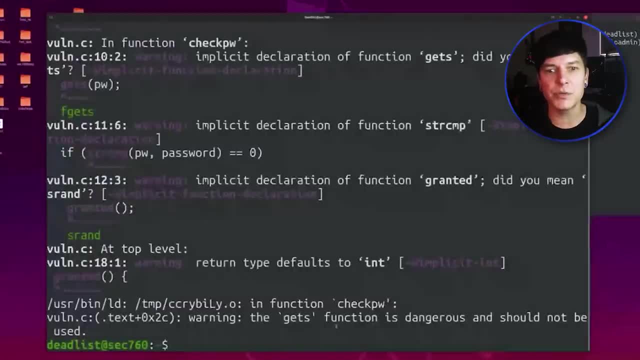 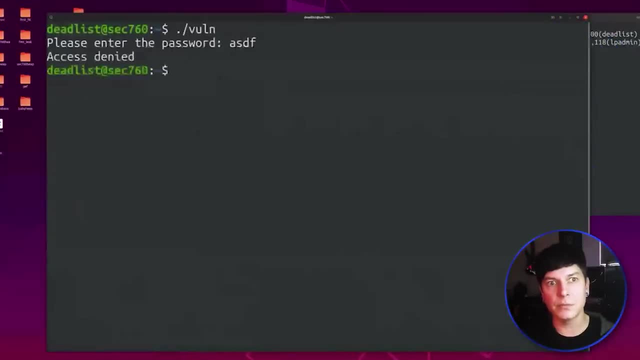 yelling at us. it says there at the bottom: the guest function is bad, don't use it. well, we just ignored that. it filed us in. let's see if it, if it actually compiled and it did so- works as expected. now we know there's a vulnerability like so to show you that argument vector thing, if I try to 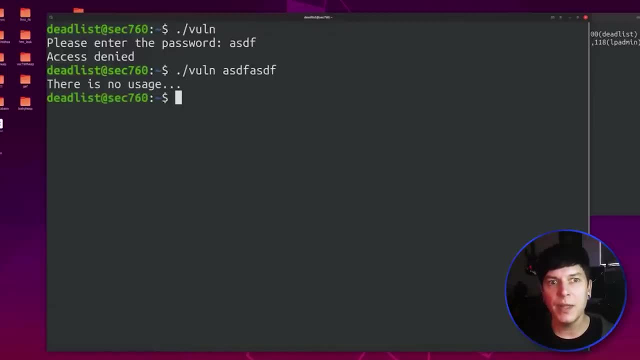 enter an argument, it's saying there's no usage. because I enter that in and if you look at the disassembly it's really easy to to spot that and you know exactly where you are in the code, because it's doing a little check. now we know there's a hundred byte buffer, so here's something cool. I 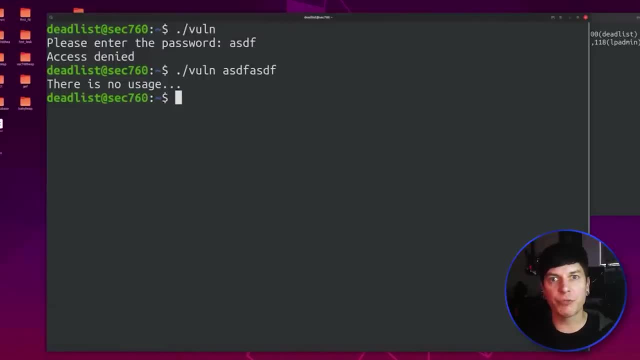 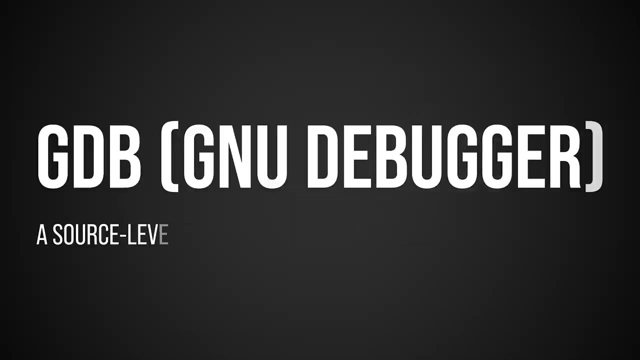 show you, which is how can you determine the buffer size through reverse engineering, as opposed to just cramming in a bunch of data with a pattern or something like that. so what we could do is go gdb. gdb is the gnu debugger and it's a debugger that supports fortran c and c plus plus. 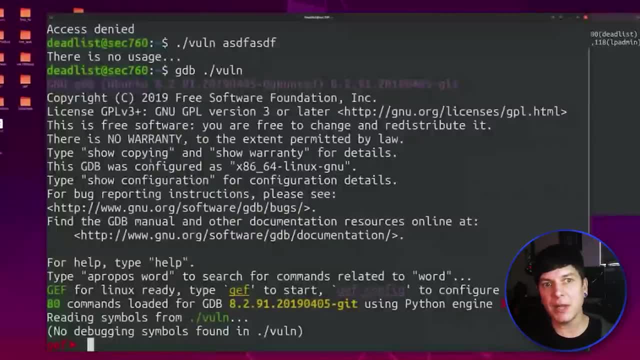 written by Richard Stallman many, many decades ago. it's a command line debugger that's not very friendly or intuitive, but there are things to help. you can get a front end to it, like a graphical front end with ddd or edb. but uh, we're using an extension called 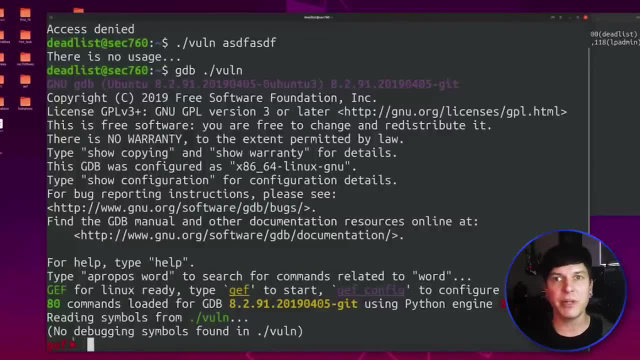 jeff, g, e, f. you can see down at the bottom. that's a exploit development assistant tool that has a bunch of functionality that comes along with it, imports it into the debugger so we can take advantage of it. so I'm just going to say, disassemble me now, defaulting to something. 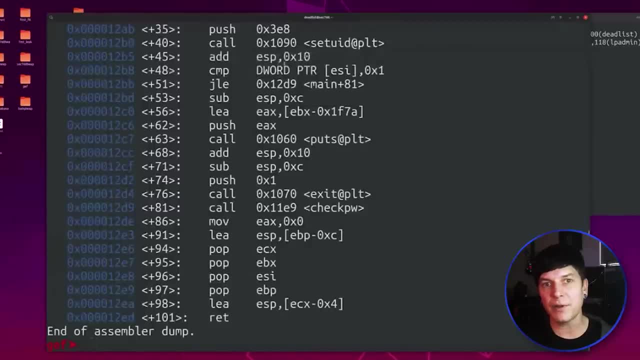 called the intel disassembly syntax. gdb by default uses what's called at&t syntax, basically swaps the operand position and does some other things, but it doesn't really affect the program or the behavior. it's just, uh, how you, as the person reversing, would like to see the disassembly displayed, nothing more than that. so by looking in this, 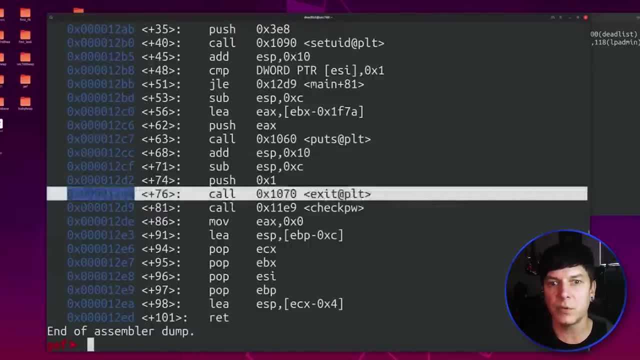 disassembly. some things stick out like right there, exit. well, we know the exit function does and we even put that in there. we said return zero and exit uh puts. that's the put string function. it just prints to the screen. so some things stick out pretty uh quickly as you're looking in here. 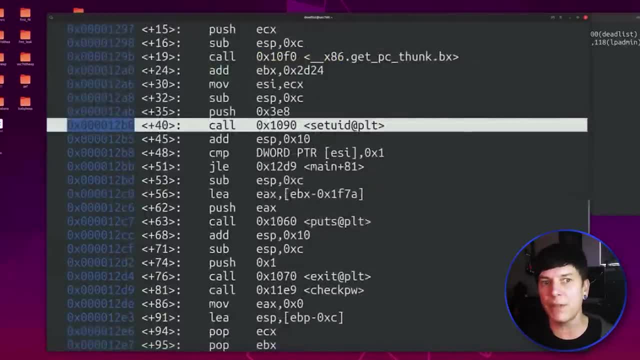 there's that set uid, remember we tried to set the id to 1000, so this 3e8 is very likely 1000 in hexadecimal, being pushed onto the stack as an argument to the set uid function. now this function check pw. we know that that's the one that's got the 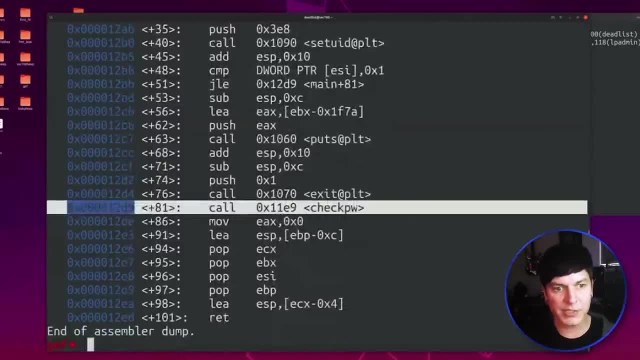 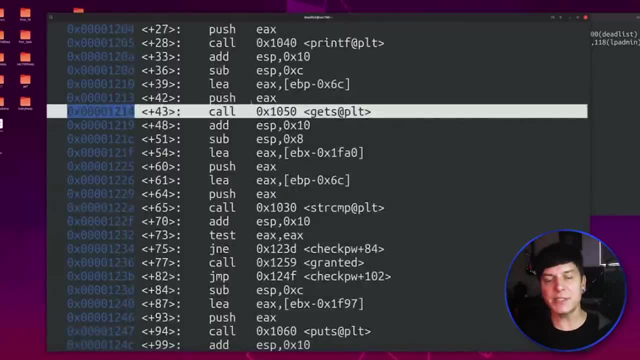 vulnerability in it because that's where I put the gets function call. so if we say disassemble, check pw, when we scroll up here there's that call to gets right above it. so gets needs the destination address where it's supposed to write the data that we're going to type in. it needs to. 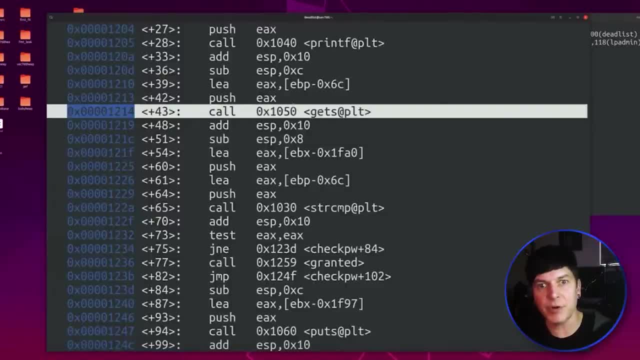 know where to write it, so we have to give that to the gets function as an argument. this is how this. right here it says evp minus 6c. that ends up being offer size because the evp is the extended base pointer. that's a stack register and basically, by what it's saying, there is take the address. 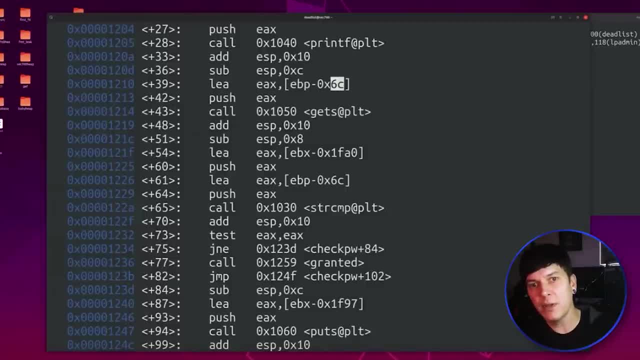 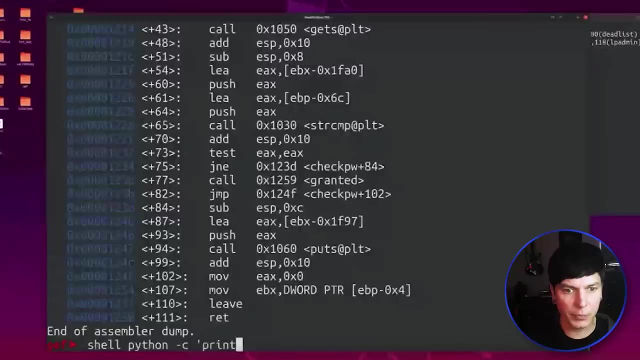 of the base pointer. that points to the base of the stack frame minus the buffer size, and that's how it tells the gets function where to write the data. but for us it tells us the buffer size. so we could real quickly say something like shell python minus c, and then I'll just say: print: and what was that size? again, that was 6c, right, so print. 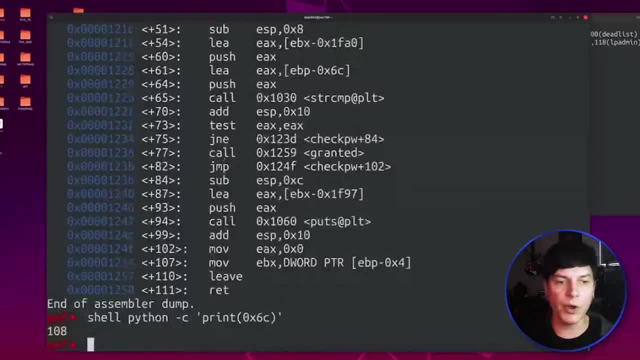 euro x 6c, and let me close that out- and it says 108. so, if you remember, the buffer size that we created was a hundred bytes, right? so there are other things that might be playing a role here making it a little bit bigger, but the point is that shows us about how much, how many bytes we 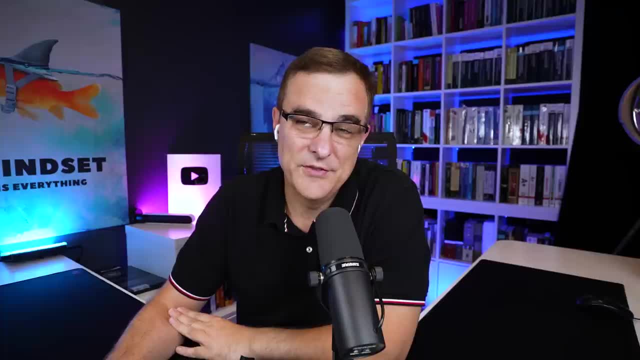 want to send in as an attacker to overrun that buffer. I'll just. I just want to interrupt you and say I love it. I love I love that because all the demonstrations I've seen is people are just stuffing it until they somehow get an overrun right, which is great. I mean you can use the pattern tool where you create a. 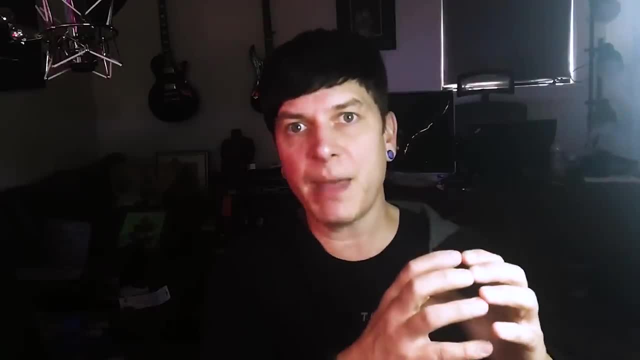 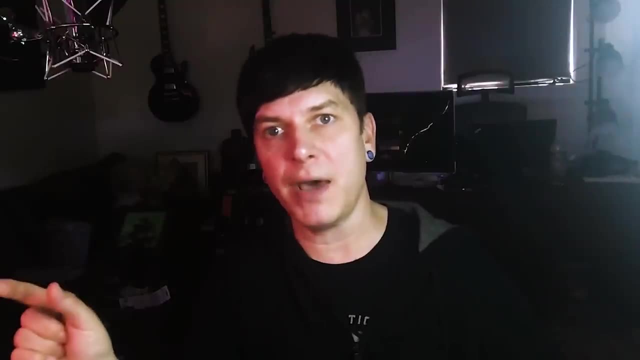 pattern and then you call it the process to crash and then a piece of that pattern shows up in the register and then you can ask the tool, how many bytes into the pattern was this piece of the pattern? and it shows you how, like that's the buffer size basically. but this is the you know. 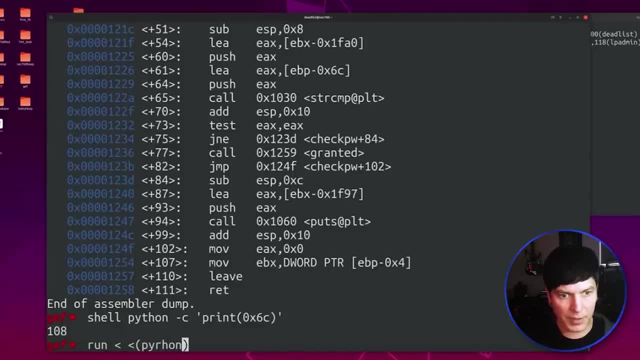 more elegant way of doing it, I guess. so we're going to say: run python minus c, print a times. I'm going to put 100 to 100 days, plus I'm going to put in me bbb plus cccc plus bddd and the reason. 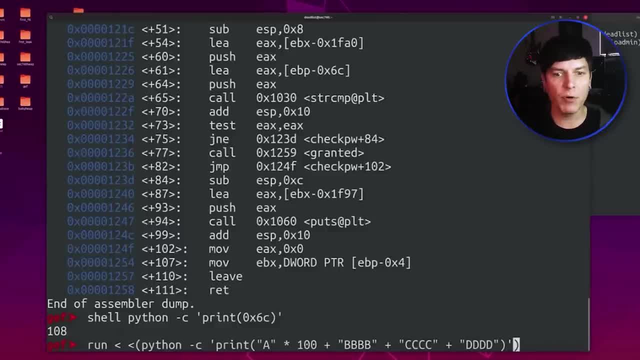 I'm doing this is because we know that if we see 41414141, that that's a's. if we see 42424242, that's b's. if we see four, threes, that c's you get. you get where I'm going, so I'm going to run this. 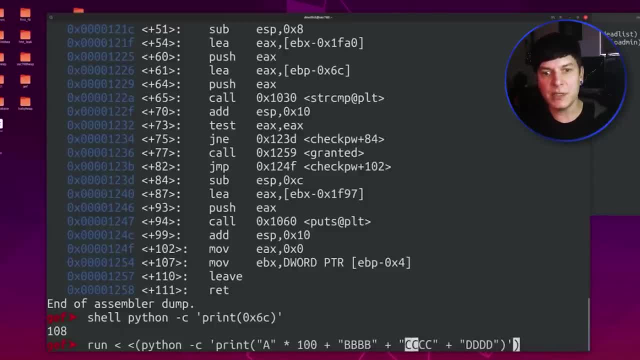 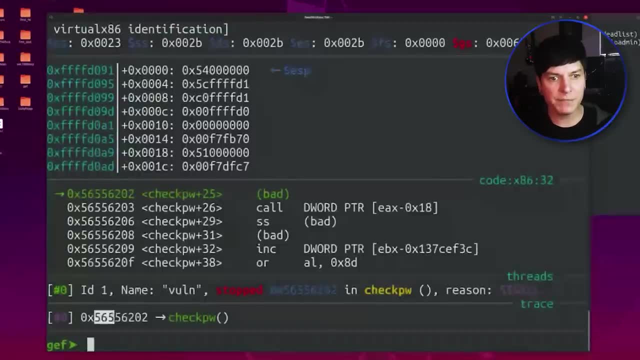 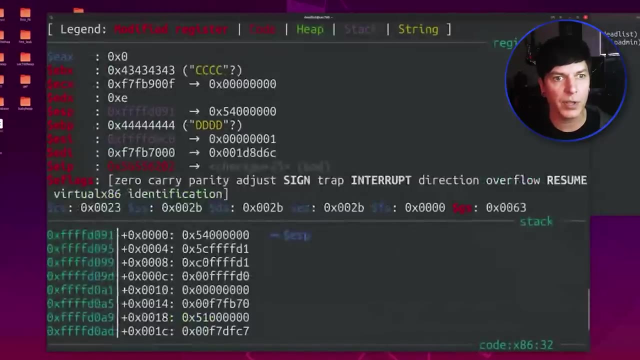 what I'm hoping for is that it crashes and we see some of those values appearing in the register to help us. let's see what happens. so right here it says five, six, five, five, six, two, zero two. and we're at this interesting memory address. something's obviously went wrong here, you can see. 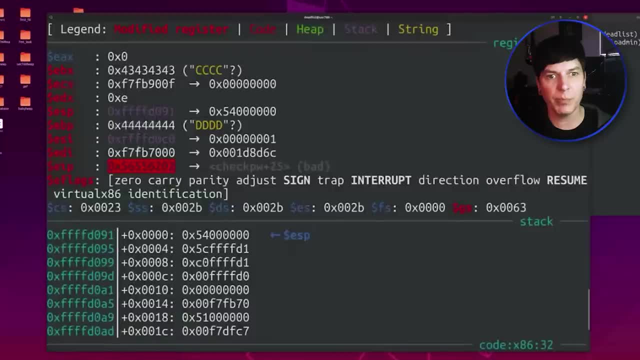 that the base pointer points to dddd, the instruction pointer points to this strange address. so what this is telling me is that I'm not seeing four one, four one or four two, four two or four three or showing up in the instruction pointer. because the instruction. but if I successfully overwrite 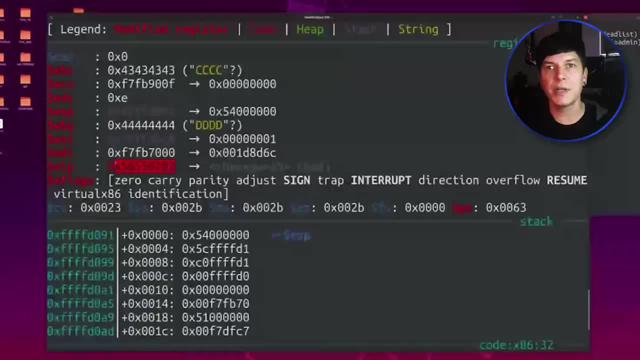 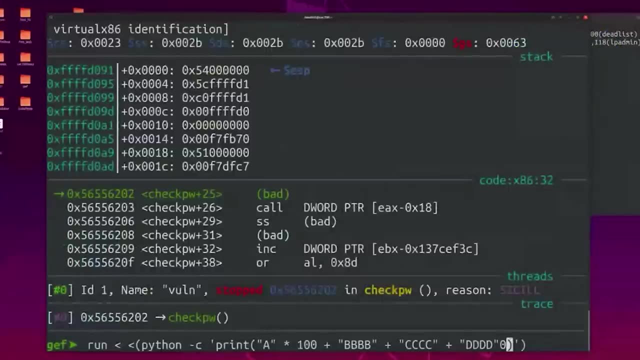 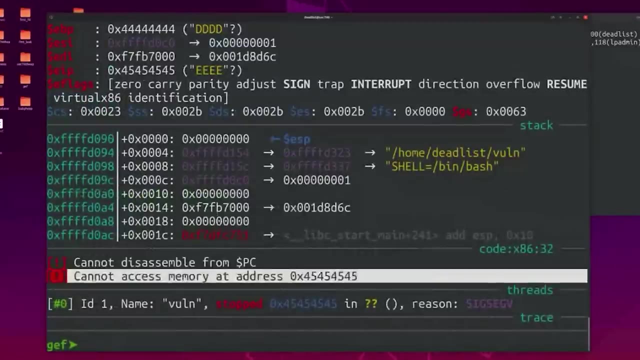 that return pointer, then the instruction pointer should be pointing to those values, because it tried to return to that as an address. so I'm going to run this again, but actually send in four more bytes. so plus eee. run this again and now look what it says. cannot access memory at. 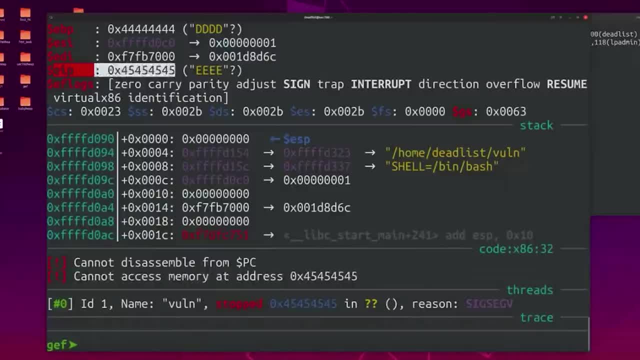 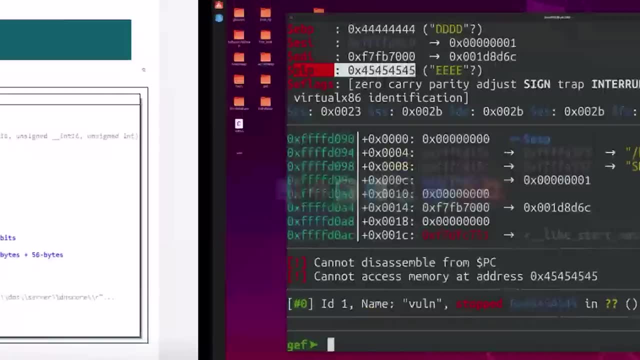 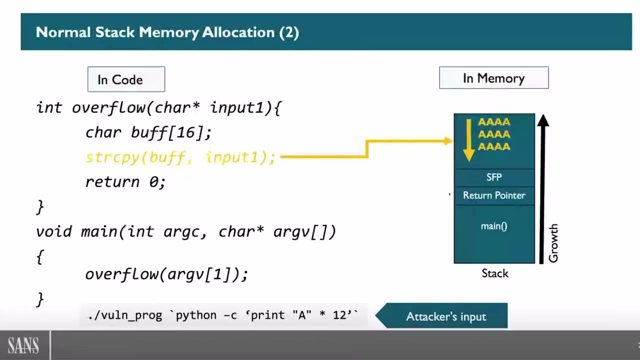 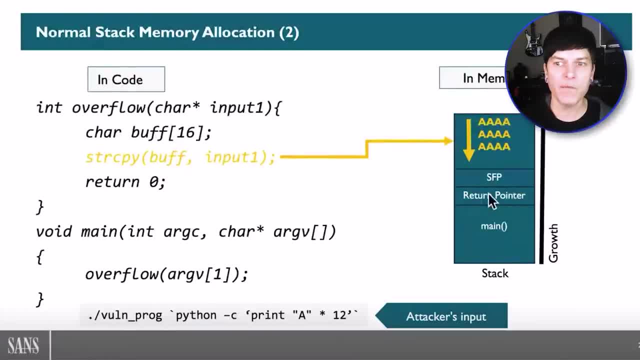 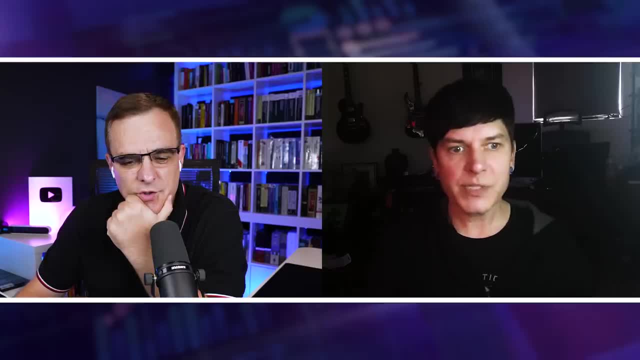 so by cramming in enough data, we eventually were able to overwrite it with our ease. so now we have control of the process. we can tell it to go wherever we want it to go. this ends up. you get it to run a shell. sorry, right, yeah, we should be able to get it to run a shell if I had shell code. 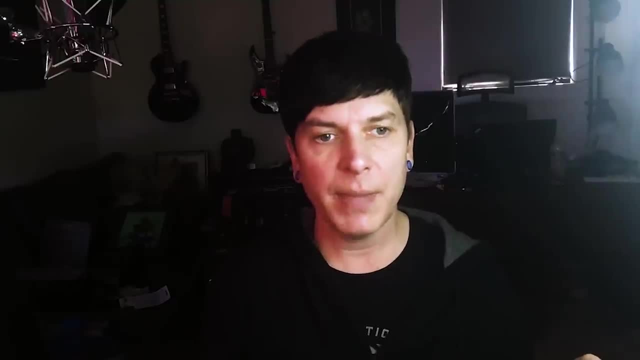 or something like that. what I'm going to try and do is see, if it lets me, is maybe I can return back to the access granted function somewhere. I'm not supposed to be able to return to bypass authentication. the issue is I didn't compile this as a position, independent executable. it's got ASLR. 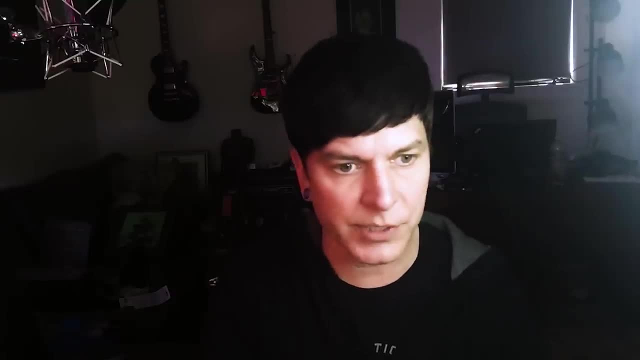 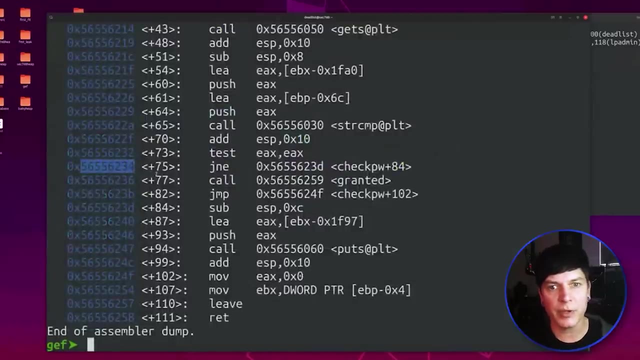 on. so it might not let us do this, but we'll give it a shot. we'll see what happens here if I disassemble check pw. so these addresses should be rather consistent. what I want to do is overwrite that return pointer with this address here so that when it returns, it returns to the 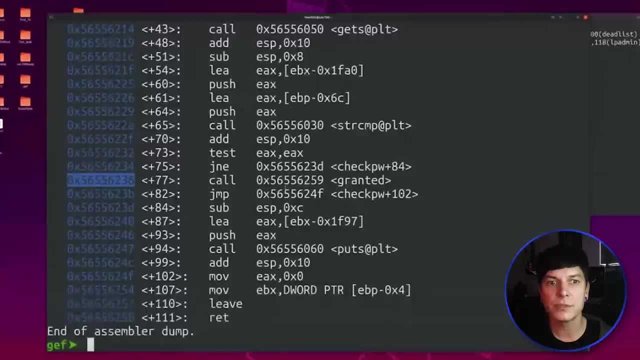 call to the granted function allowing me to bypass authentication. see how that would work. so let's see if we can get it to work, though I'm going to take my input here. so, instead of eee, in a little Indian format, because x86 is little Indian architecture, which means it writes the bytes in. 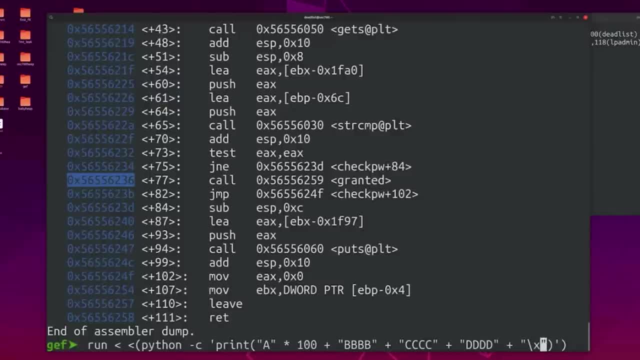 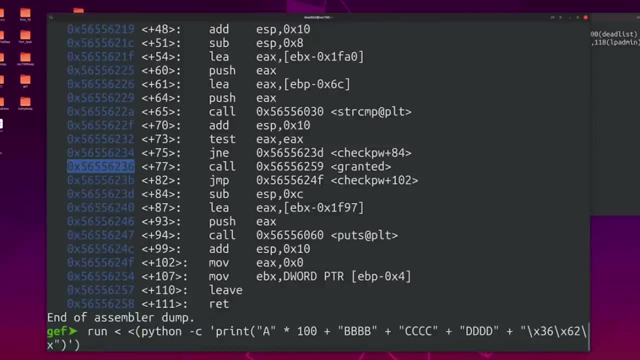 reverse order in memory, so we have to write the address in backwards so that it actually writes in forwards in the right order. so three, six, slash x, six, two, slash x and slash x. by the way, if you ever see, that means base 16, hexadecimal five, five. 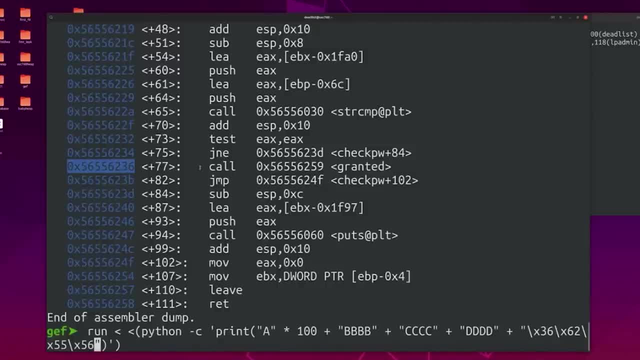 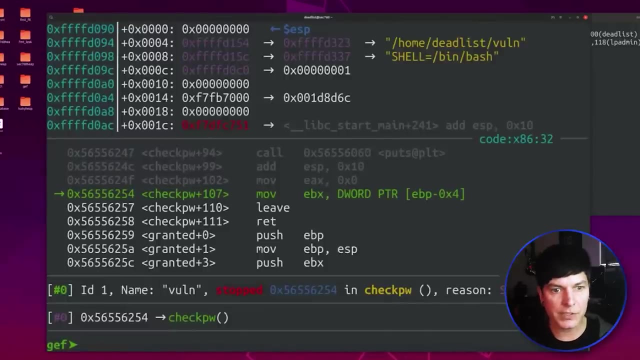 slash x, five, six. so I've now written that address that I have highlighted in a little Indian format that will overwrite this position here, where it says: return pointer. if it works, we'll return to the granted function called bypassing authentication. so let's see what happens here. I'm going to let it go. and it says: stopped check pw- segfault. but we're in the check. 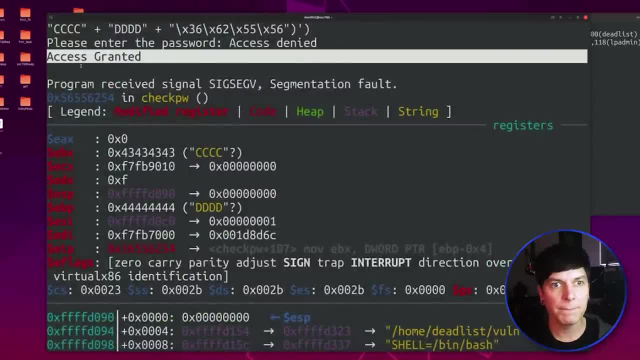 pw function. so if I go up top here, look at that access granted so we successfully bypass authentication. now we we could have done that if we had done that. we could have done that if we had overridden that with uh, a call to a function or something like that. like that's one cool technique. 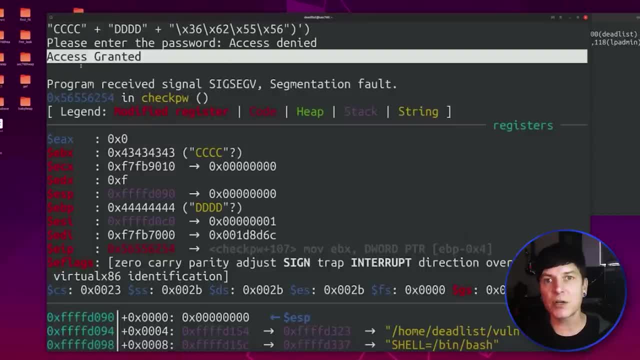 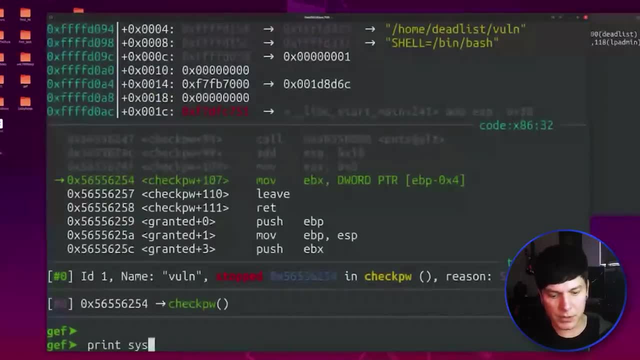 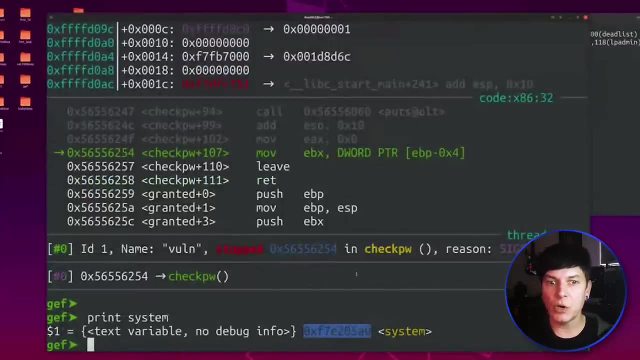 to get around asl- I mean data execution prevention- there's a technique called return to libc. it's an older technique but it works quite well where, if inside the debugger we say print, uh, let's see here how about we print system? what this is showing us is the address of the system function. so, if I can, 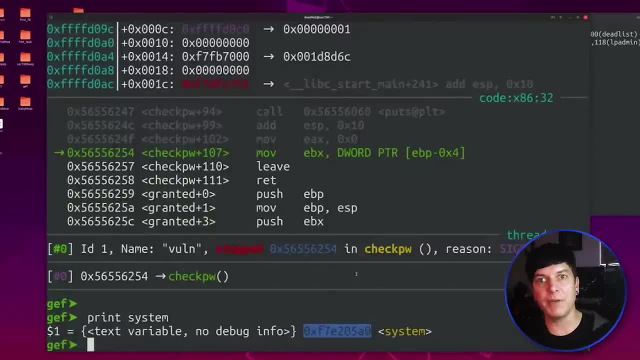 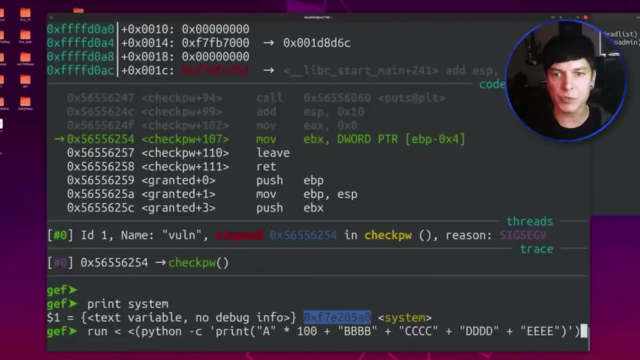 return to the system function. I might be able to pass it something like an environment variable, sh, something like that. there might be some cool opportunities there. so we have a lot of options, which is nice. well, one thing I just noticed here is: I don't know why this shell is here. this: 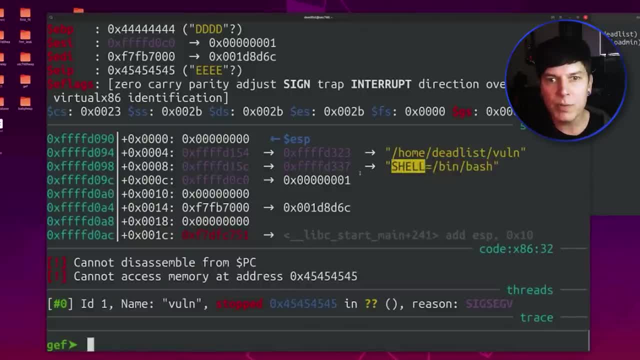 environment variable is in there, but this says shell equals bin bash, so we might be able to return to that address. if we return to system and pass it the argument of bin bash, it might pop a shell, which would be interesting. let me see if I can print that string out in memory, though, so I'm 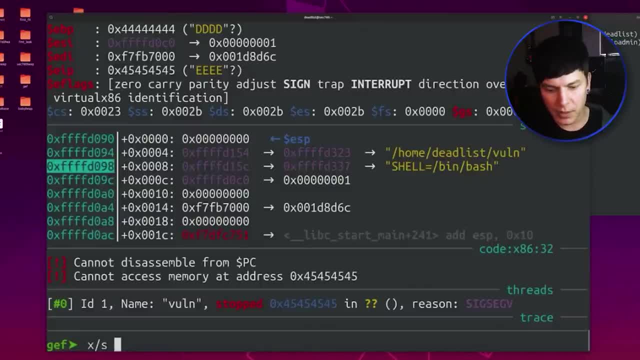 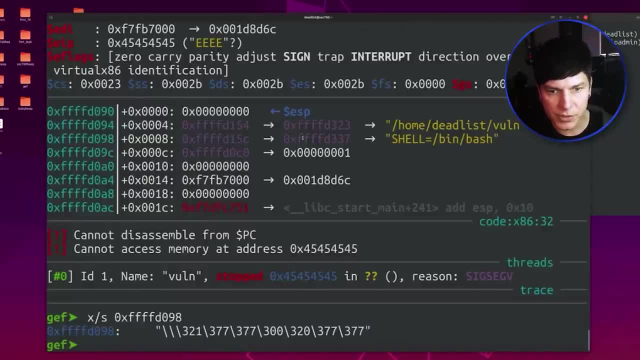 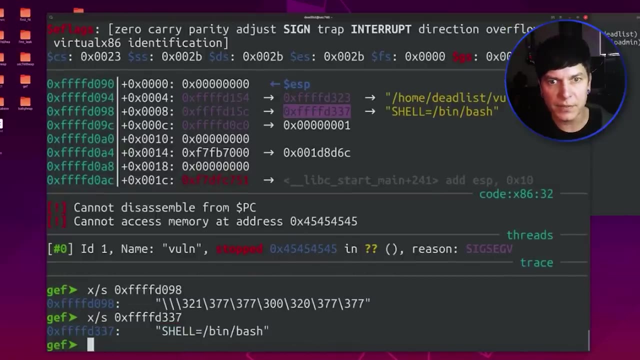 going to say x slash s. it says examine as a string, and then I'm going to give it a memory address. so that's showing us not what I was hoping to see. let's try this address here, though. so x slash s, examine as a string: fff- d337. so shell equals bin bash. so we need to go a little forward here. how. 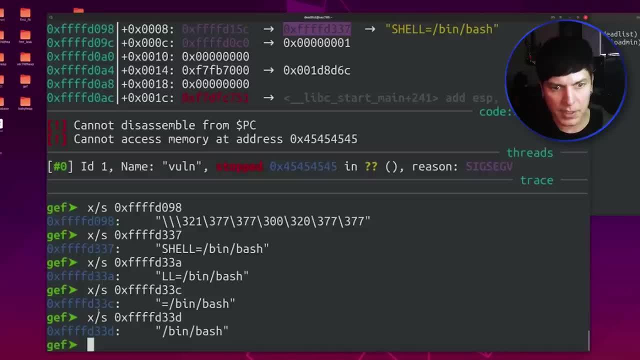 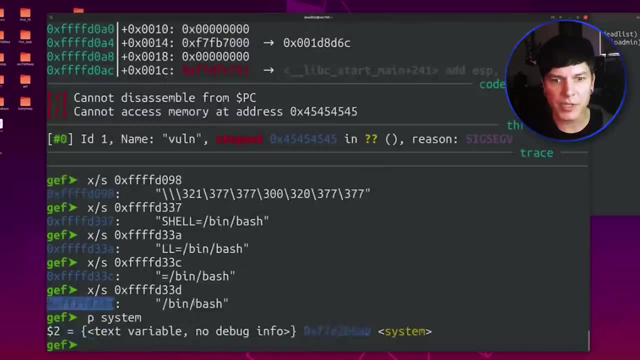 about 3a, ll? how about 3c, 3d? so bin bash is at this memory address. so if we overwrite the return pointer with the address of system and pass it this address as an argument, it might pop a shell, it might not, but we're going to be able to return to the system and pass it this address as an. 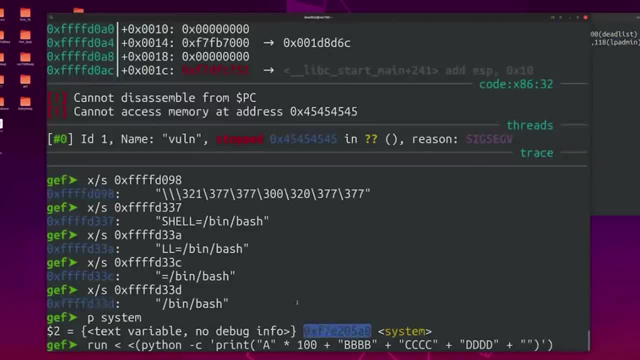 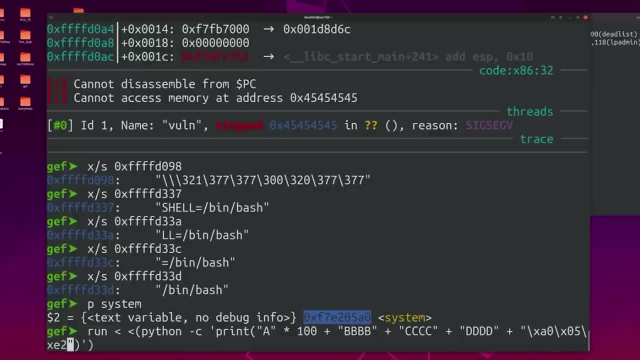 argument. we're going to try it, because- why not? so let's overwrite the return pointer of the address of system, which I'll highlight real quick: it's that guy. so hex, a0, hex, 05, e2, f7, and then a four byte pad and then, finally, the address of the shell. so why a four byte pad? because I know. 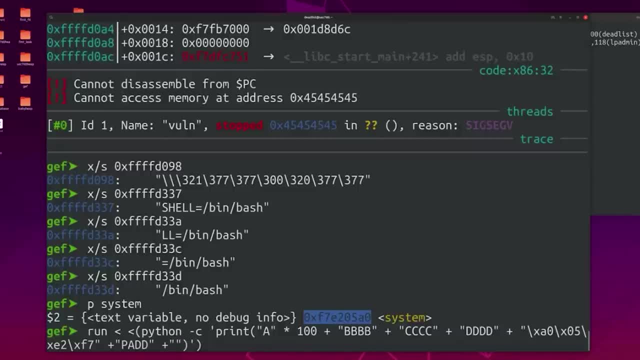 someone's going to ask: we are returning to the system function. that is not how you call a function. you don't return to it, you call it. remember the first thing to call instruction does: it pushes the return pointer onto the stack. so this pad that I'm putting there is literally. 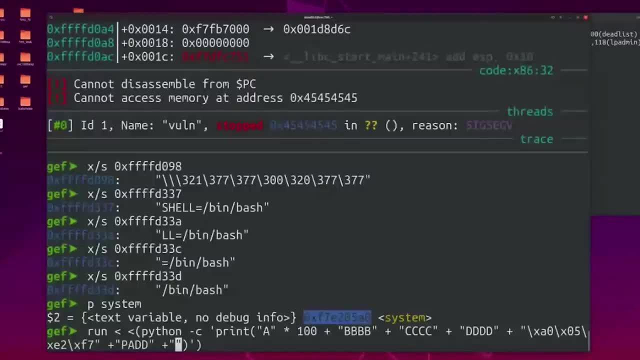 where system will return to when it gets done executing my, my command. so that's it's expecting the return pointer to be at that position in memory. so we're just putting padd. it'll crash, but hopefully it'll pop my shell first. so let's see if we can make that work. I'm going to put 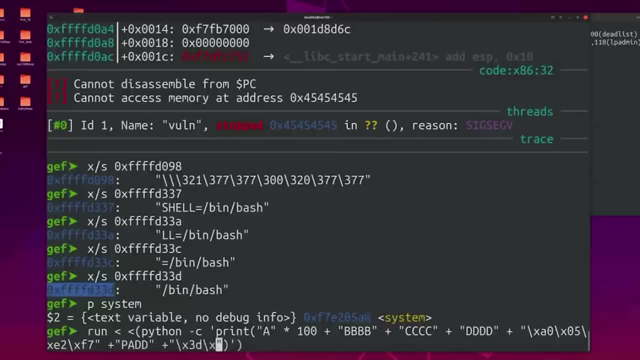 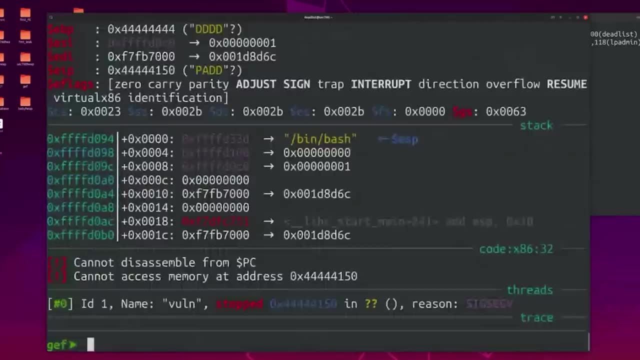 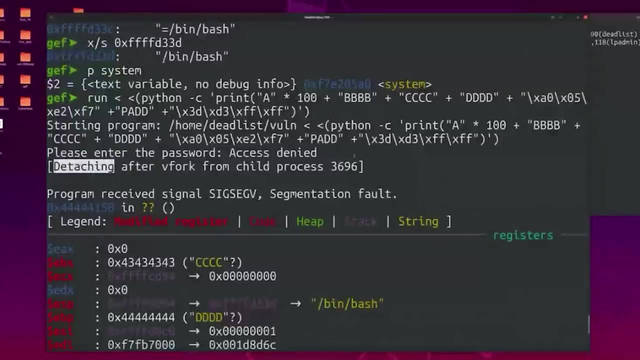 in this address now, which is the address of the bin bash. so 3d, b3, fff, and let's our fingers and a seg faulted. I don't know if I got a shell or not. oh yeah, we did look. see that detaching after v4 from shell process. so it did pop a shell, just didn't follow the fork. 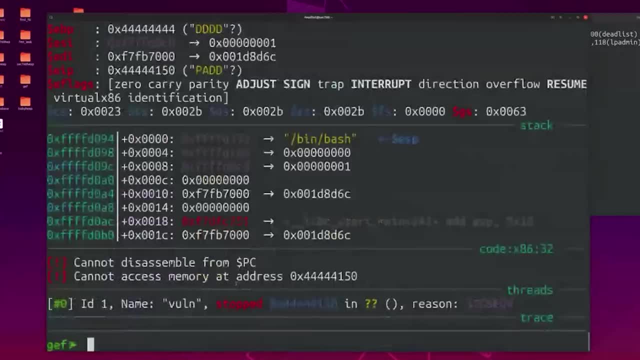 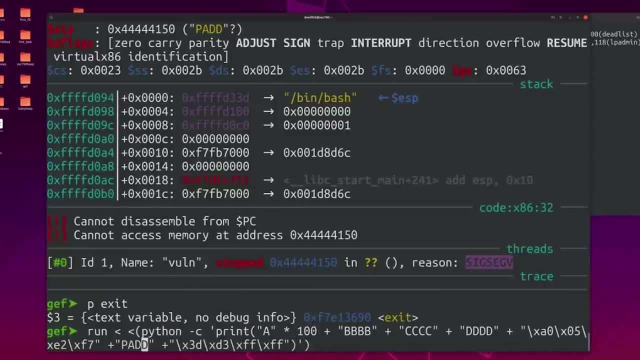 so that's pretty cool. it did actually pop the shell, but here the thing is, it still crashed though, didn't it? let's fix that so it doesn't crash. and it crashes, gracefully: print the address of the exit function. so instead of the pad, I'm going to put the address of the exit function. 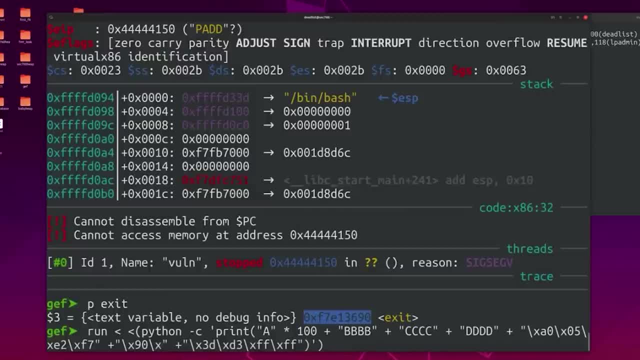 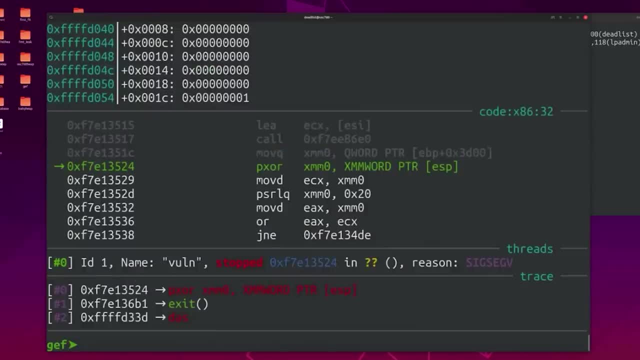 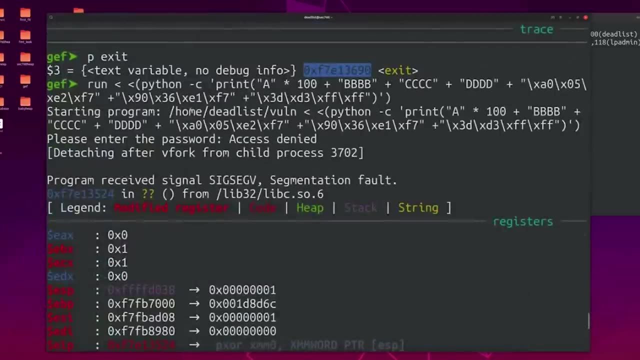 you know that we would see with d message. so now I'm going to put this address in and we'll say hex, nine zero three, six e, one f, seven. now when I run it I'm hoping it doesn't crash. it's still safe, all did. no, it did crash anyway. I wonder why it did that. trap adjust, sign trap interrupt. 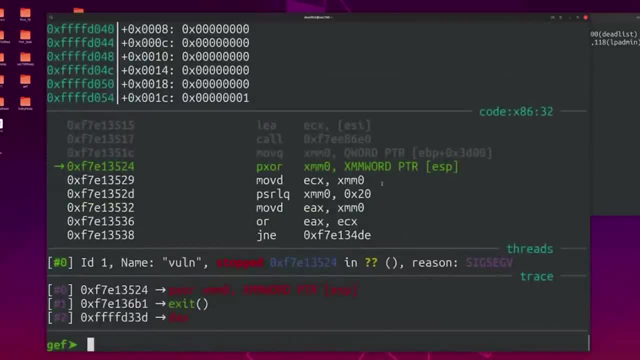 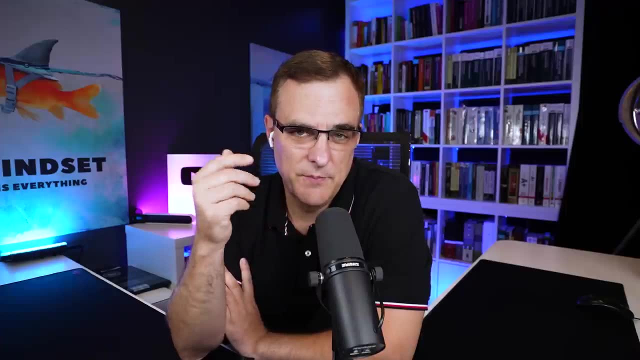 direction soon. virtual still did the fork, but for whatever reason, I think it's because we're in the debugger, but normally that would let us exit out cleanly, so you would have popped a shell. yeah, that, totally that's. it's just not following a fork. I'll try it outside the debugger real. 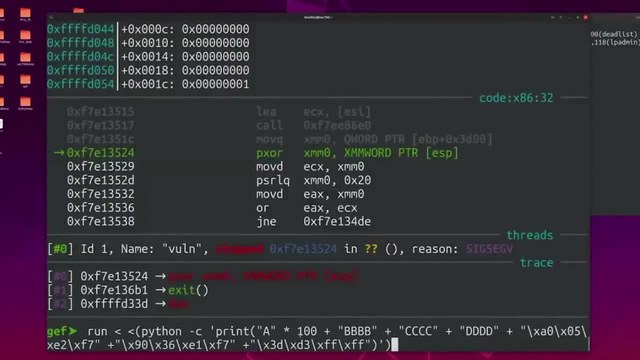 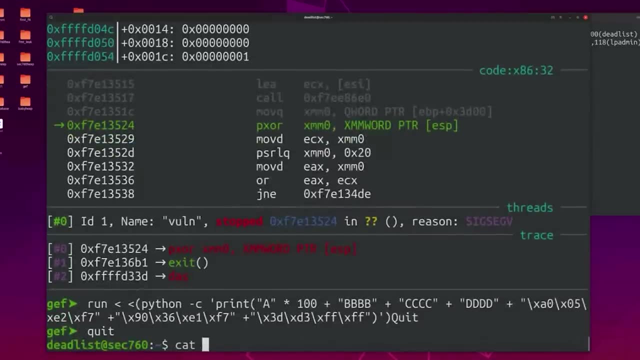 quickly, but aslr is on, so I don't know if it's going to work, but it's okay, we'll give it a shot. let's copy this. why isn't it? let me copy that. maybe it did. all right, let's so what? I just looked. 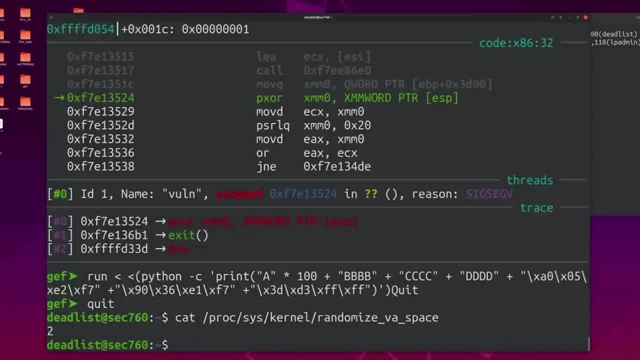 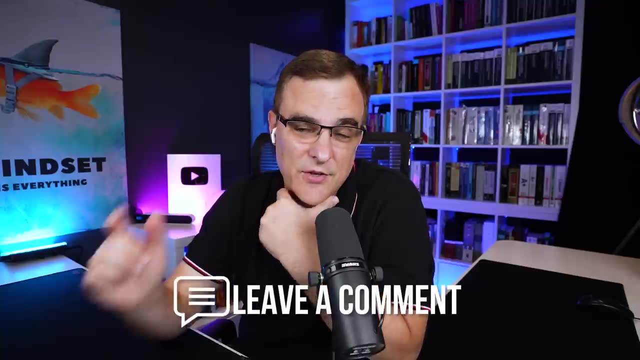 at there is randomized va space. that's the setting for aslr. I'm going to try and turn that off right now, since we're not going through a- just you know, defeating aslr session right now. let's jump in ahead, I think for everyone who's watching, let us know in the comments the kind of stuff that you 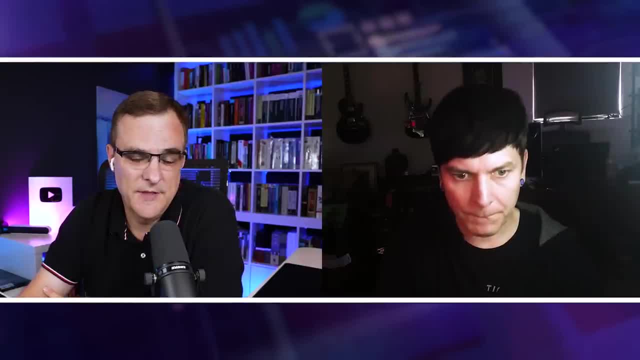 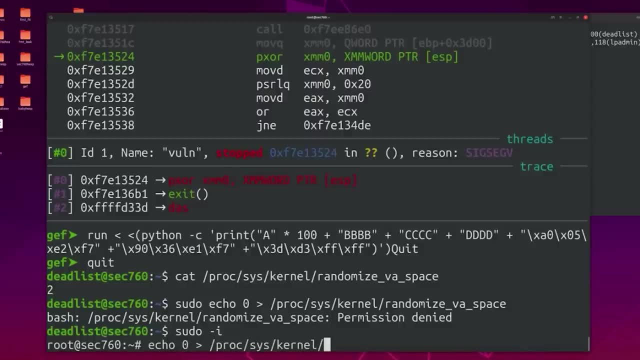 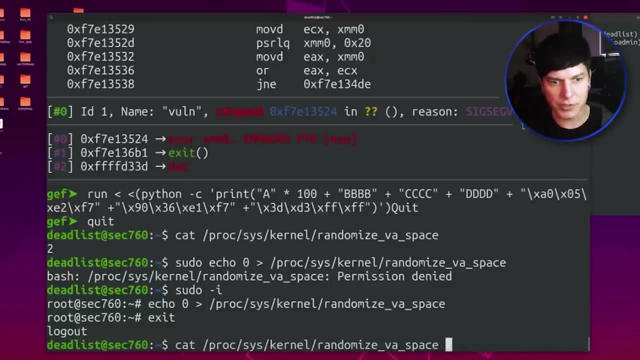 want to see. stephens got so much knowledge and I mean this is just the beginning, so let us know the kind of stuff that you want to see. provision that I agree to. the minus I echo: zero into proc sys kernel. that's the crazy thing is you can turn off aslr so easily on a linux box. on windows you can't do that all. 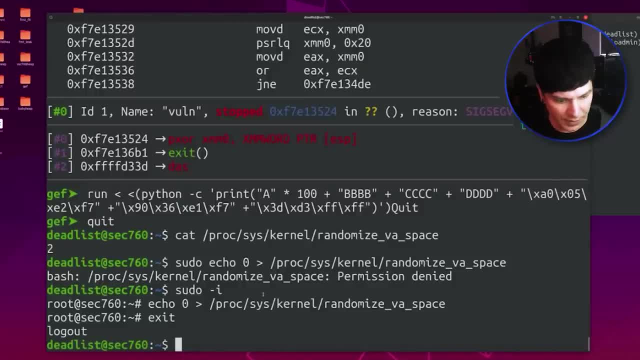 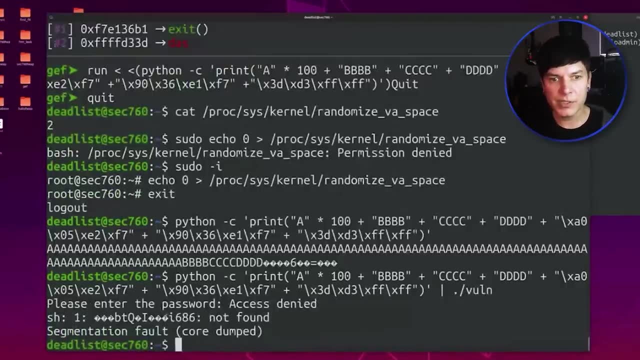 right. so now let's try to run the exploit again. I don't think it's going to be happy, all right. so here's something interesting: we try to run this outside of the debugger and notice it's saying: not found, saying that this crazy thing here is not found. what's happening is it's actually working, so system is actually. 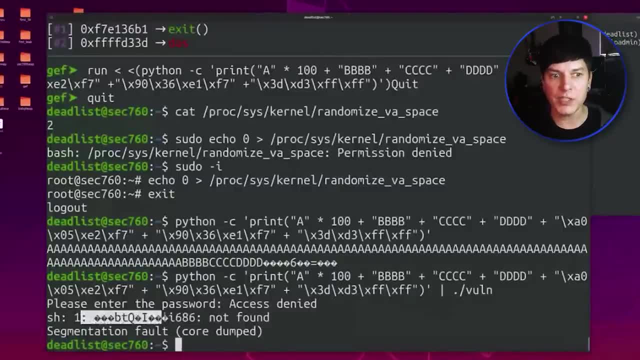 trying to execute our command and that's why a shell is printing out this crazy stuff. but the memory layout outside the debugger is different than inside the debugger, so I'm going to try one last thing to see if I can get this to work. export: I'm going to create an environment variable. no, 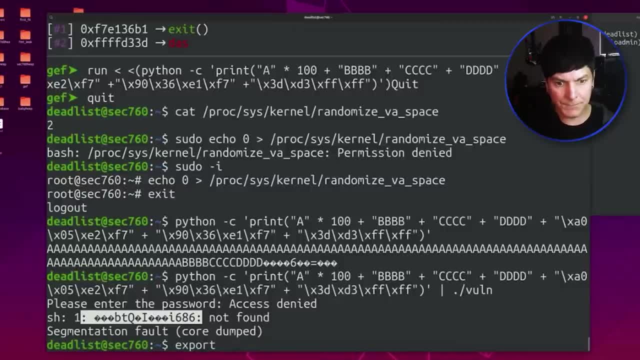 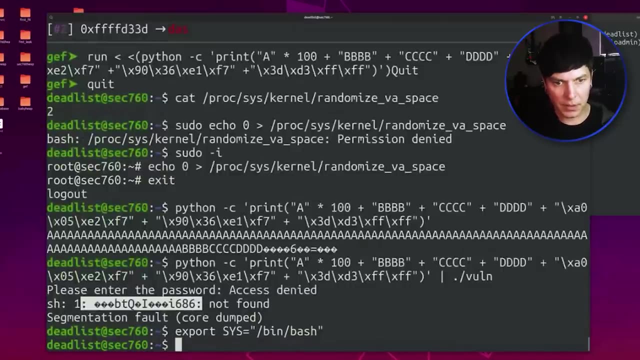 one can see if we can find it. but let's see export and then we're going to call it sys equals, that's my environment variable, and I want it to simply say bin bash. and if I can find that environment variable in memory, then it will execute that. let me see if I can find it here. so that's the problem now is I need to find. 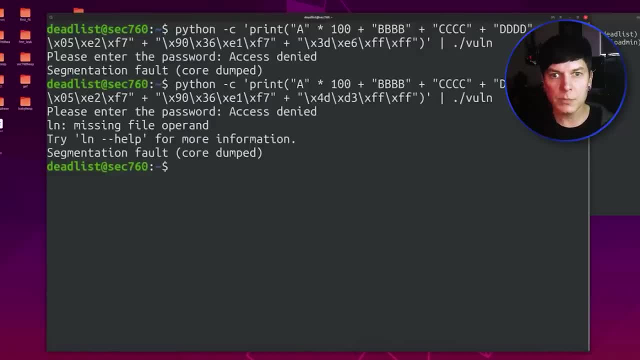 that environment variable, which can be really, really tricky. I'm going to look around a little bit so see how um ln missing file operand. we're getting weird things getting sent to us. that's because we're sneaking around in memory. I'm typing different addresses trying to find the string. 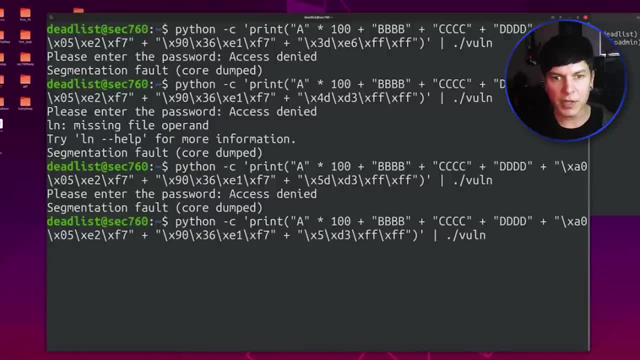 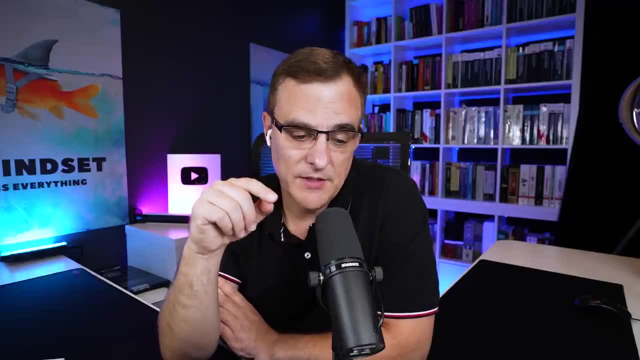 bin bash. so sometimes we can't find it. so I'm going to try to find it. and I'm going to find it because we are passing a string, the system, that it doesn't understand. it's like: what is that so for everyone watching? Stephen and I've spent quite a bit of time now trying to manually find. 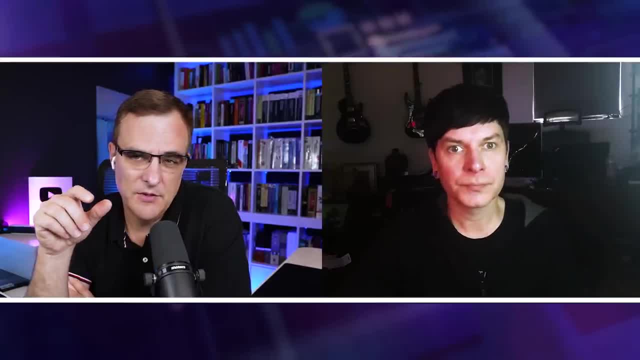 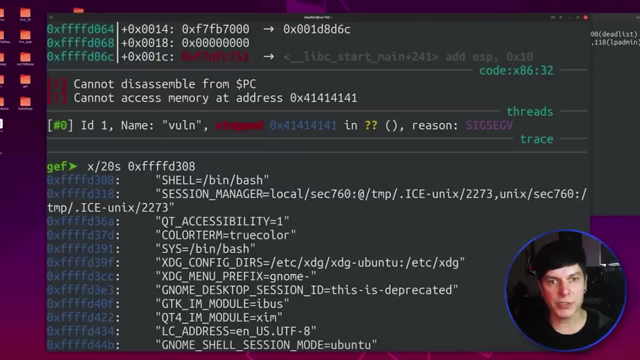 the part of memory. so, Stephen, you can explain it better than I, but you're missing a piece of software that would allow you to find it. and then, when we try to run bash, it wasn't allowing us to do it right. yeah for sure. unfortunately, there's this little program I wrote. it doesn't do anything. 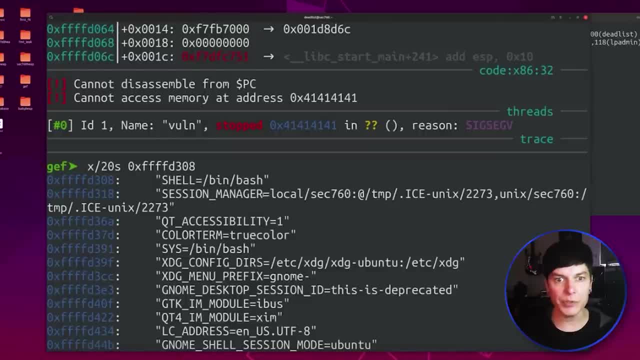 fancy, but it basically, if you create an environment variable, it will tell you the address as to where that environment variable will be located and it will tell you the address as to where that environment variable will be located. and it will tell you the address as to where that environment variable will be located. 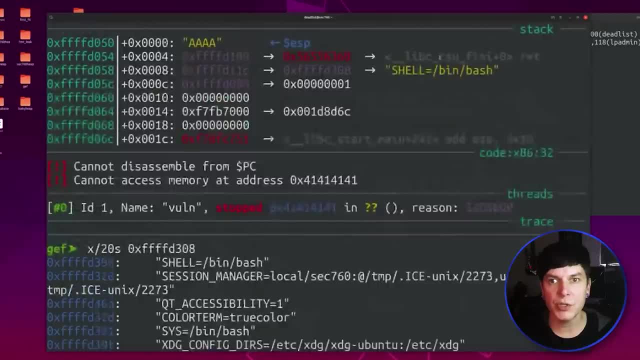 so the first thing we saw was, when the process crashes, we saw this shell equals bin bash. that was, for some reason, there mapped into the environment. so when I ran it in the debugger, as you saw, we got a shell and it worked. it just didn't follow the fork, but we got a shell. 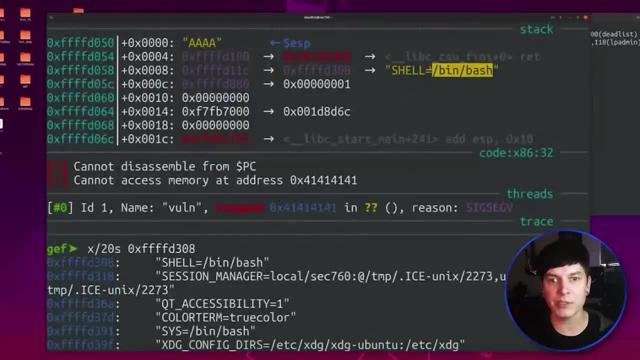 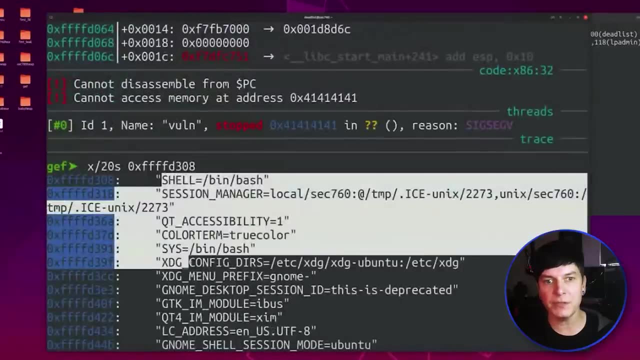 perfect, awesome. wanted to get it working outside the debugger real quick. so I was like maybe I can find this slash bin, slash bash outside the debugger. so we started looking at these environment variables all around here and by messing around with the memory, I was able to find the address as to where that environment variable was located. 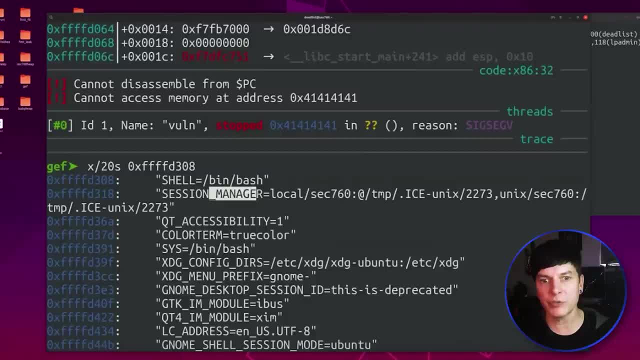 we were able to find out exactly where we were. we printed out true color, we printed out session manager and we should have been right here and we were able to get to some stuff behind that address, but for whatever reason, it wasn't actually mapping that specific shell environment variable. 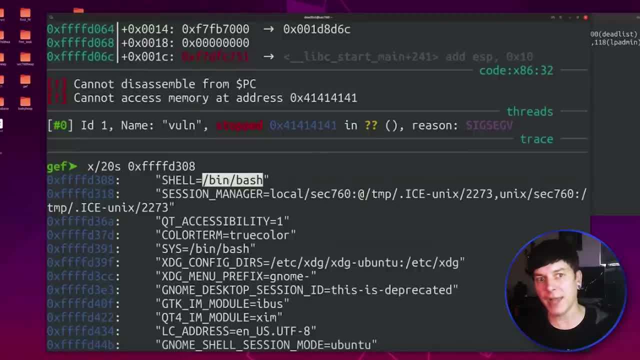 into memory at that spot, even though we found the right address and we don't know if that's maybe a protection or for some other reason that's not there. to get around this, you typically can simply create an environment variable yourself and then find out where that environment variable is. 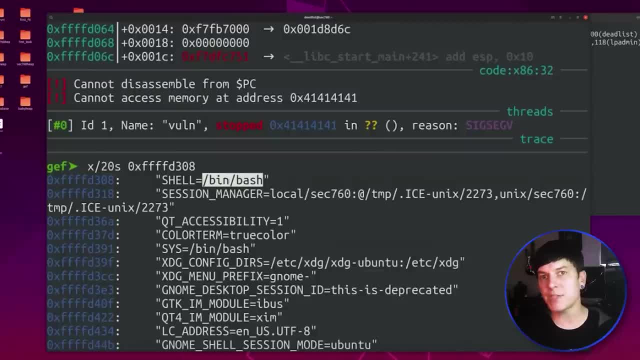 and you can find the address of that variable and pass it as an argument. and this was just one of the techniques that we were looking at, called return to libc, which you overwrite the return pointer with the address of the function. that's loaded into memory and you can pass any argument you want. 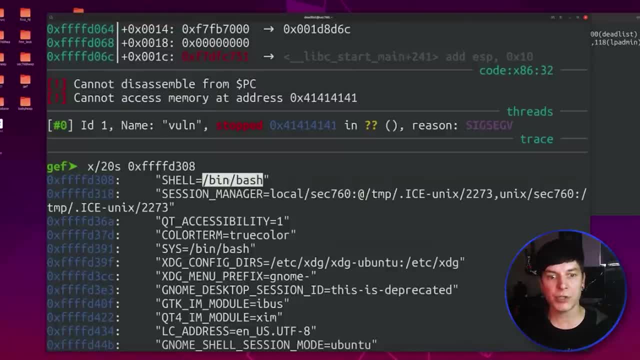 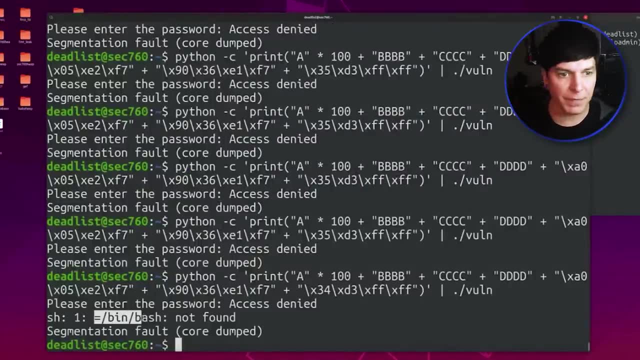 to that function and you get around data execution prevention because the code you're executing is really in the code segment. we're searching through memory here. we just couldn't help ourselves. but to look around a bit more, we were able to find the equals bin bash environment variable and for. 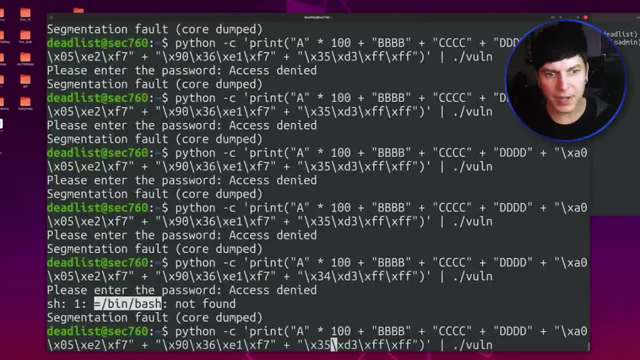 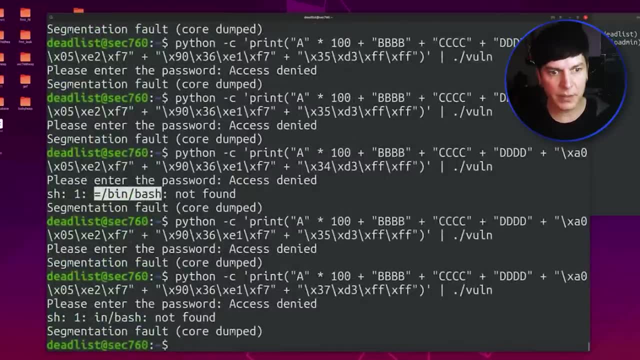 whatever reason we were able to find the equals bin bash environment variable and for whatever reason, when we go forward one more byte to three five, which should actually be slash bin bash, it's not popping a shell. we go forward a couple more bytes, like three, seven, you can see in bash. but 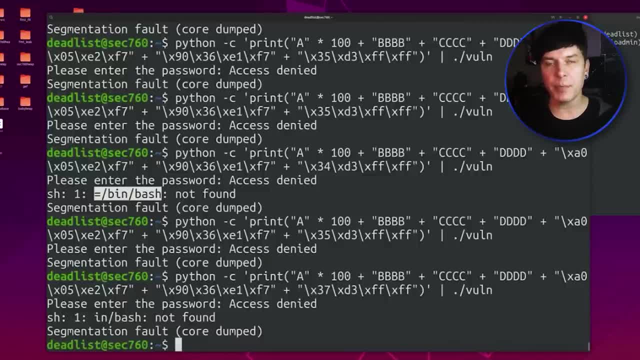 for whatever reason, it's not popping one and it probably has to do with, like, their permissions not being set properly or so the protection might be running on this box. that i'm not compensating for, but we actually had it working perfectly right here and the debugger it worked outside.